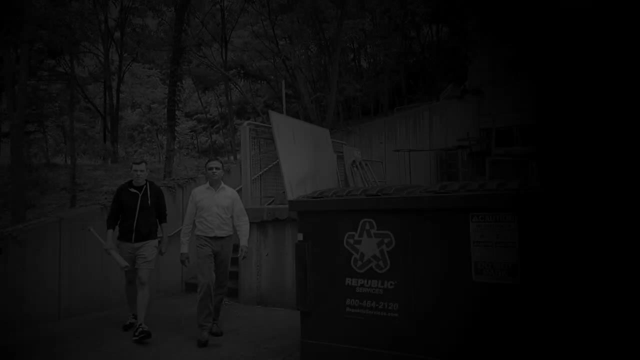 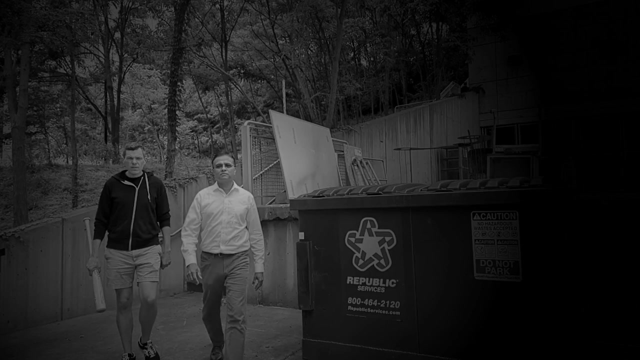 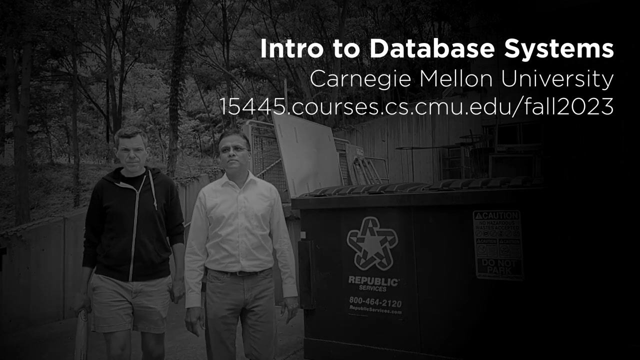 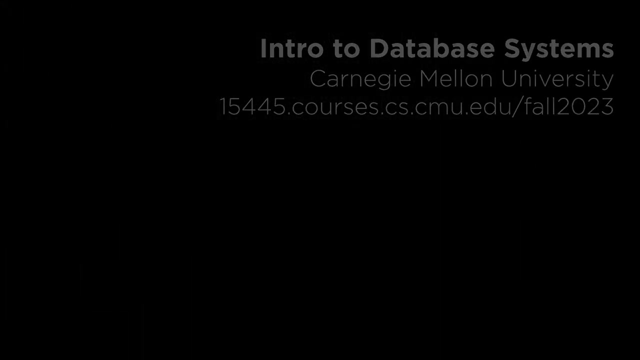 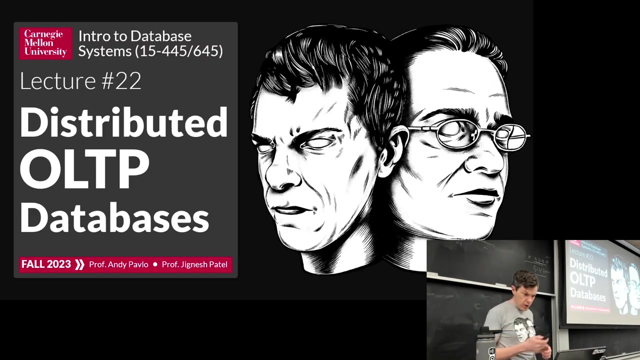 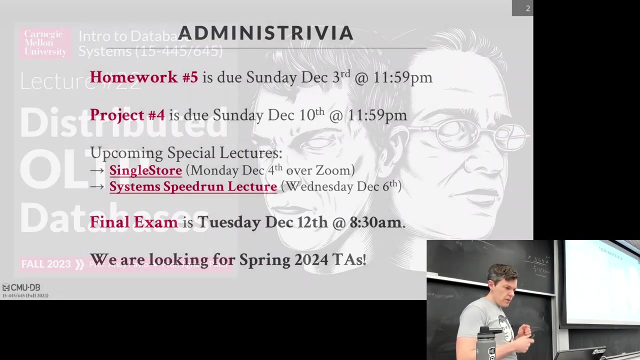 DTGPL is not here. He just got sick. I took him to the free clinic this morning so hopefully he'll be back here feeling better on Wednesday. For you guys in the class, as again Homework 5 is due on the Sunday, coming up on the 3rd. 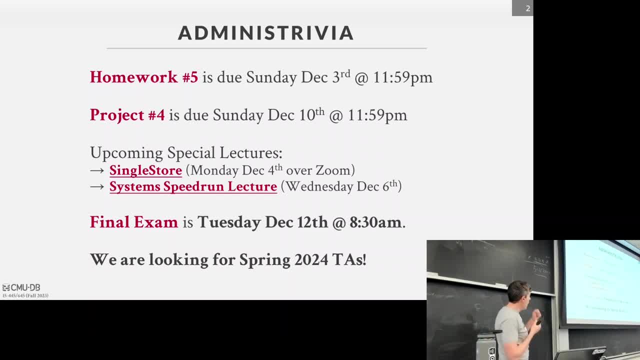 Part 4 is doing the following week, on the 10th, also midnight Next Monday in class- sorry, next Monday not in class- over Zoom we'll have a guest speaker from Single Store talk about their distributed database system And again it'll cover a lot of the core ideas we've been talking about the entire semester. 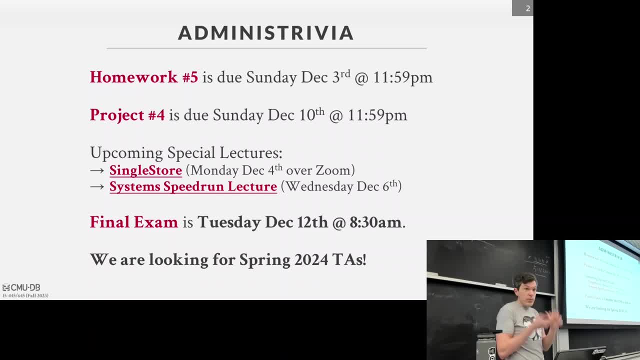 And then you realize, oh, Andy's not crazy and just made a s**t up. This is how people really build systems. And then, as I posted on Piazza yesterday, please go vote. We'll do a speed run on the last day of class. 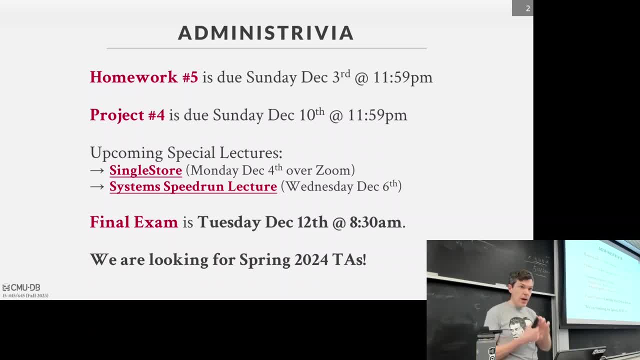 We'll start off with a review for the final exam And then we'll just plow through as many systems as you guys want to learn about And again, instead of having a giant drop-down of 900 different databases- because nobody would click that- just copy and paste URLs in. 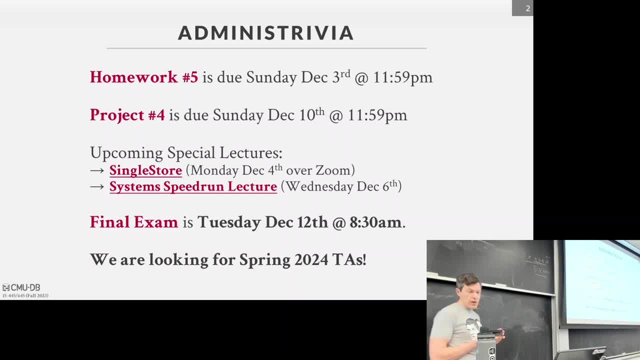 And that way I can sort by uniqueness. right, Just do a group buy. Okay, Again, there's a post on Piazza that takes you to the Google form And then vote as many times as you want, I don't care. 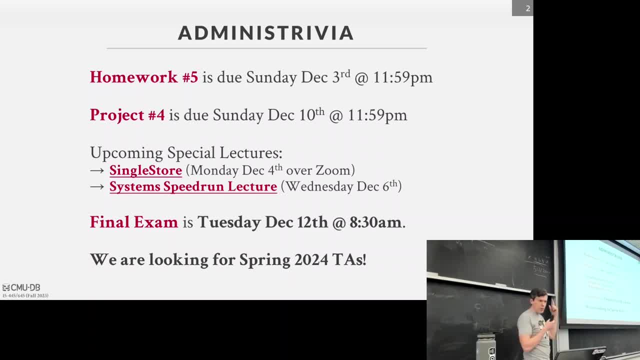 The- I think the number one vote this morning was Redis. It's an interesting system. All right, final exam will be Tuesday, December 12th, somewhere. We'll announce it. That'll be 8.30 in the morning, because it's early and that sucks. 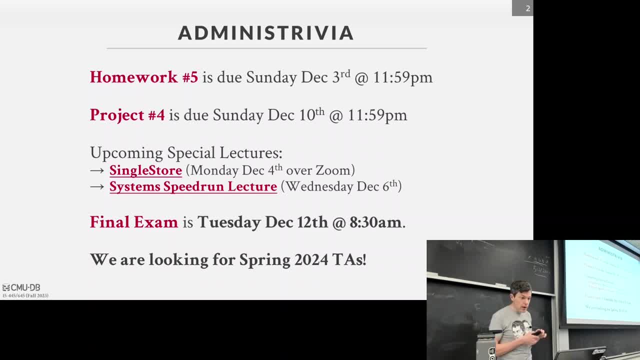 We'll do like coffee, donuts and cigarettes for everyone in the morning And then Jake Nash- He's teaching this class by himself in the fall. So if you want more databases, I want to go even deeper into Bust Hub. 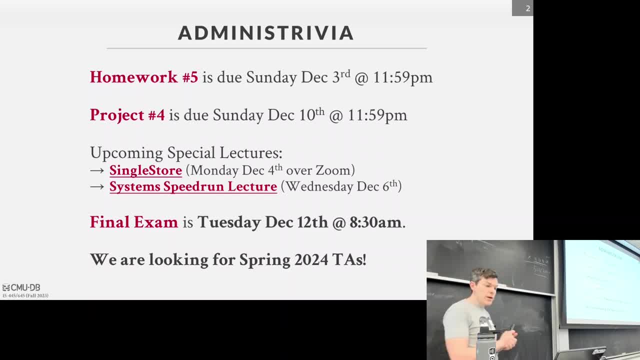 Please sign up for to be a TA. Okay, And we'll post on Piazza how to make that happen. All right, There's a lot here. Any questions? We're almost done for the end of the semester. Okay, All right, let's get through it. 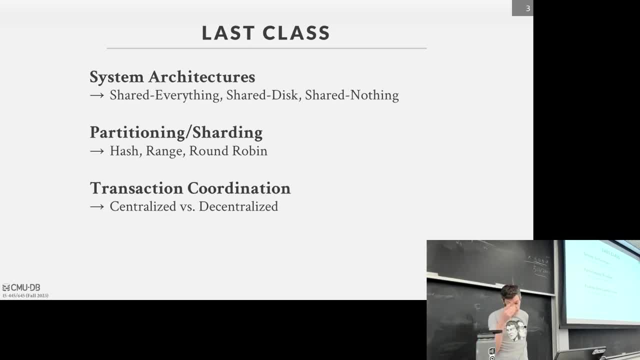 So last class we started off talking about distributed database systems. Again it was a high-level introduction to the key concepts about how people think about and reason And design these database systems. And again, unfortunately there's no distributed data system course at Carnegie Mellon. 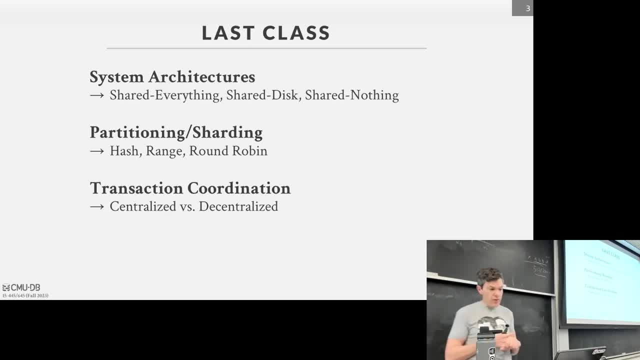 Eventually maybe we'll teach you, But right now it's just myself, So we can't do that. So this last lecture and this week's lecture is really much all you'll be able to get out of distributed databases in sort of low-level detail at Carnegie Mellon. 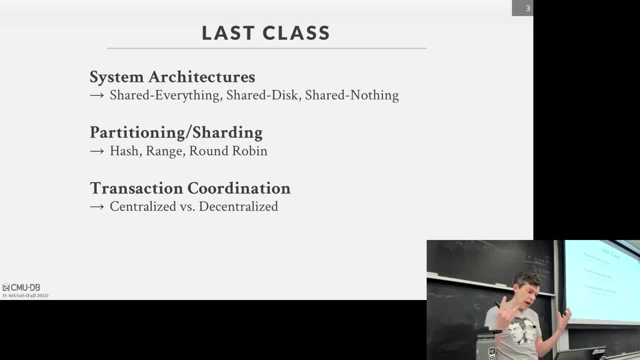 But the again. the idea is to sort of give you a litany of different concepts and ideas and techniques And then that way, when you go out to the real world, you'll see these ideas come up and then you can reason. 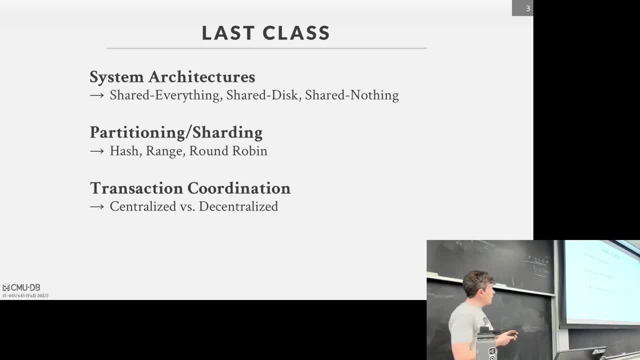 about how people describe their systems. So we started off talking about the different system architectures. We said: shared everything is basically what BustHub is. It's a single-node system where everyone can communicate. The processes or workers can communicate very quickly. And then shared disk and shared nothing are the two sort 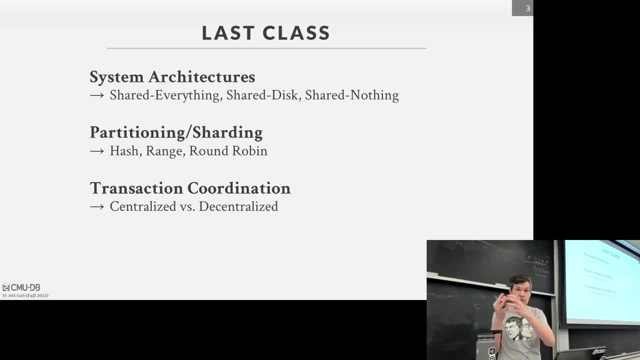 of major distributed database architectures Where shared disk was. there's a single repository or a shared, a single storage device that all the worker nodes can read and write to. Okay, And then the shared nothing is where each worker node, each node in the system, has some portion of the database. 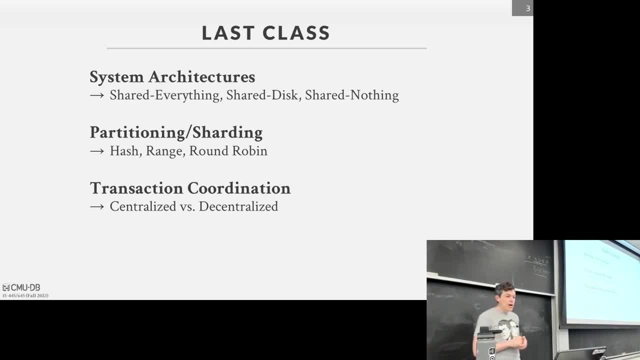 And you have to send messages and pass data between the nodes directly. Then we talked about how to do partitioning or sharding: simple range partitioning, hash partitioning- again splitting the database up into disjoint subsets and distributing them across different nodes. 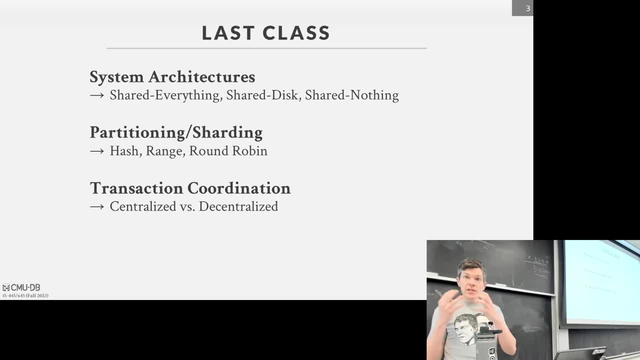 And then we talked about how to do transaction coordination at a high level, Like is there a centralized coordinator that's in charge of taking all the queries, figuring out what locks or what data they're going to touch And communicating to the different nodes? 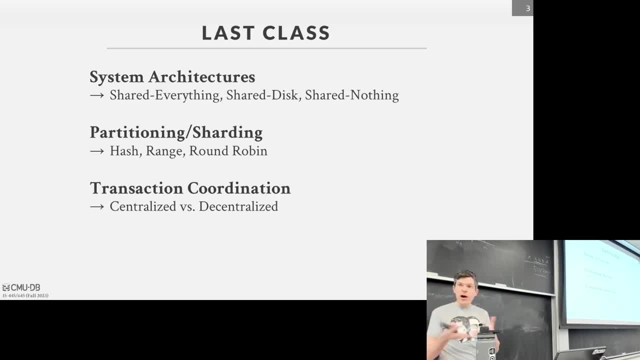 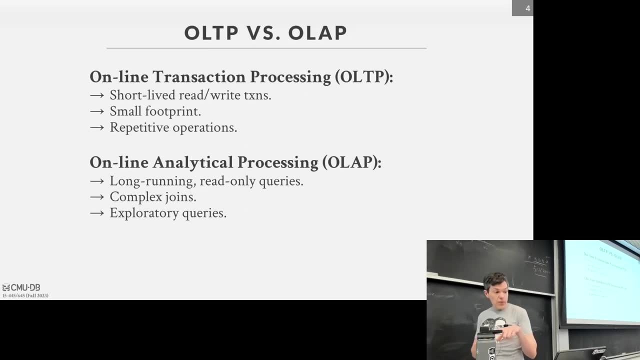 Or is it decentralized, meaning the nodes are free to decide on their own how they're going to commit and order transactions? All right, So today's class we're going to focus on transaction processing. Wednesday's class will be about analytical processing or decision support systems. 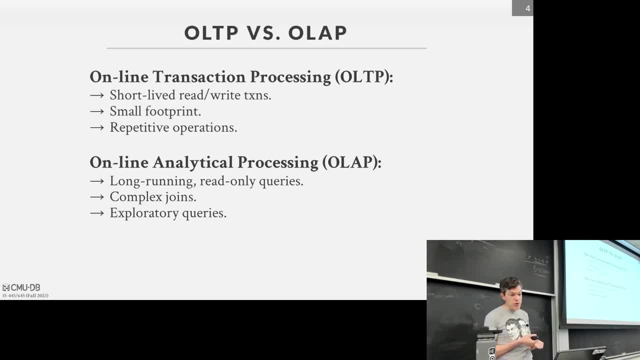 And we've talked about this many times. I just want to bring up the distinction between the two workloads today again, because then that'll help us understand what are the different workloads that we're going to use. Okay, So what are the different design, tradeoffs or things we're going to care? 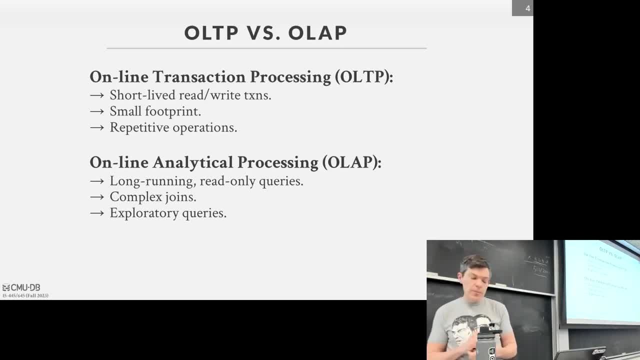 about in one sort of category of a system versus another. You can think of it like something like Postgres is meant to be like a general purpose database system. It is a row store and it can use transactions. Primarily people use it for OTP, but there are some aspects. 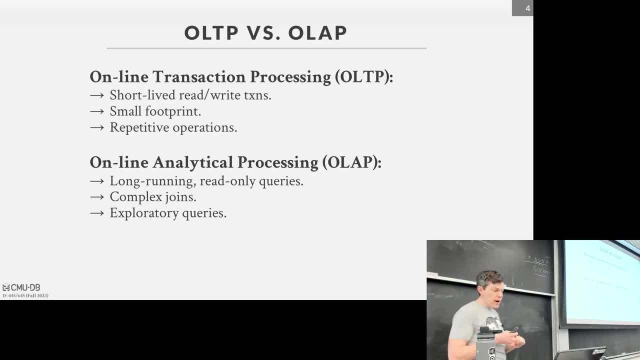 of it that you would see in an OLAP system- Right, But there's certain things that Postgres does that you wouldn't want to use in like a Snowflake system, because they're not worried about running transactions. So the two rough categories. 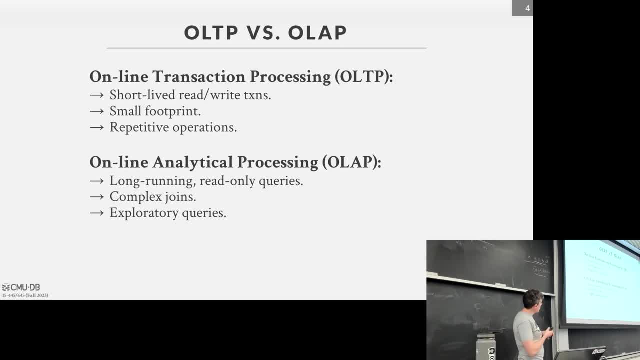 It can be sort of broken up between these characteristics. So for OLTP workloads, these transactions are going to be short-lived and they're going to be a combination of read-write queries. Short-lived means like less than 100 milliseconds. Even that's a long time. 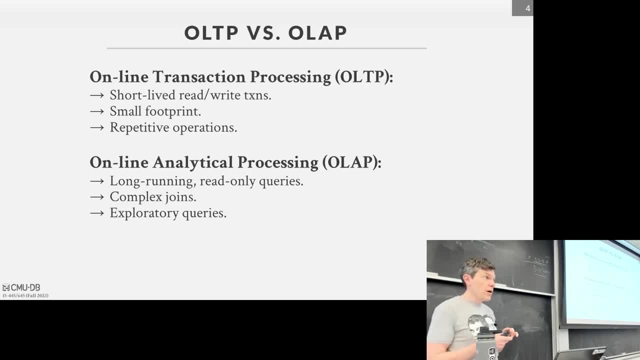 50 milliseconds is considered the max you want to have for a transaction. Anything longer than that is considered a longer run transaction And that number comes from that. 50 milliseconds is like the conventional wisdom in like internet advertising, Like when you go visit a website, assuming you don't have an ad blocker turned on. 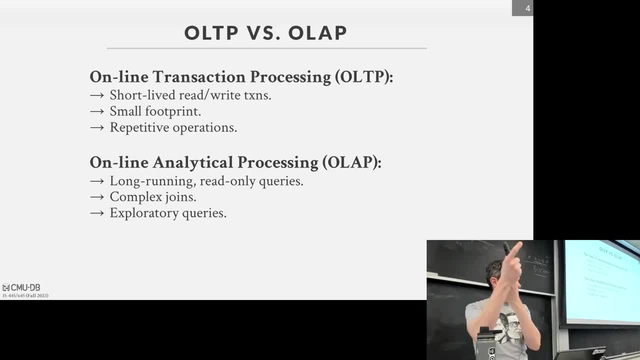 If you don't, please do that. When you go visit a website there's an ad blocker turned on. Sorry, If you go visit a website, the ad serving company has an auction that it sends out information to all the people that want to potentially put out ads to do like a bid on it. 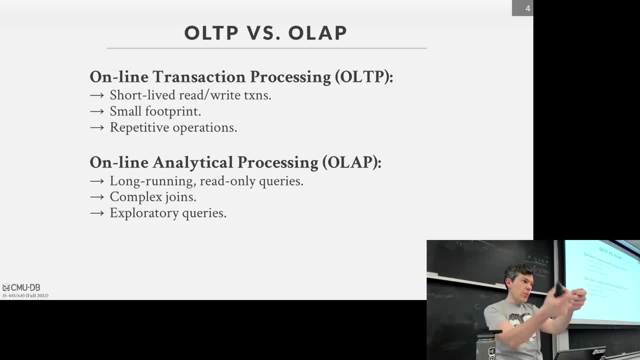 And they say: here's the information about this person visiting the website And you have to give back a response roughly in 50 milliseconds, Right? So roughly that's where this number comes from. It might be down to 30 milliseconds nowadays. 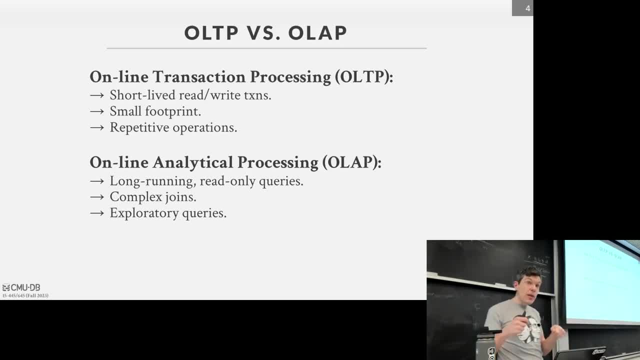 If you're doing high-frequency trading. those guys are freaks and they want things done fast. They want things less than a millisecond, but the workload basically still looks the same. It's a lot of small gets and sets, And then these operations are also going to be very repetitive. 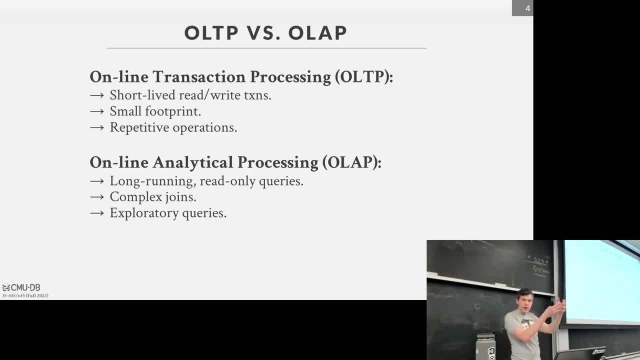 Again. think of like going through a website. You can only do a certain many things on a website. You know you're not sitting at a raw terminal putting in a SQL query, So you're running application code that's going to be running the same queries over and over again. 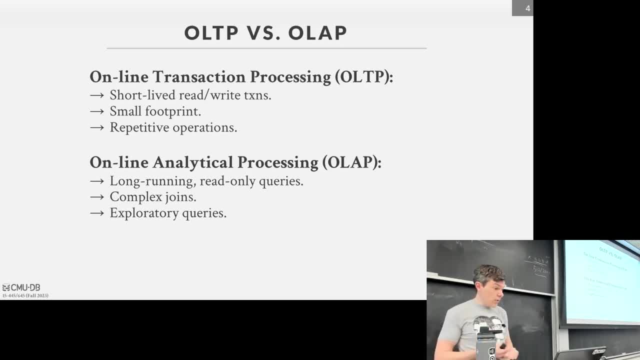 And there's certain optimizations you can do if you know you're going to be running the same queries over and over again In OLAP. again, we'll focus more on this workload on Wednesday, but these will be long-running queries, Typically read-only. 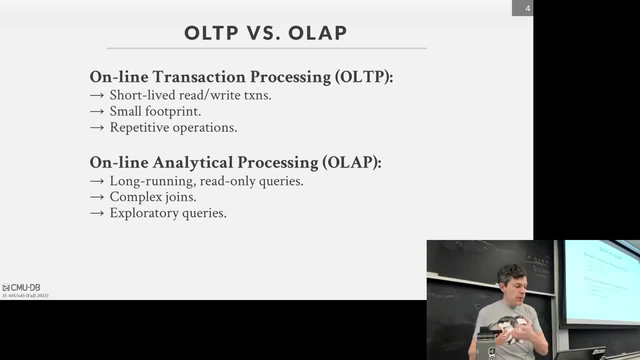 Doing a lot of joins and oftentimes they'll be sort of one-off ad-hoc queries, Because someone's sitting in a dashboard clicking a bunch of buttons to form a query. They click, go to generate the visualization and it may be the first time. 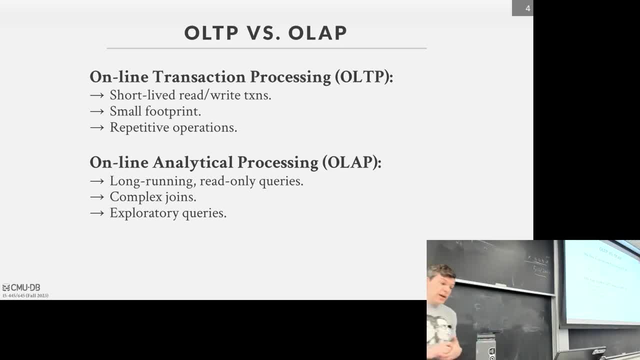 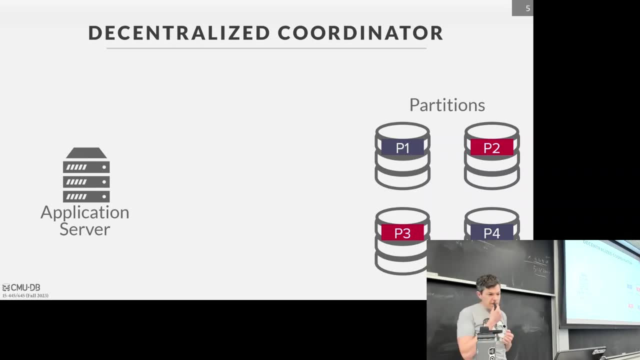 that the database system has ever seen that query And it may never see it again. So that limits what sort of optimizations you can do. All right, so this is the setup that we sort of care about today. right, We have some application server that wants to run a transaction that's going to touch. 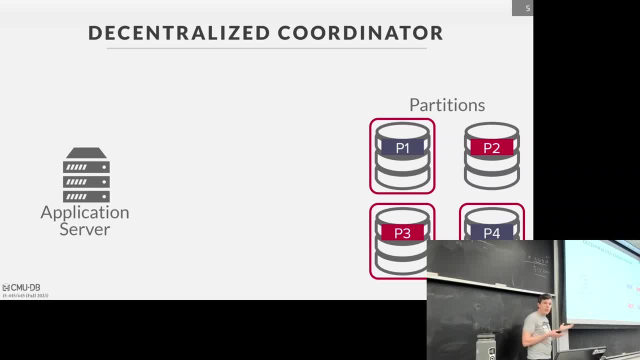 data at these three partitions. I'm not saying whether it's shared disk or shared nothing. For our purposes right now it doesn't matter. So somehow we've elected this one first partition here to be the primary node. So the begin request for the transaction goes to this node. 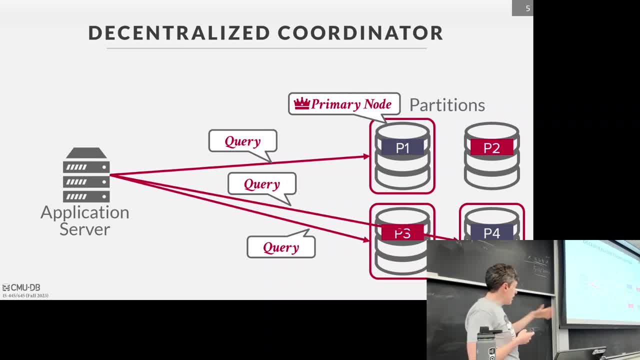 And let's say there's no centralized coordinator and the application is allowed to send queries directly to the various nodes And then, when it comes time to commit, it goes to the primary node and says, hey, can I commit? And the primary node is responsible for figuring out amongst the 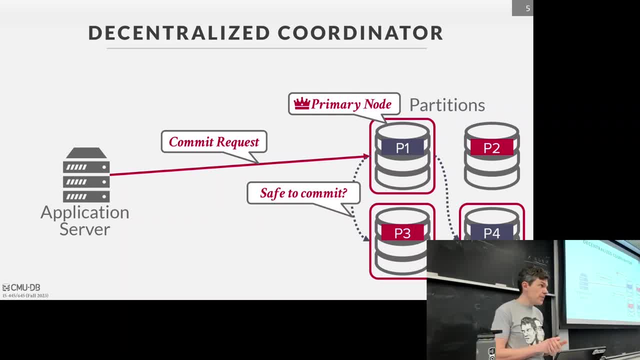 nodes that participate in the transaction whether this thing is allowed to commit, All right. so our focus really today is this sort of safe commit step and how to get everyone to agree that, yes, this transaction is safe to commit. And then, if they all say yes, it's going to commit, that we commit it, all right. 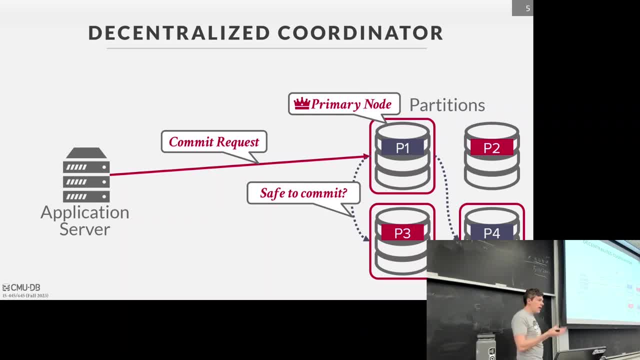 And all the stuff we talked about before, like two-phase locking or multi-version query control or OCC, all of that is still happening here. right, There's still. That's still the Yeah, The mechanism that's going to use to determine is this thing allowed to commit. 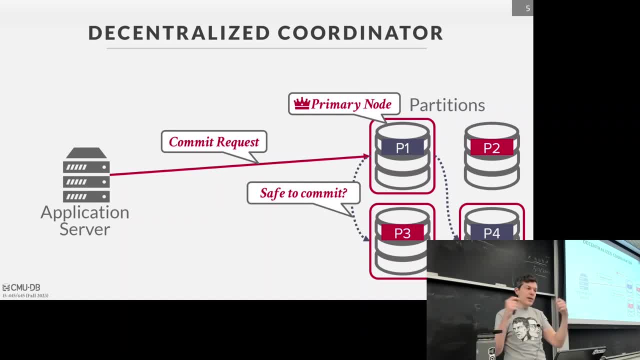 on each individual node, and then there's a higher level process above that. that's trying to get everyone to agree that it's now time to commit this transaction. So that's the big picture of what we're trying to do today. And so again, even though my last example, I showed the application going directly- 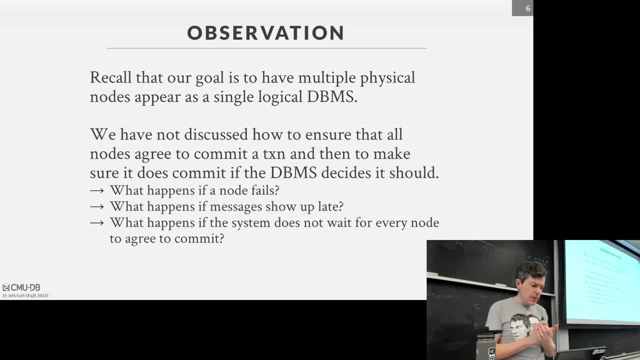 to different partitions. ignore that for now, but the big picture of what we're trying to achieve today is that, and as you would want in any distributed data system, is that you would have a. You want to have a single logical view against a single database system, even though, underneath, 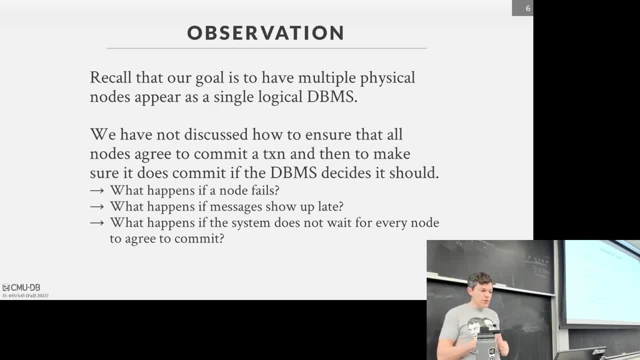 the covers. it's comprised by multiple physical servers, so multiple physical resources, And so we haven't talked about how, again, we're going to get a transaction or nodes to agree that we commit a transaction And then, if we decide that it is going to commit, how do we make sure that it does commit? 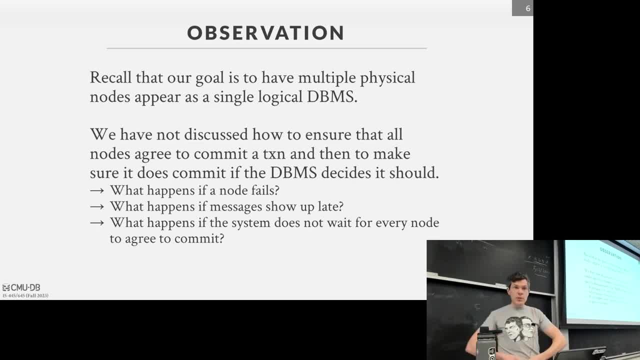 And if there's a crash, if there's a failure, that when the system comes back up, that if we set, We told the outside world that a transaction committed, We have to, We have to make that guarantee. That's the D in asset, the durability guarantee. 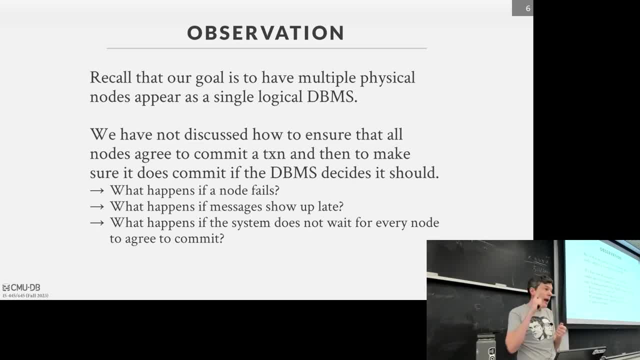 But again, if the whole thing goes down and come back up, then that's one thing, But what happens if one node goes down, which will happen? How do we deal with that? Well, what happens if we send a message, commit a transaction and then the message disappears? 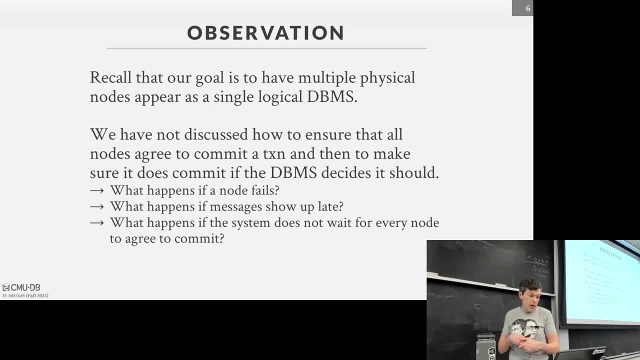 somehow Because someone tripped over the cable, there's a weird hiccup in the network or something, and then now our message to commit this transaction shows up late. What do we do? What does the node do in that setting? And then what happens if every node 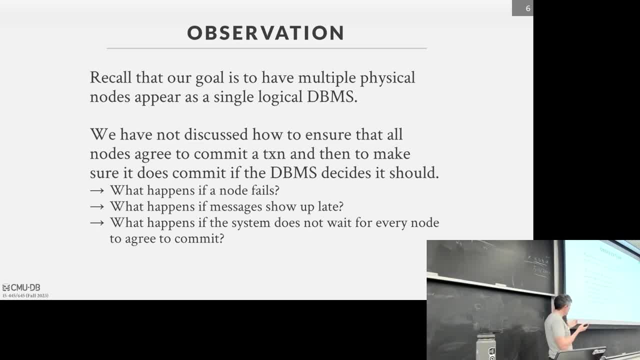 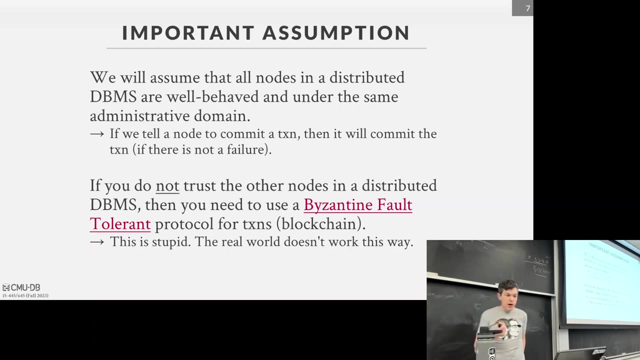 Sorry, What happens if the system? We don't want to wait for everyone to agree to commit, but we still want to commit in some cases. We don't want to block everything in case one node goes down right. So one very, very important assumption that we're going to make in today's discussion: 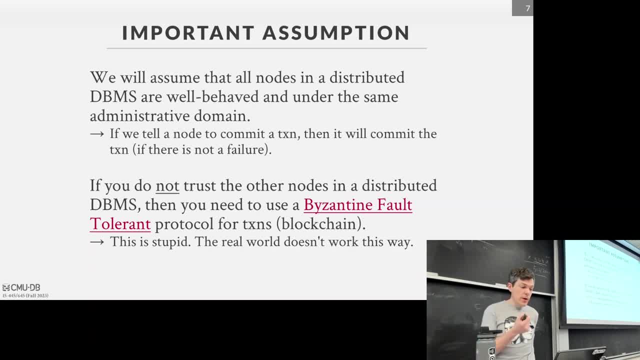 is that we're going to assume that all the nodes in our distributed database system are going to be well-behaved and under the same administrative domain, And what I mean by that is these are nodes that, if you're the database system operator, these are nodes you control, that you own or you're renting or whatever, and it's running. 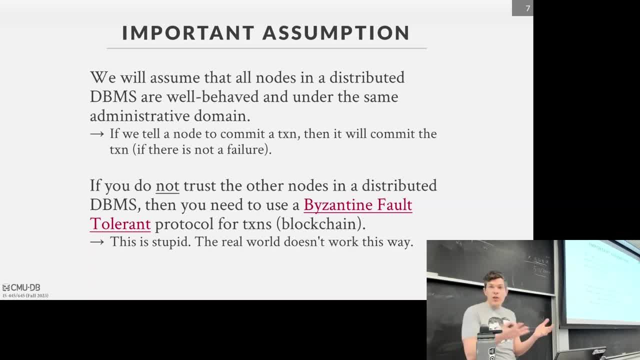 software that it's expected to run as part of the database server, right? So that just means that we're not in this weird untrusted world where there's some nodes in our distributed database that we don't control and we're renting, Or that people are running altruistically or something, and it's not going to be the. 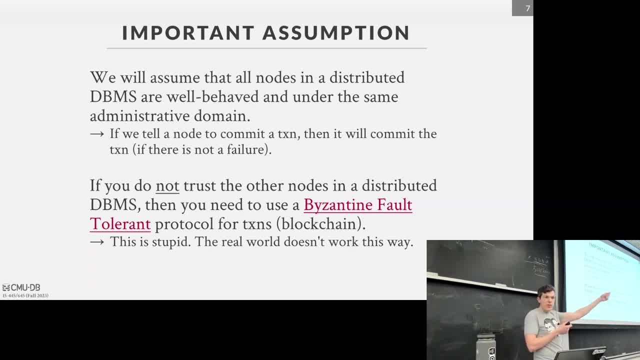 case that we go commit a transaction and one node's going to be nefarious and start trying to screw with us and say no, no, no, we're not going to commit that. Or if everyone agrees that it commits, this other node isn't going to come back later. 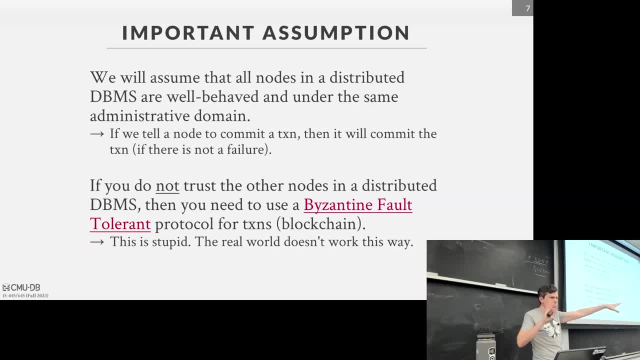 on and say, hey look, I lied, we didn't commit that transaction- and start trying to change the state of things, right? So that kind of tolerance, or that property, is called Byzantine fault tolerance, and that's what you get if you get a blockchain right. 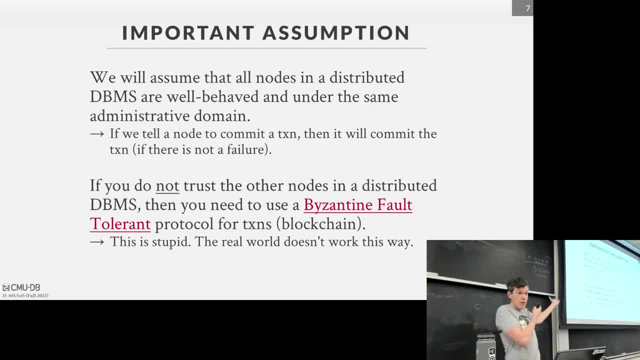 Blockchain basically is just a database, a distributed ledger, distributed write-ahead log And in that world- because something like on Bitcoin, where it's a bunch of people running these peer-to-peer networks where you don't control, there's no single authority controlling. 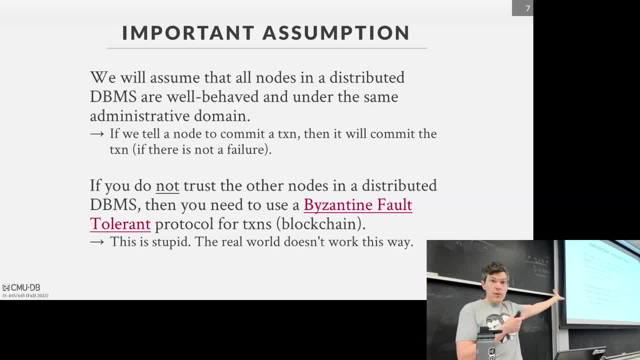 all the different nodes. you need a BFT protocol. We don't care about that shit, right? That's a bunch of overhead that we don't have to deal with And, to be honest, if you want to run transactions at scale, you want to run transactions at scale. 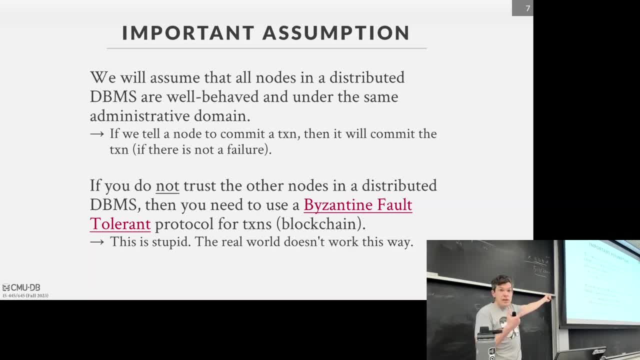 you wouldn't want to use a blockchain anyway, because they measure their latencies in like seconds. Right? If you go to a website and make an order on Amazon and it takes like 20 seconds to commit that transaction, you're going to give up, right? So nobody runs a real database system doing transactions on a blockchain. This is stupid. The real world doesn't work this way. We can ignore that entirely. OK, So now that doesn't mean a node won't crash, disappear. come back and try to say hey. 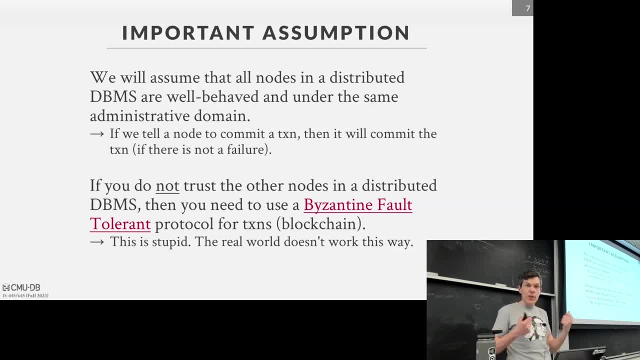 guys, I missed What's going on. I missed all the updates And then you've got to go ahead and update. But again, that's just a hardware failure And we will have mechanisms to deal with that. And we're still not worried about whether the node is nefarious or not. 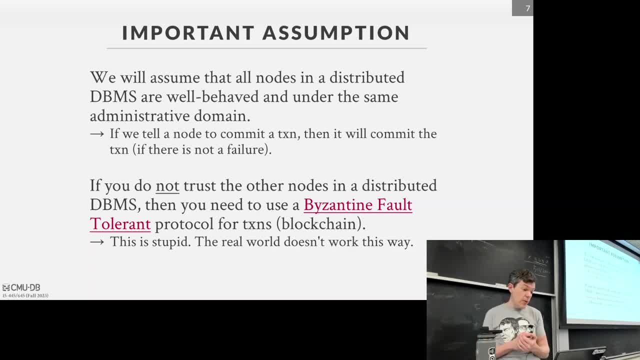 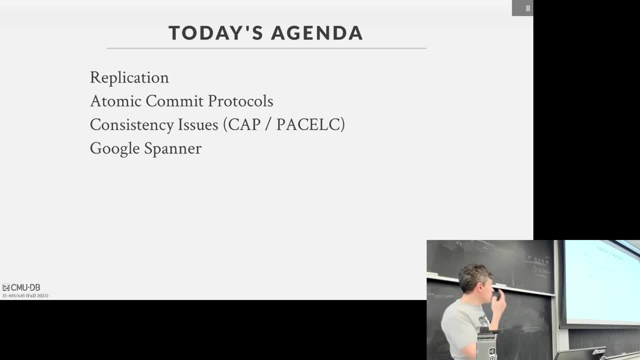 OK. So it makes our lives a lot easier if we don't worry about visiting fault tolerance, All right. So today's lecture is really me again attempting to try to condense a year's worth of material in distributed databases, And I'm going to go ahead and give you a little bit of a summary of what I'm going to do. 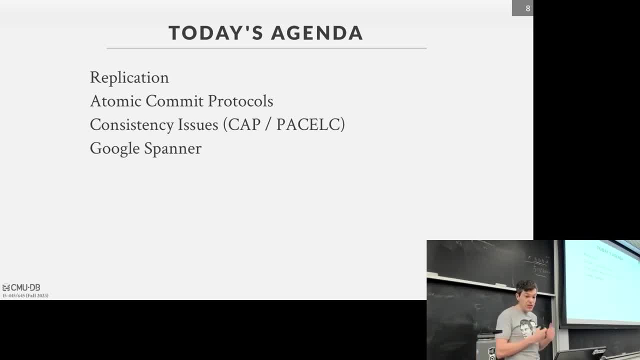 So we're going to go ahead and go ahead and go through some of the most common things we've done in distributed databases into one or two lectures, So we can't cover everything into detail. We're going to go through these are the most important things that you need to be aware. 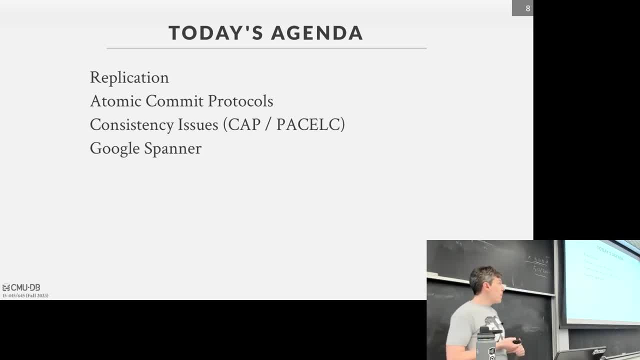 of that exist and the challenges you will face when we have a distributed data system. So we're going to first talk about what replication looks like in this environment. So for most people when they say, oh, my database can't scale, the very first step. 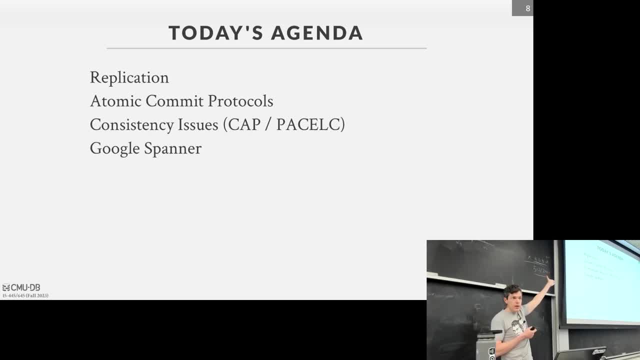 you actually should do is replication. You should probably be doing this anyway for high availability and durability, But you can actually offload some reads to, like the database, to replicas, to, depending on your workload, to alleviate some of the load and start scaling things out. So, even though most people don't need a massive 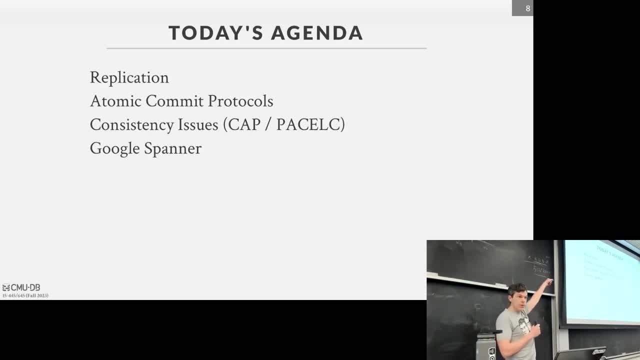 distributed database system like a Spanner. you're gonna need replication almost always, right, if you care about your data. Then we'll talk about atomic commit protocols, two-phase commit, Paxos, RAPT, how to actually get everyone to agree, And again, I realize there's a distributed systems course at CMU that. 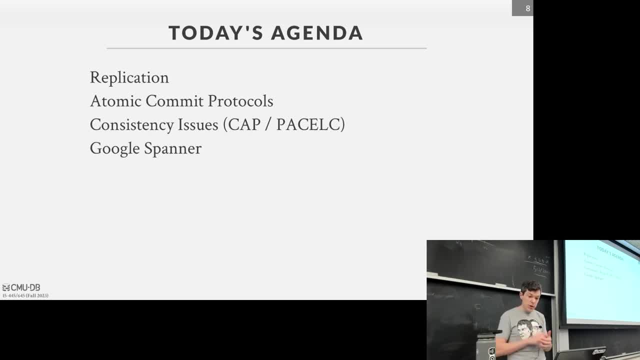 does a better job and spends more time talking about these things. but we just want to describe it in the context of databases, And then we'll talk about consistency issues in the context of the CAT theorem or PESELIC, which is the follow-up to it, again in the context of databases, And, if you have time, we'll. 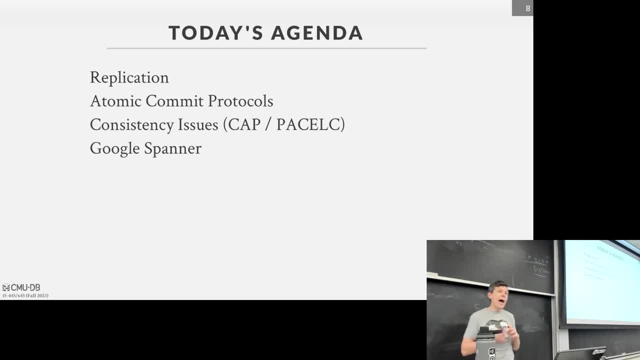 finish up just talking about Spanner real quickly, just because it encapsulates a lot of the ideas we'll talk about today, and I consider this a state-of-the-art system, even though Google put it out, you know, over 10 years. 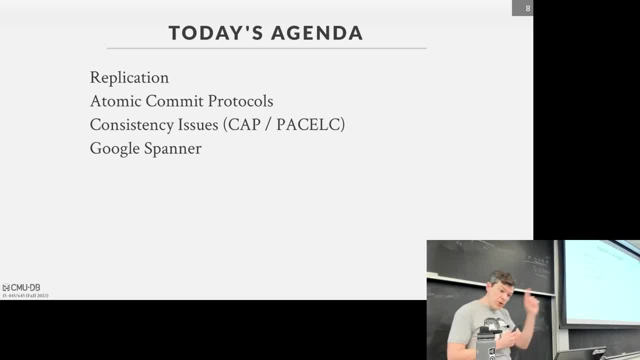 ago. It does a lot of very interesting things, And then you do this one thing that nobody else does, which is you can do if you're Google and have Google money. Anybody take a guess what that is. know what that is if you're familiar with Spanner. Which one Atomic clocks? Yes, we'll get there in a second. So, spoiler alert, Google basically puts satellite hookups, gets the time from satellites, from GPS satellites, and has atomic clocks in every data center. And that doesn't make things magically always in sync, but it reduces the 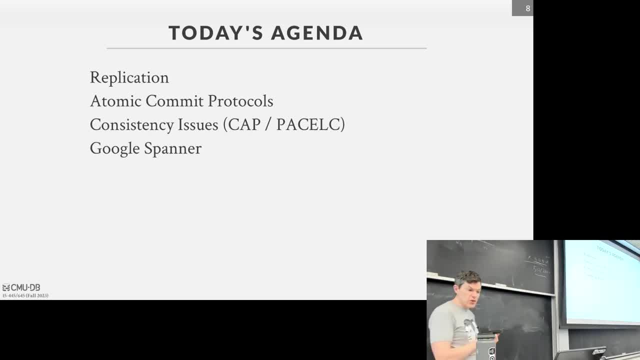 bounds how much time you have to spend waiting for new transactions to show up Again. we'll get there in a second, But they're still gonna do Paxos, they're still gonna do phase commit, they're still gonna do NVC- all this. 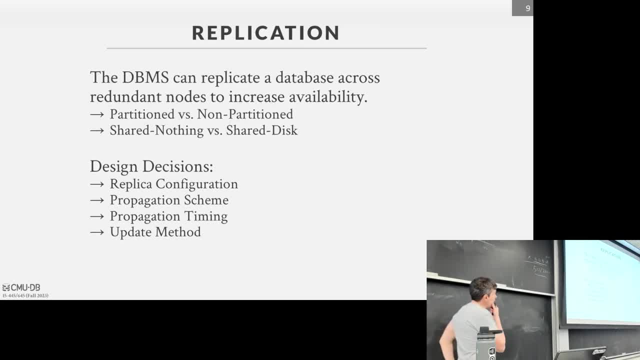 other stuff. Okay, so with replication, the idea is that we want to replicate the database, either a portion of it or all of it, across multiple nodes, And we want to do this to increase availability and, in some cases, scalability. Not always, but 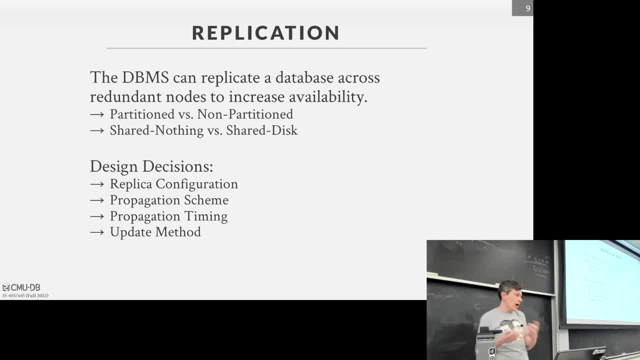 in some cases, yes, And again we want to do this whether it's partition or not. So partition would be: if I split my database up into disjoint sets, I still want to have multiple copies of those disjoint subsets. So again, if one node, 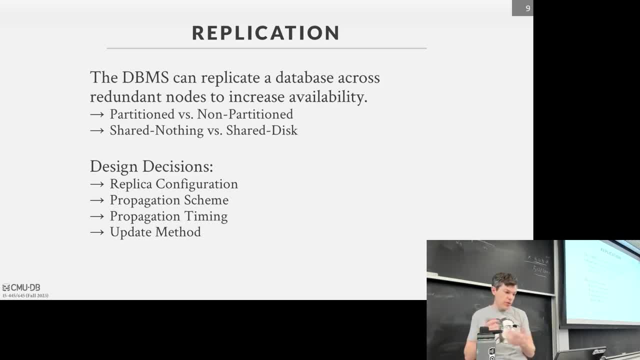 goes down, I've got to have multiple copies of those disjoint subsets. So again, if one node goes down, I can still potentially serve queries. Or if it's not partitioned, which is most database systems, then I want to be able to use the replicas for offloading. 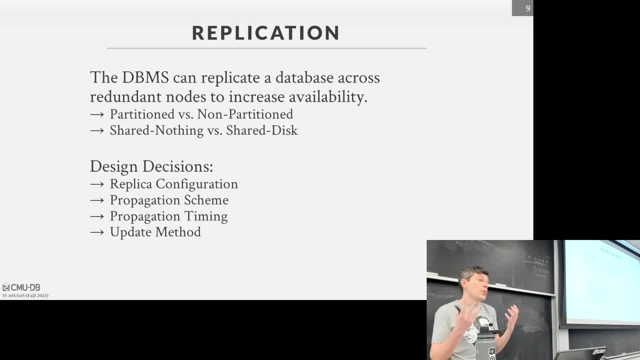 maybe read-only queries. So the idea is again, we want to make multiple copies of data so that if any node goes down, we can still potentially remain online. So there's a bunch of design decisions we have to put in our system if we want to add. 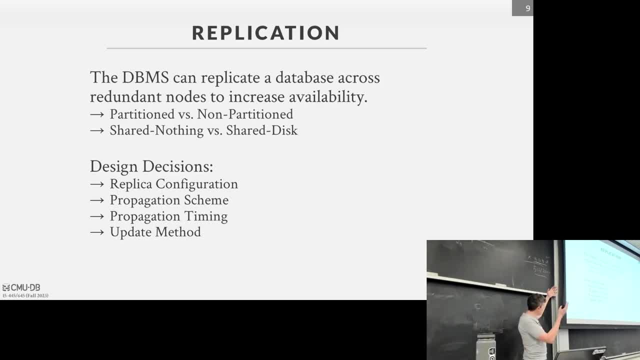 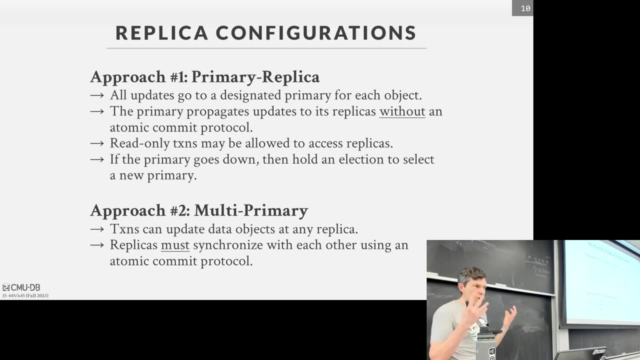 replication. So what the overall configuration of the architecture is going to look like, how we're going to propagate the updates- when should we propagate the updates? and then the method in which we propagate those updates. So at a high level. basically, there's two approaches to do replication. You have what is called 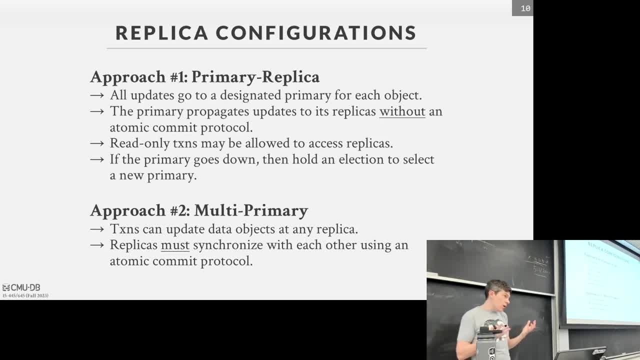 primary replica and multi-primary. So primary replica is the most common one. Sometimes you'll see this as leader-follower. The older terms use master-slave. We obviously don't say that anymore. The problem is a lot of the literature that describes this. 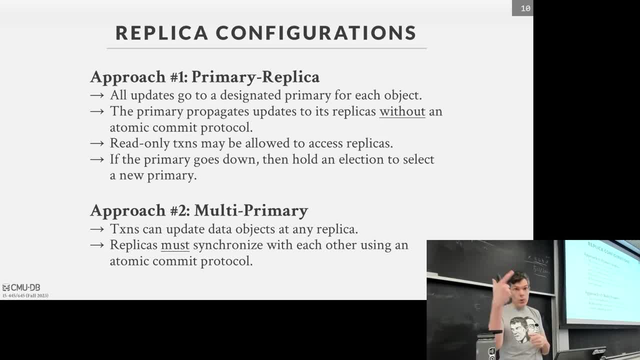 configuration is going to be a bit older, so you have the Google master-slave, but usually the newer stuff will refer to as primary replica. The idea here is that all our updates are going to go to a single node, primary node, in the 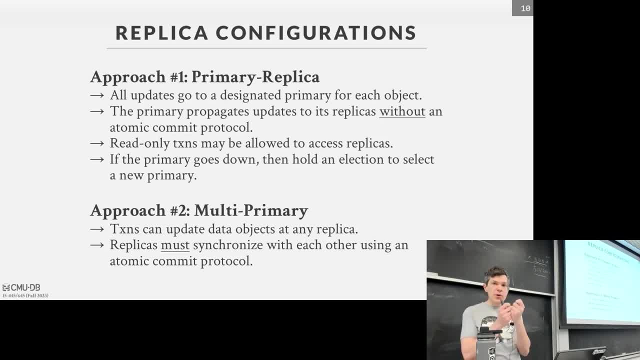 database right And it's going to be that primary's responsibility to then propagate those updates to any replicas- right Leader-follower, primary replica And in some cases, depending on the system how they expose this capability, you'll allow read-only transactions to run queries on those. 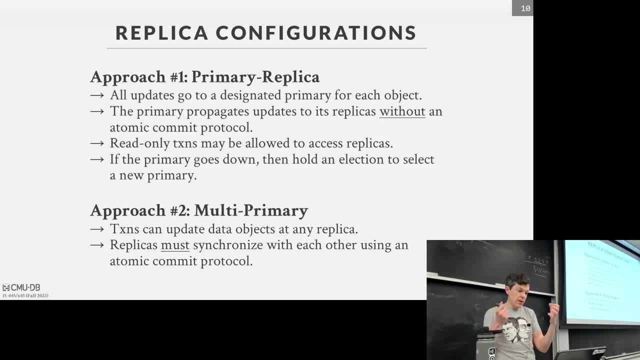 replicas right. And you can do this because if everything's all transactional- meaning if I do a transactional update on the primary, then I propagate that transactional update to the replica and that update is atomic- then any read query will see a consistent view of the 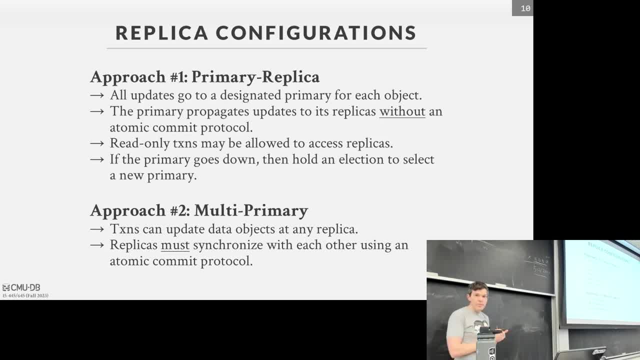 database on the replica. It may not be the most up-to-date version, to be honest, depending on how we propagate the updates, but it'll be at least consistent And of course you can relax that and see. you know, see partial. 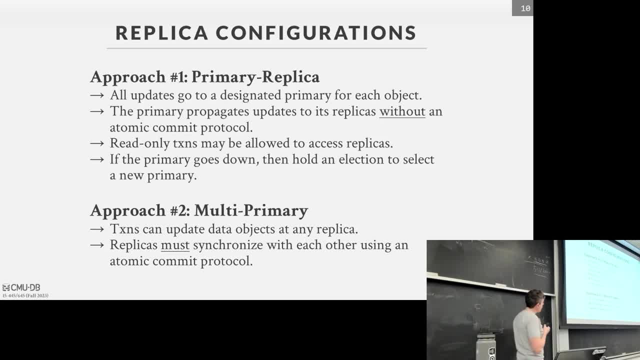 updates if you want. Alright. So then what happens is if thein the event, the primary goes down, we'll hold some kind of election process, which willwill be Paxos or something, and we'll elect aone of the replicas will become a new. 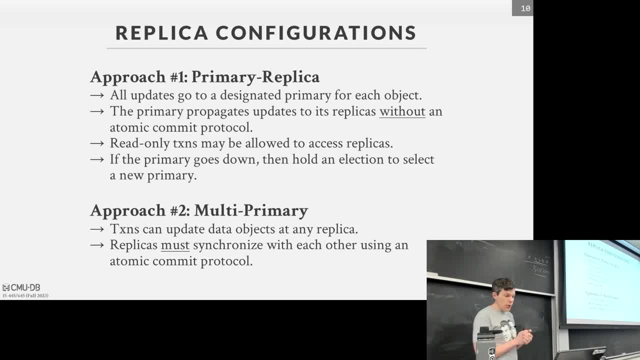 primary and then now all the rights will go to that, to that, to that new primary right, And if the old primary ever comes back up it'll get relegated to the new primary, to the to be a replica again. we'll handle that in a second, all right, so this: 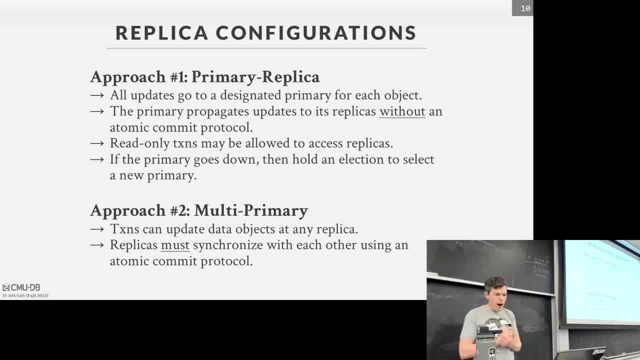 is the top one. here is what most people are going to do: the bottoms, the bottom one, multi primary, sometimes called multi home. this is where the, the replica, every object we replicated in, cross multiple nodes and any transaction can update that object, like a record, a table, whatever- at any possible node and then 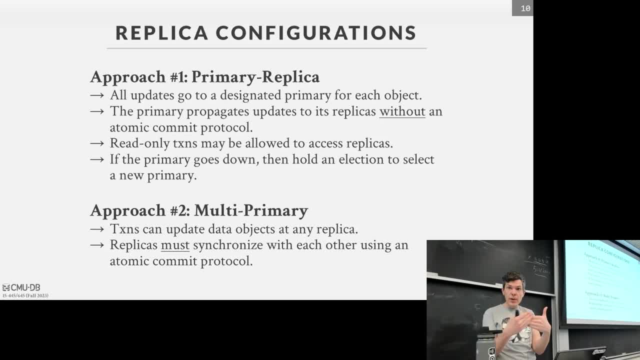 when you go to commit. now the replicas need to synchronize amongst each other because they're all considered leaders or are the primary. they need to need to coordinate with each other to figure out, okay, like who's allowed to commit, you know, who has the most latest version and how to reconcile any changes. all right, 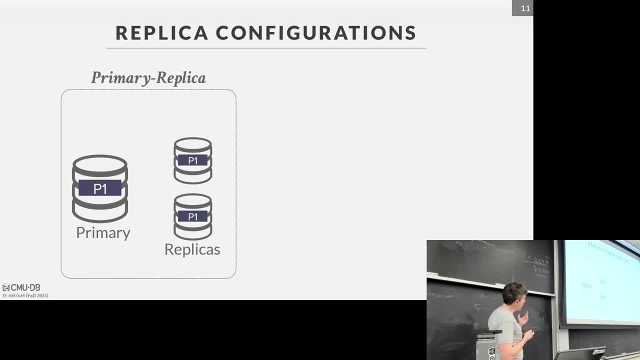 so those are, you know, two visualizations of this right. so again, primary, replica, we have a single primary and then the two replicas. all the read and write queries will go to the primary and then the rights will get propagated to the replicas, and this is typically just sending the write ahead log. 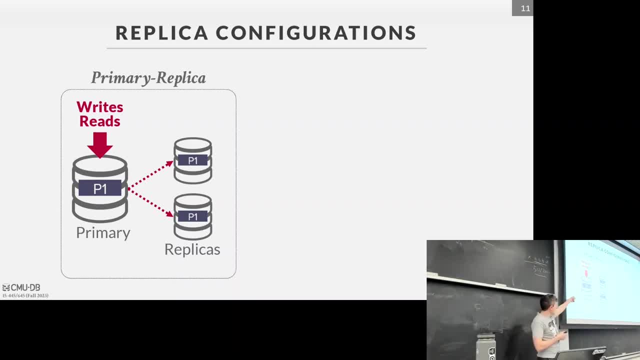 um, that we talked about before, because you're just sending the write ahead log of all the changes that come out of the primary and the replicas are more or less in recovery mode and as if they're reading like this, this never-ending file from disk and they're replaying the. the right head log to apply the changes again. the right head log could. 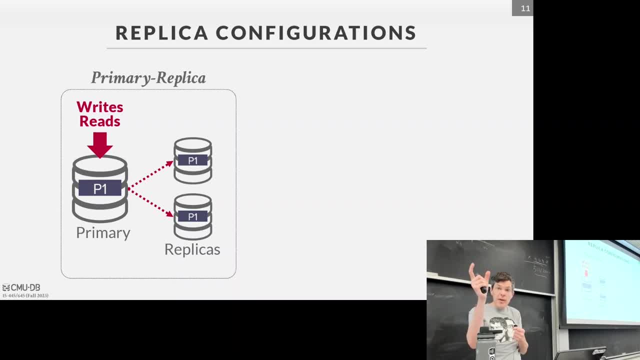 be physiological, physical, like here's the deltas of the or the diffs I'm making on single pages, or it could be the queries. if you send the queries, things get tricky because now, like things in the query, like time stamps or random, you got to make sure that the replicas execute. 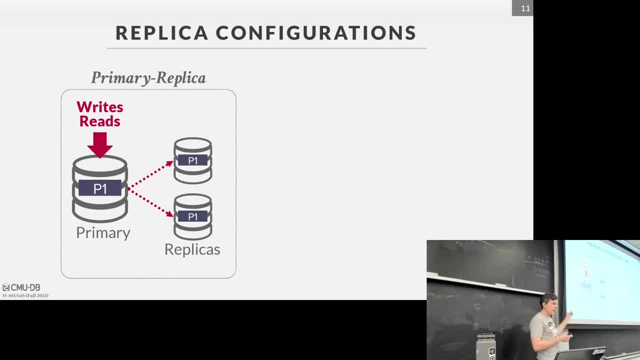 the exact same. uh, you know, have the exact same values for those functions when they run and there's tricks to handle that right and, as I said, in some systems they'll allow you to run read-only queries on on the replicas. now, how you actually find these replicas. that's that, coordinator. 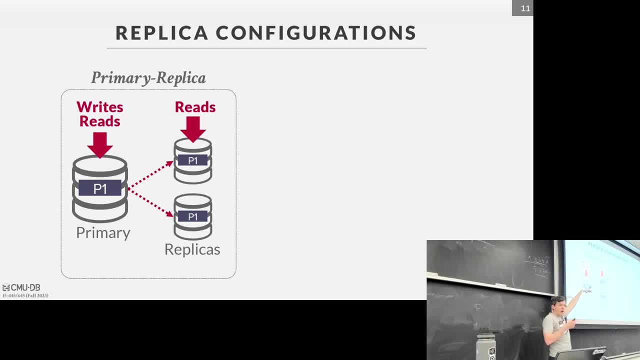 middleware, stuff we talked about before. right, you can either explicitly in your application say: oh, I know, here's the IP address of some replica, let me go. let me go send my query there. or you send it to middleware and says: oh, this is read-only, let me send it to the replica. all right, and so if you? 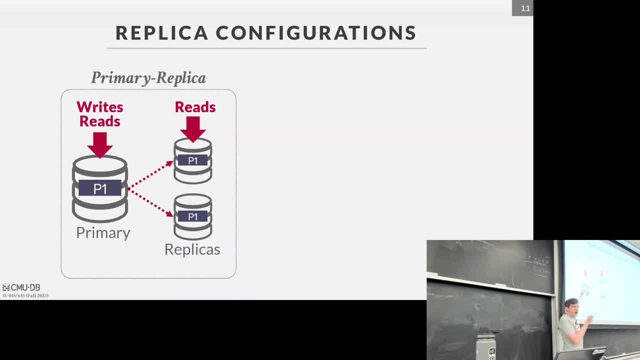 can offload all the reads to the replicas, then this thing's just doing nothing but rights, which are going to always typically be slower. so this allows you a lot of taking the overhead and the burden off of a running read queries and put it on the replicas. some cases this is okay, like if 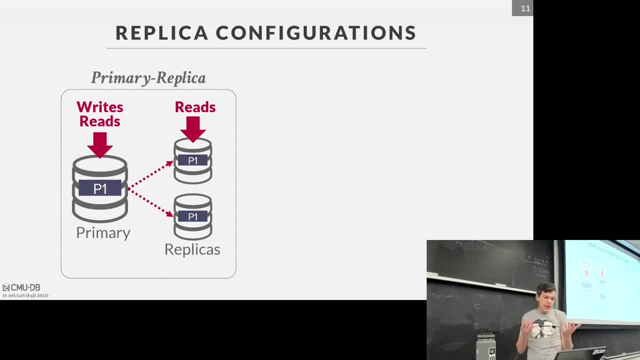 you again, if you don't really care about having the most up-to-date uh view of the database, which will be reoccurring theme throughout the entire lecture, then this is fine. but if you need to have exactly here's the most latest version, uh, then you, you know you have to run to the primary because 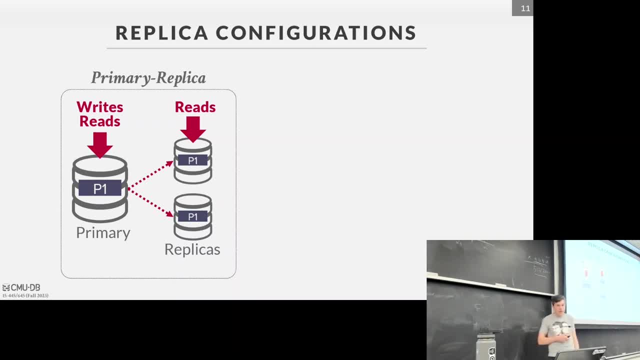 I haven't said yet how long is this going to take. right, we'll get there in a second. so in multi-primary you have again the every node can is considered the primary, or uh and can take reads and writes. so now, what happens if you have a two, uh, two transactions that do rights, uh, you. 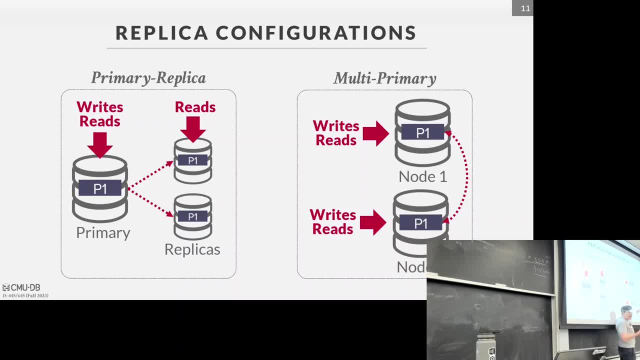 know one down here when I hear: get to propagate those updates across these guys. and then the slide, you know, coordinate who's allowed to commit and see the latest version, right. so this is less common, because this is hard to do, um, and a lot of times people will start with something like this and then, if this thing becomes the 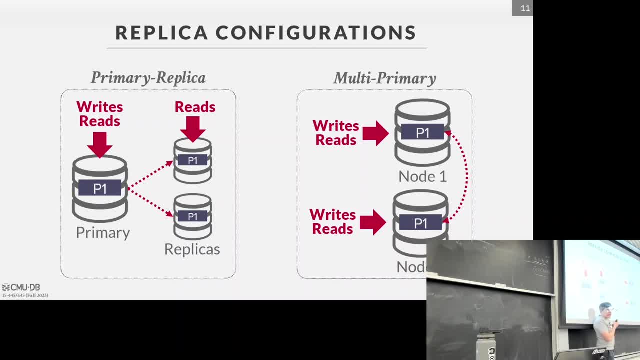 bottleneck the right node, then you got to switch to something like this: right, it actually doesn't necessarily have to be a bottleneck, all right. it could just be that the geographical distance between these- the primary and the- and the replicas are really far. when you look at it this way, the biggest model i think i want you to use is was Facebookternas today. 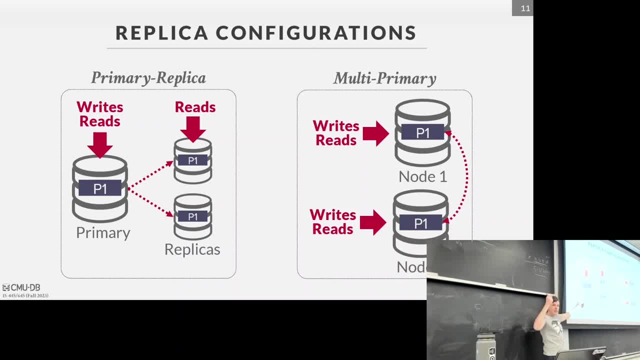 i don't think it is the first, though. the first thing to use is was Facebookreplic to use is is like in the old days, 2010ish right. so every decade agoFacebook used this model, so the data center were Somewhere in California for the primary, but then all the the replicas are all. 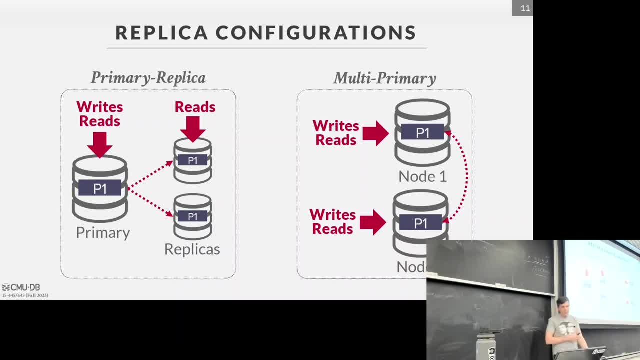 like down in brazil and whatever other countries. right, of course. what's the problem with that? okay, you have to, you know, you have to go geographical distance and you know, and get propagated back and then. so if someone like you know posts a cat picture on on their timeline, 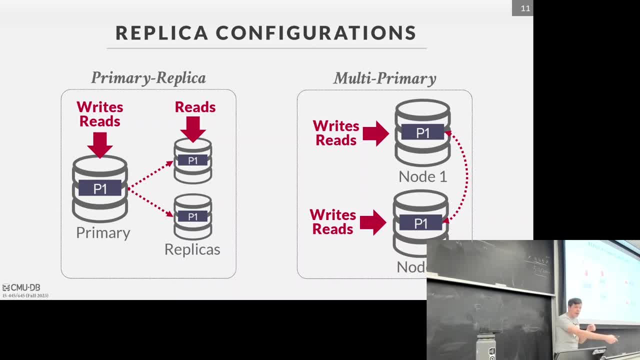 click submit but then refreshes the page that that page refresh is going to pull the data from the database, but it's going to pull from its local replica and it's not going to see the update, so people aren't going to see their own. you know timeline updates, so facebook played a. 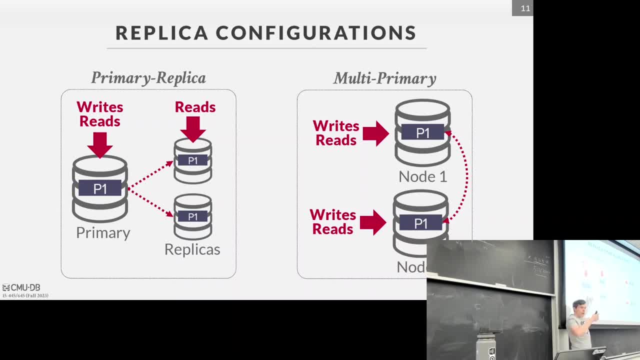 little game by putting something in a cookie in your browser so that when you refresh you saw your own rights locally, not actually from the database, right? so they hid that all that from you. but eventually you had to switch to this model because you know for doing for in things. 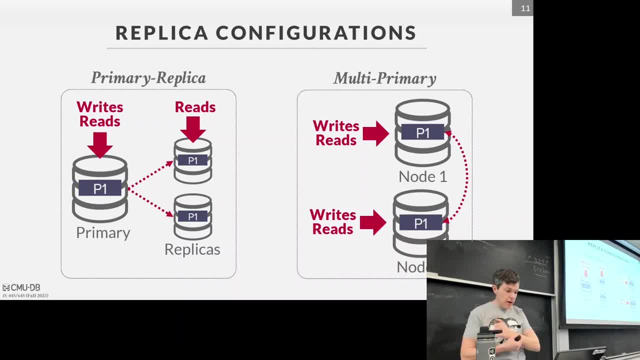 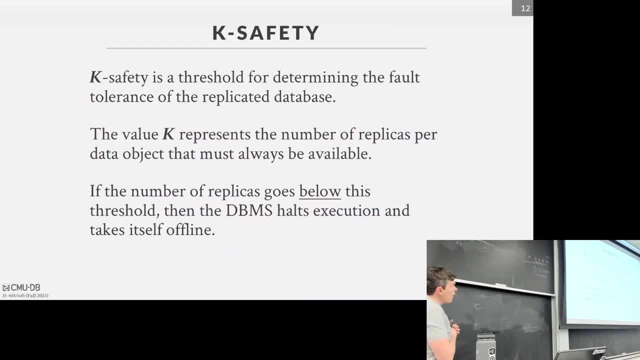 we're doing updates and you can't put the browser cookie trick in. uh, you know they had to. they had to scale it this way, all right. so next issue we got to consider is case safety, and this is a, a. i think this is primarily a database term, but the idea here is that it's the number of failures. 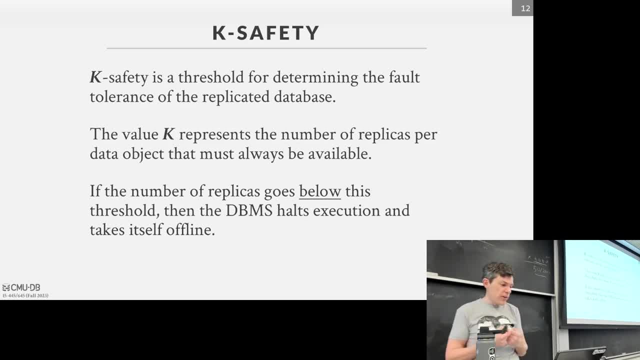 your distributed database is going to be allowed to have before it decides that, uh, it doesn't want to proceed any further because it may end up losing data if there's, if there's more failures, right, this is sort of like you know, think like a quorum, right? same same kind of ideas that we 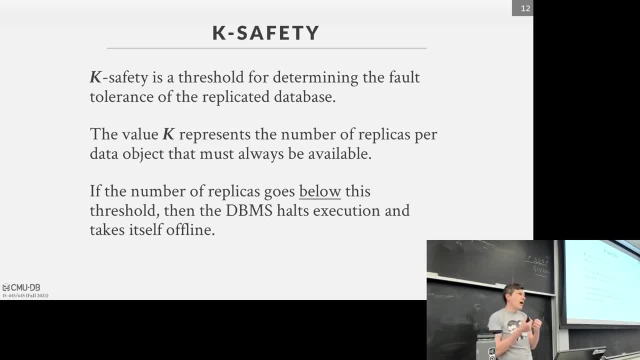 talked about before, but it's basically saying how many times, how many nodes can go down for a uh, for all the replicas i have of a given object in my database, before i decide that this is enough. right, and we'll see this in a sec when we talk about the cap theorem. 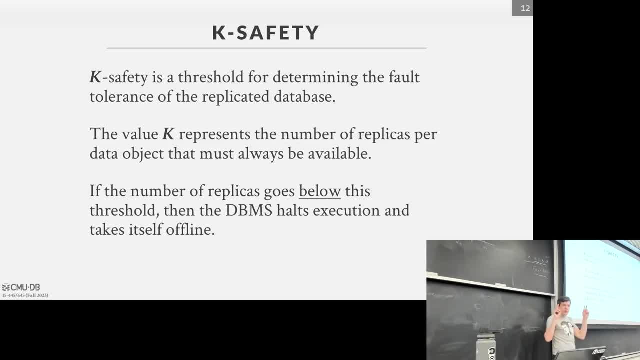 but like in a distributed relational database, like a well see traditional, but like a in the relational database world we typically we don't like losing data. we care about acid and so we don't want to have a bunch of nodes go down and say there's like one last copy of a of an object we do a write to. 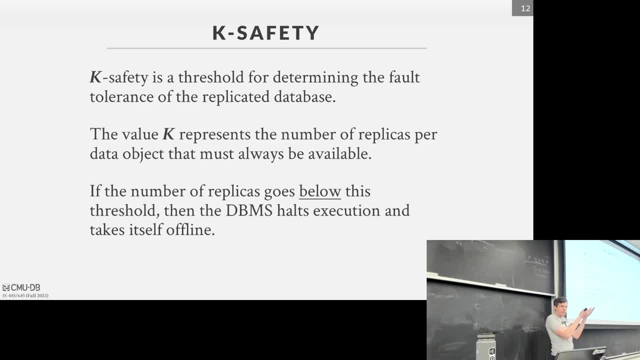 it. but then we crash and then now there's: you know that we, you know that portion of the database is now missing. so sometimes you would say i'll, i need to have at least two copies of every object in my database, for my data is considered online if i go, if i, if i go below that threshold. 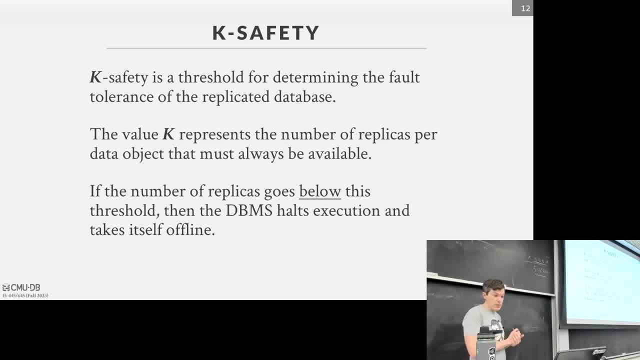 then the system just stops, it doesn't accept any new requests. there's, there's self-healing models. there's, there's other tricks like that you can say: all right, i've gone below the threshold, so let me make a copy of this data now, before i run any queries, so that you know, now you know i can start. 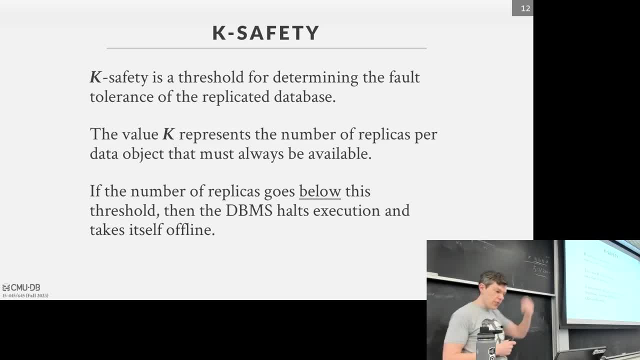 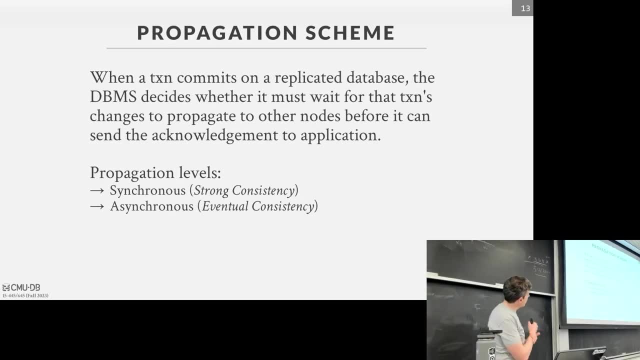 running more, running more queries after i make another copy to go above the threshold, and there's different ways to handle that. all right, so i've already alluded to this as well. the next is the propagation scheme. so this is how we're going to decide when and how we will propagate the changes from a primary 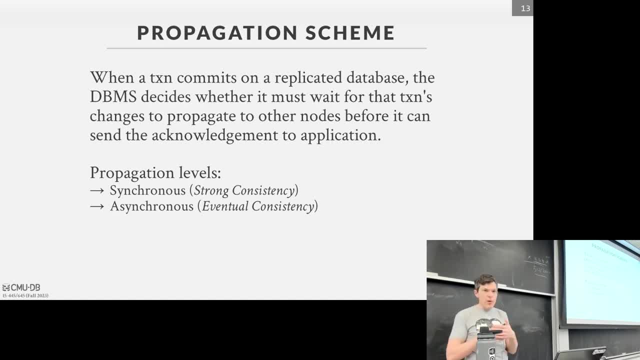 to a replica, and this is whether it's the primary replica model or the, the multi-home, multi-primary model, right, and there's basically two approaches and there's obviously there's different degrees of of uh, propagation or strength you want to have between these different um, these different uh, these two approaches. but we'll just take the, the, the two major ones, the. 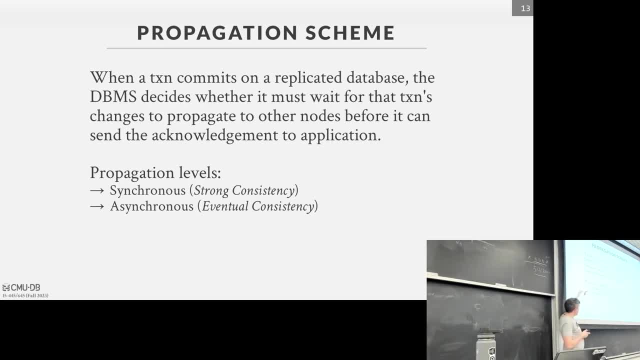 two, the two extremes. the first is synchronous commits, or what is called strong consistency in the distributed data this world, or distributed systems world. the guy here is that if i do an update to an object that may have multiple copies on multiple replicas, then i don't get an. 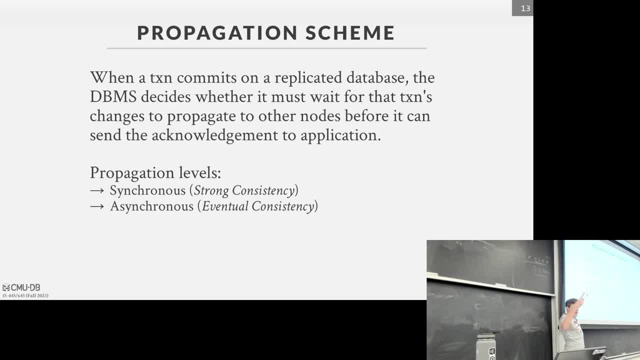 acknowledgement back my application that my change has been committed or saved until all the replicas have been updated and agreed to have been updated. right, they agreed the transaction has committed. eventual consistency means that if i do it right it'll eventually get propagated to the replicas. but i'll get a response back. 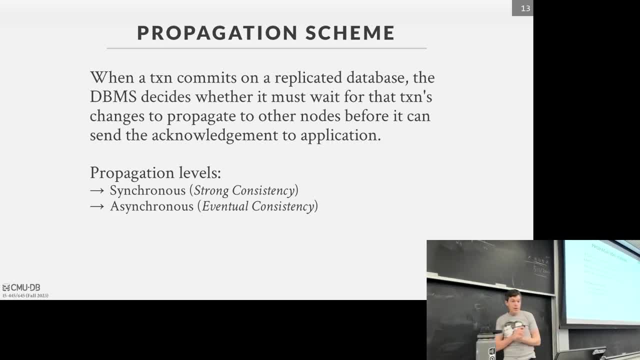 potentially before they they get updated. so if you have yes question right. so this question is: how do you make sure you're eventually you'll be eventually consistent. if there's no guarantee that you get a response, we'll get there in a second. yes, the answer is. 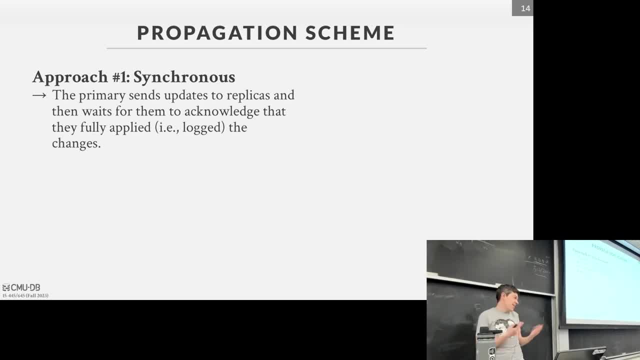 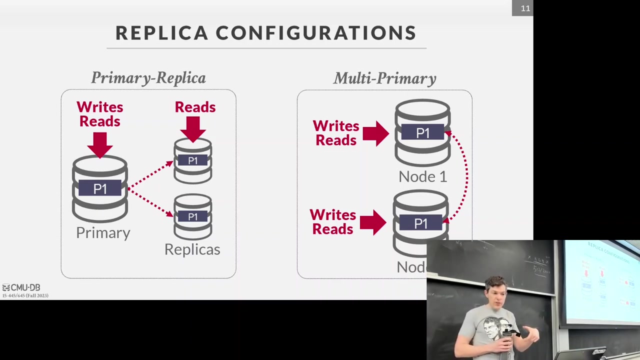 right, like you'll get there eventually. but when other questions: yes, because you allow rights on both the primary nodes, yeah, go back here. so the question is: in multi-primary, how do i prevent writes from occurring on the same object? two-phase locking- OCC. So you basically you run two-phase locking across multiple nodes, right? 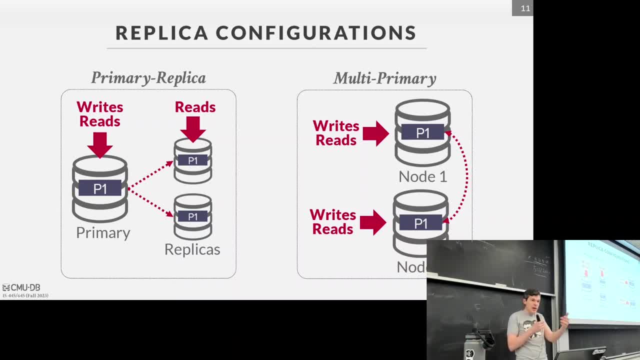 Again, it's just the same protocols. it's just now we're distributed and now, like someone's going to have to build the weights for a graph, assuming it's two-phase locking and someone's going to have to decide, 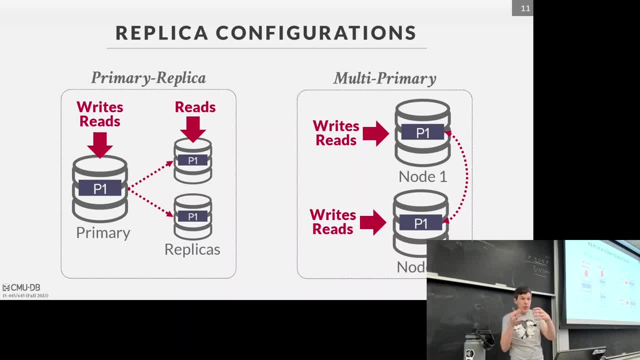 okay, there's a deadlock, let me go ahead and kill it, And that could be either the centralized coordinator or it could be amongst the nodes. they say, okay, well, I'm waiting for this and you have this, but you update it. 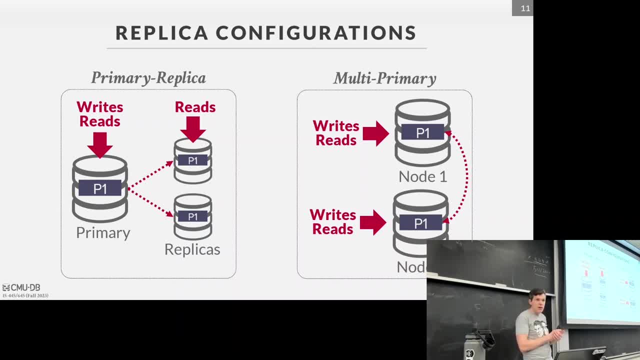 And then the two nodes decide: okay, yeah, there's a deadlock here, and then there's some other ordering team to decide, determine the priority of who gets killed. So all the stuff we talked about before is still here. So we don't worry about, say, the network traffic or anything like that. 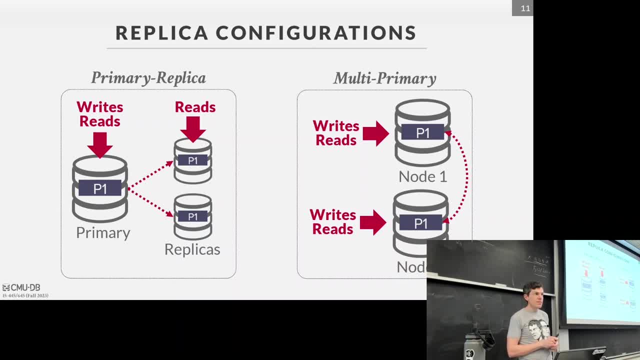 What do you say? we don't worry about the network traffic, So the latency in terms of updating any data structure, you have to keep account of the loss. so that would not be the same as if there's an issue with this. Yeah, so the statement is: 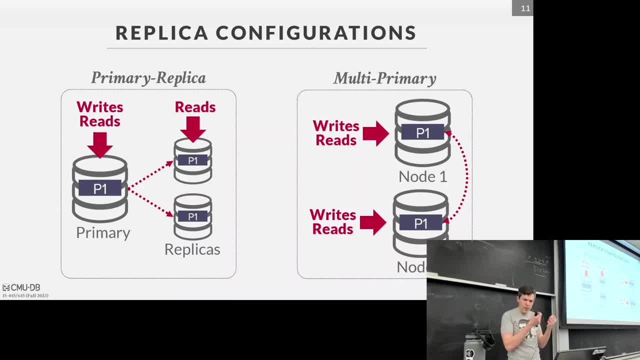 and he's correct that- in a distributed system- and we said this before- between parallel systems and distributed systems- in a distributed system the communication latency is going to be much higher, the cost is much higher. We do worry about it, but there's no magic wand to make it go away. 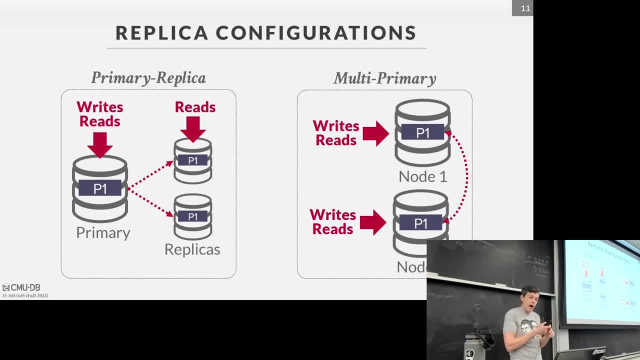 We're kind of limited by the speed of light, So we will see this in a second. The trick they basically do is say: well, I'll wait for a certain amount of time to see whether someone shows up. they may conflict with my transaction. 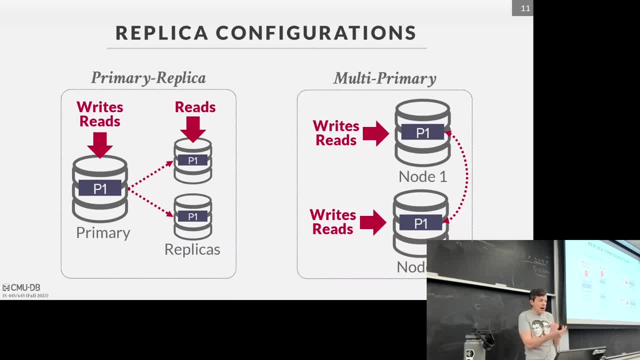 and if they don't show up in that time, then I'm allowed to commit. But there's no way to get around that. There's no magic two-phase locking you can do because you're going to the wide area network. It's going to be basically the stuff we talked about before. 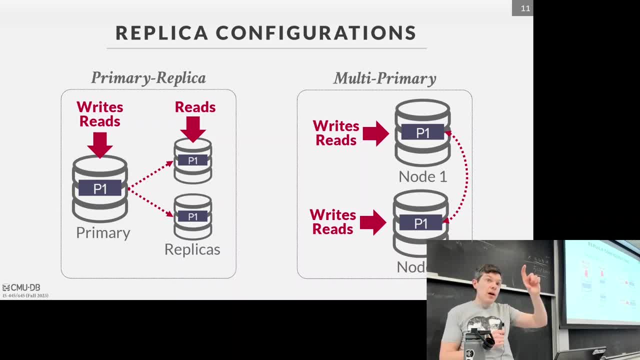 And the tricks, the games they play, is: how much hints can you pass along to say, okay, yeah, by the way, I'm going to, instead of saying one message at a time. here's all the locks you need to acquire. 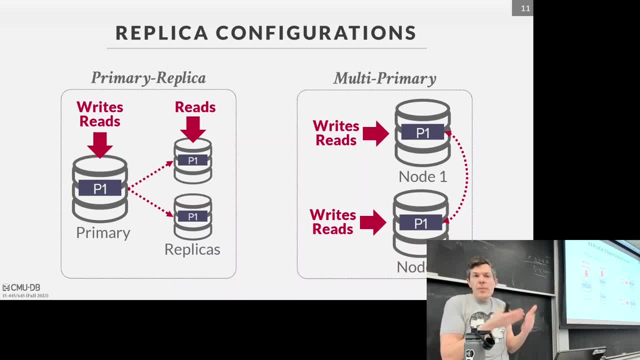 it's like: here's the locks I'm going to acquire, and here's the locks I think I'm going to acquire, and maybe you do more pessimistic things like that. That's really all you really can do. Okay, Let's go back. 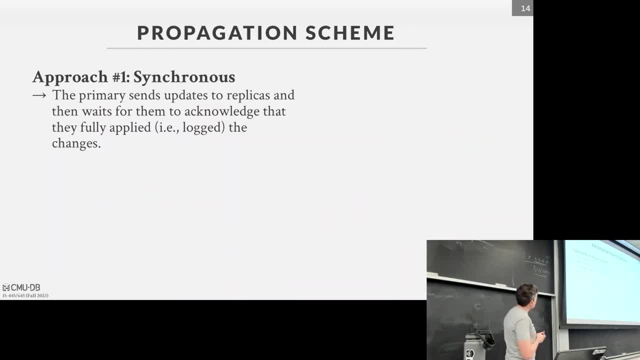 All right, propagation theme. So synchronous commit or synchronous propagation. So the idea here is that when the primary sends a, when the application sends a commit request to the primary, the primary will send that request to all its replicas and it has to wait until they come back and say: 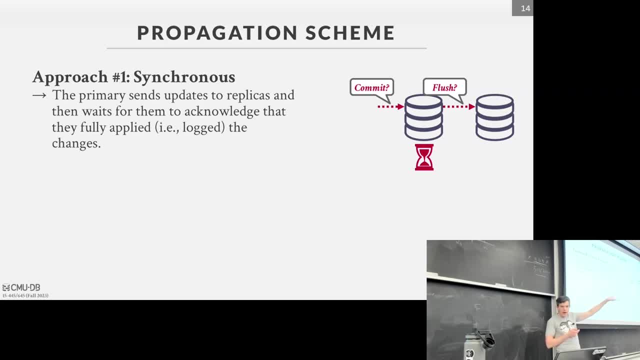 yes, I've got this change. I've go ahead and committed. I flushed the changes to the disk and then, once it gets acknowledgement from all its replicas that things are durable and safe or there's transactions allowed to commit, then, and only then, can it propagate the acknowledgement. 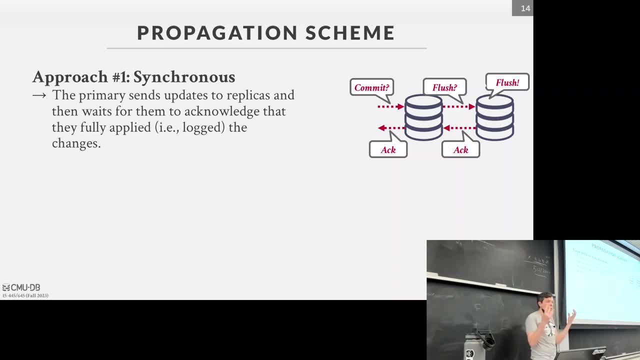 back to the primary. It's just like before, when we committed transactions with the write-ahead log, except now we've got to wait for somebody else over the network to come back and say they got it too. A synchronous commit at a high level is basically: 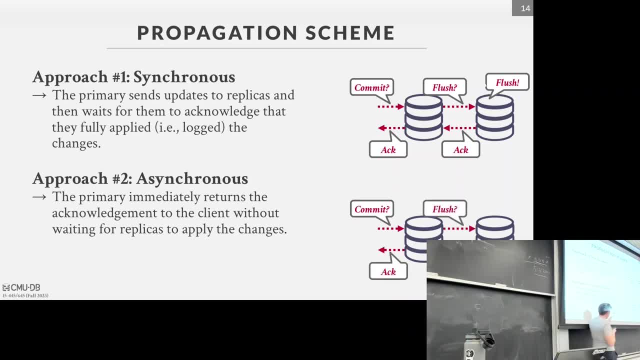 all right, commit message shows up. I'll send the request to my replicas, but I'm not going to wait for them to come back. I'll immediately say yep, I got it, commit And what I was saying before that. there's sort of like. 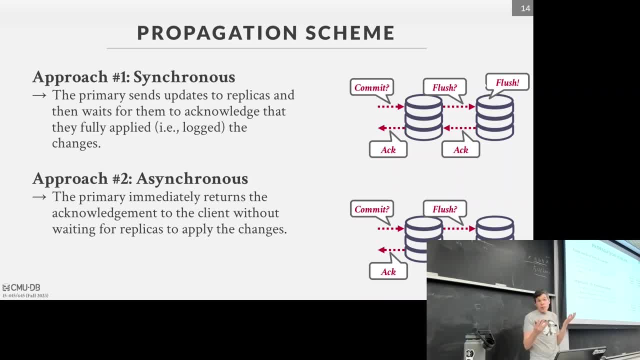 you know these are two extremes. there's a bunch of games you can play about. how much can you really wait or how much should you wait right? So going back here to the one at the top, so say there was like four replicas. 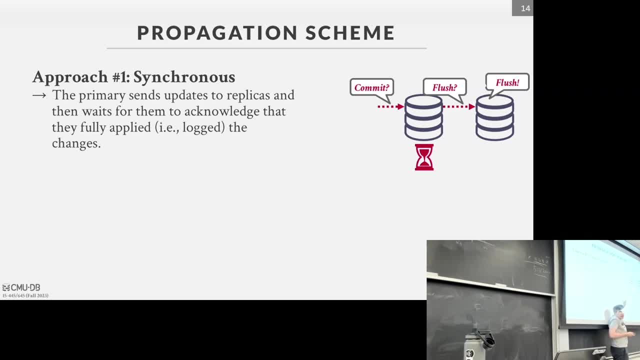 but instead of waiting for acknowledgement from all four, maybe I waited for two out of four or one out of four. So at least know it's propagated on at least one right. Same thing for the asynchronous one right. So I send my request. 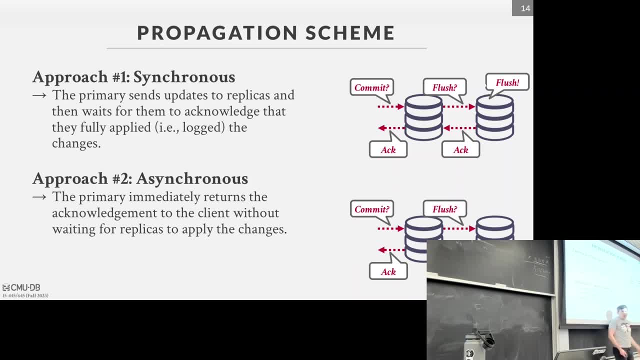 I send my requests out. maybe I wait for some of them. We saw this with consistent hashing in Cassandra. right, They do. quorum writes, so you could say: all right, every tuple is replicated three times. I'll wait for two out of three responses from my replicas. 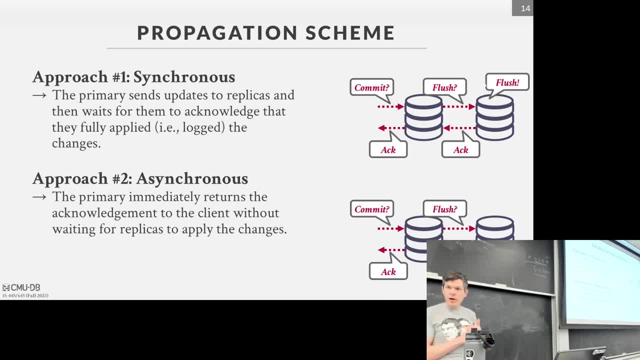 before I say: tell the outside world that my data's been saved. I don't want to use the term transaction committed in Cassandra because they don't. newer versions maybe support it, but not the older versions. They didn't support multi-object updates. 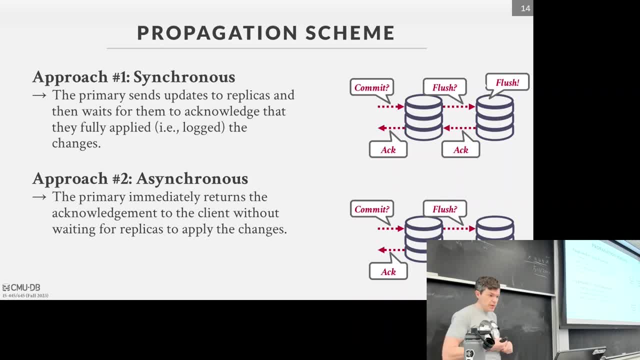 They didn't support transactions. They definitely didn't support multi-node transactions. For our purposes, assume that we're updating things just on a single node. So again, there's pros and cons to all of these, right, And there isn't one scheme that's gonna be universal. for everyone. it depends on the tolerance of the organization or the company running your database and depends on what the application is. If it's like posts on Reddit and Twitter and Hacker News, then, like you know, if I lose something, eh, maybe no big deal, right. 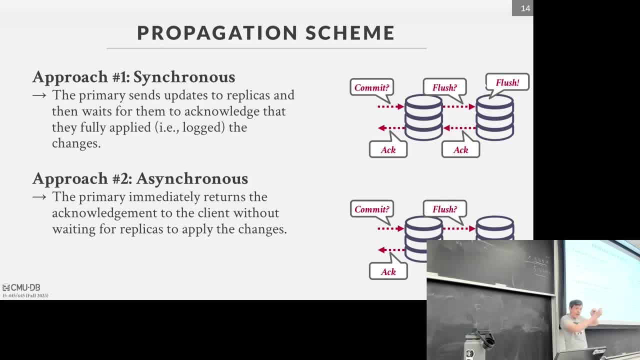 But if it's your bank, then you don't wanna lose anything and you wanna make sure everything is fully committed. And so the NoSQL guys are saying, oh yeah, you don't wanna be to be web scale support. you know online applications, a lot of users. 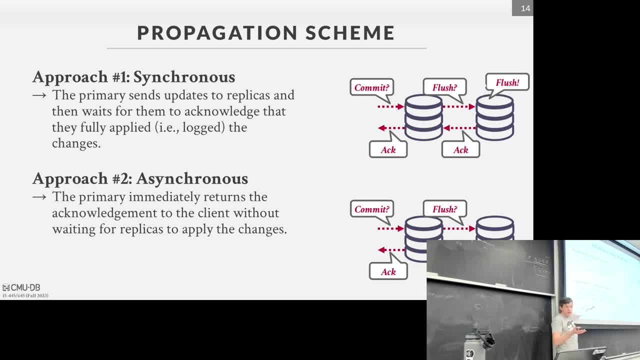 you wanna use asynchronous commit or eventual consistency, And then the traditional database, people will say, oh, you don't wanna lose any data and you wanna do, you know. you don't wanna lose any data and you wanna you know. 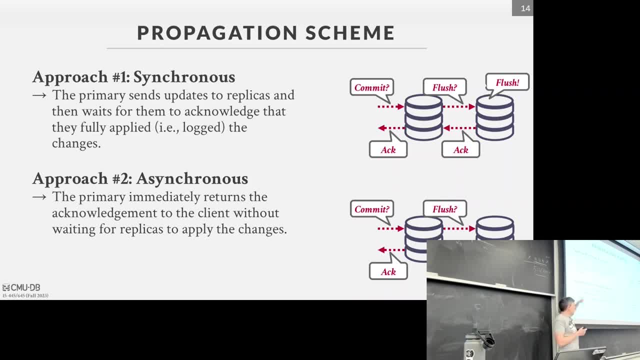 when you want fully-asseted transactions, even though you're across multiple nodes. And so the answer is again: the correct answer is: it's somewhere in between: Some applications, yes, some applications, no. The difference with the NoSQL guys. 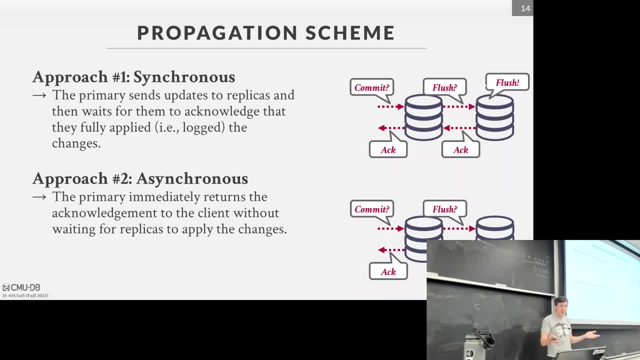 they said straight up no, and they never had it, at least in the beginning, and they eventually had to add it back, Whereas the relational database system started off adding transactions and then they eventually relaxed it a little bit And I would argue it's better off starting with a, you know. full transactional, strong consistency support, and then they eventually relaxed it a little bit And I would argue it's better off starting with a, you know, full transactional, strong consistency support, and then they eventually relaxed it a little bit And I would argue it's better off starting with a, you know, 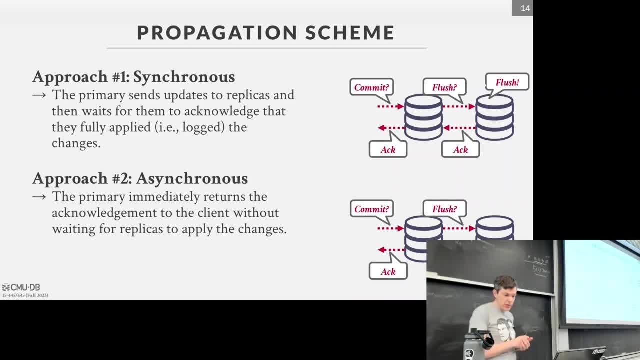 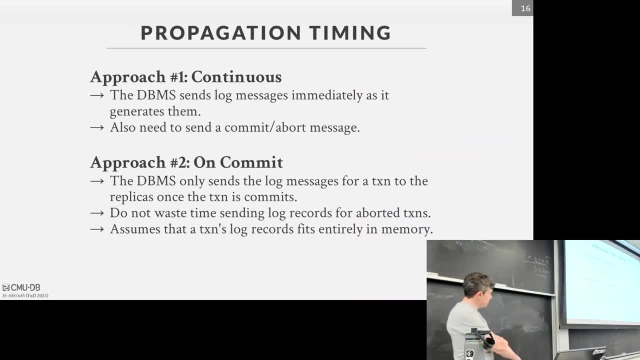 full transactional, strong consistency support and then dial it back as needed, rather than like trying to shoehorn it after you've already built the system. All right, the next is: when are the changes actually propagated? So again in my example here: 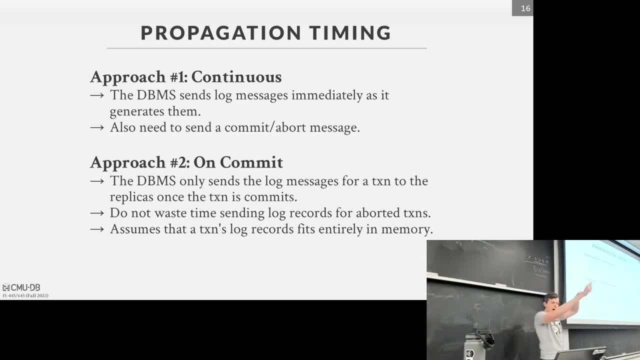 I just showed like on commit. tell the outside, you know, tell the other replica. I wanna go ahead and apply my changes, But let's say that I'm doing a transactional update. it's a lot of data and it's a lot of round trips. 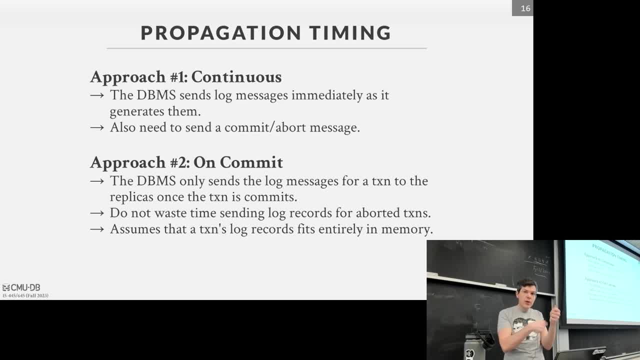 between the application server and the data server because, like, do one update, do another update and so forth. Do I wanna wait for the I get the commit message before I propagate those changes to the replica? Maybe not right? 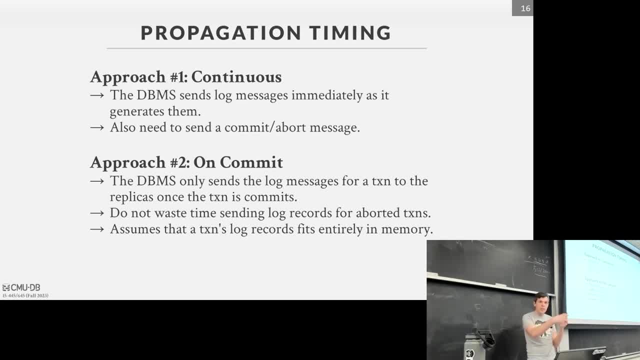 Because maybe, like as the updates come in, I can start sending them piecemeal to the replicas so that when I go ahead and commit, you know, they don't have to apply a bunch of those changes. they've already seen a bunch of those things. 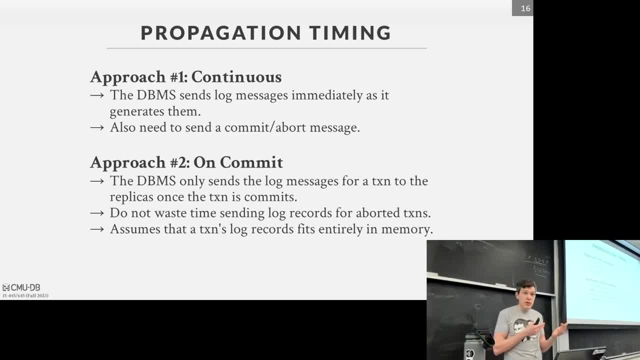 But then that now means that if I roll back the transaction, they've already applied a bunch of changes that I have to then reverse. But again, this is sort of like what I was saying before, like the replicas are more or less in recovery mode. 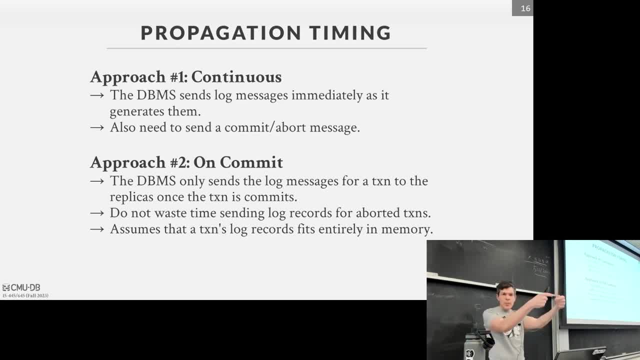 ignoring multi-home like because they're just replaying these log messages and they're maintaining the undo state or undo buffer, just as you would during regular recovery. So most systems do the top one. If you do the bottom one, it does make it easier to implement. 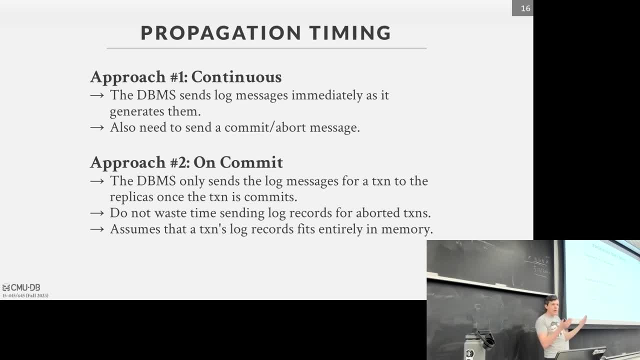 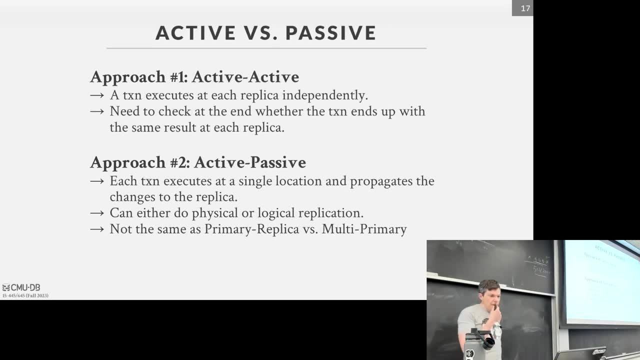 but again it makes the commit process a bit longer because now you batch up a bunch of updates you have to apply. All right, this one's a bit nuanced and always confuses the students, so ask questions if it just makes sense. 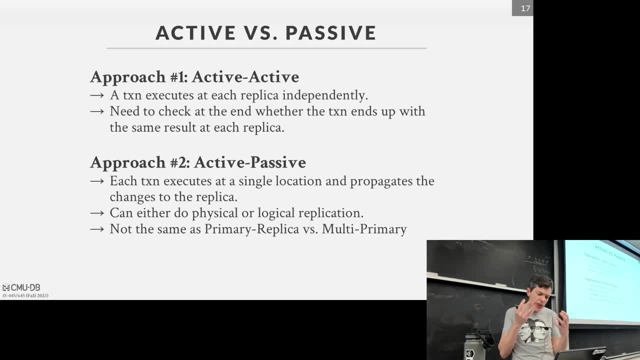 So then there's the question of what are the transactions actually, or what are the nodes actually doing that are involved in, say like a multi-node transaction, And so the two ideas are active-active versus active-passive. So active-passive is what I've been sort of describing so far. 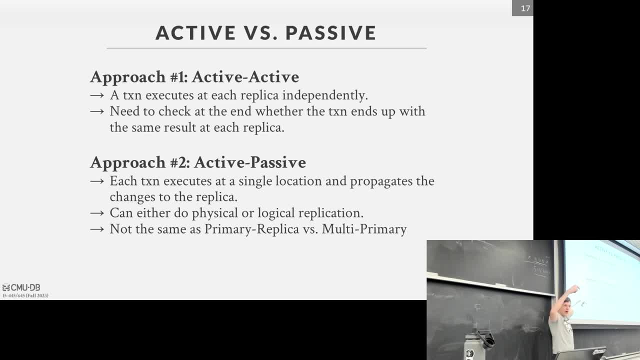 where there's some primary, the queries go there, they do updates and then they get propagated to the replicas and the replicas are eventually. they're not really running the queries, they're doing the work, they're just replaying the updates. 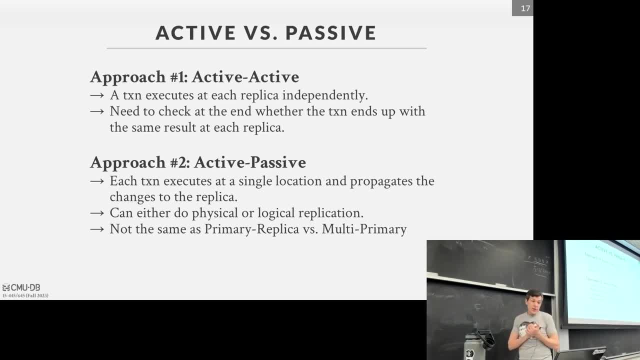 that occurred on the primary With active-active. the idea is that when I execute a transaction, it's gonna actually execute the logic of that transaction at every replica and that when you go to now commit you don't need to send like. 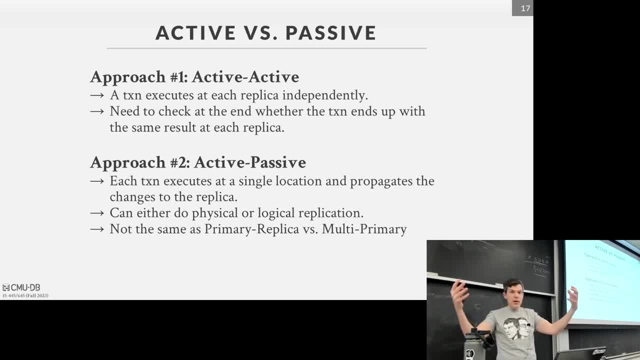 hey, here's my updates from the write-ahead log, because they all did the same thing. I think of, like I have an update query ignoring random, ignoring times and all that other stuff. then, like assuming I can execute it deterministically. I send it to the two, the two nodes, and they're both executed in the exact same order and produce the exact same result. so now, when they go to commit, they just need to agree: yep, I did this, yep, you did that, and you're done. 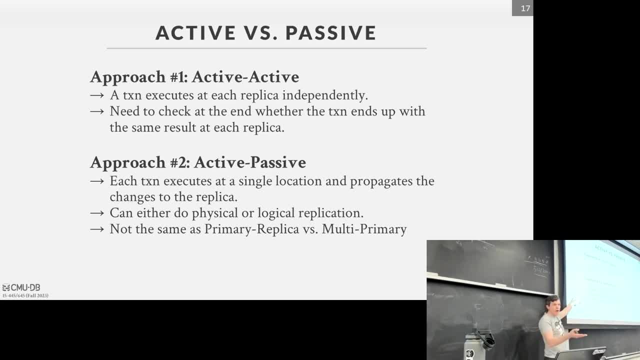 So most systems do this bottom one because it's just easier, because again you're just piggybacking off of the, you're piggybacking off of the write-ahead log mechanism. but the top one is: if you can do it. 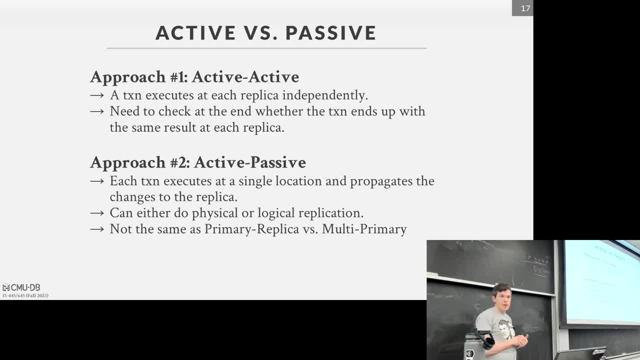 it's way more efficient because you're just sending less data. Similar to that: the push versus pushing the data. sorry, pushing the query to the data versus pulling the data to the query. yes, Does active-active kind of defeat the purpose? 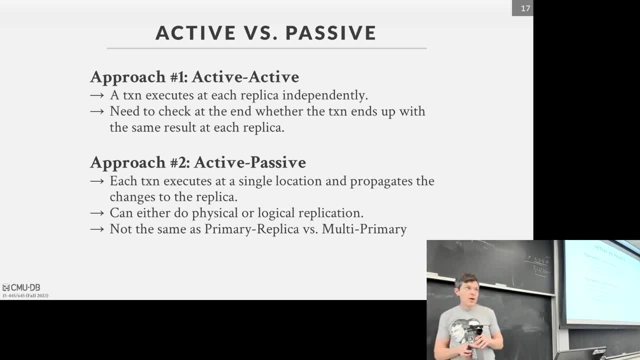 of being able to run a lot of read queries on. The question is: does active-active defeat the purpose of being able to run a lot of read queries on replicas? Yes, So like when would you want to use? The question is: when would you want to do this? 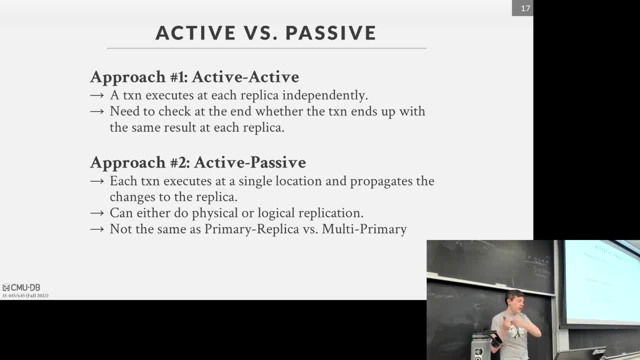 If the, if the amount of data you have to send to say here's the transaction is gonna be less than, like here's, the write-ahead log updates, then it may potentially use better. It also reduce shrinks the window. 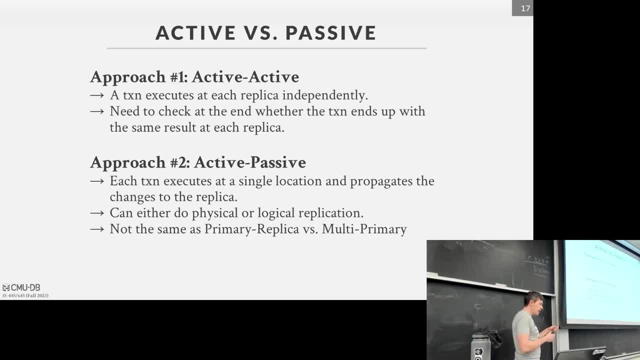 of the synchronization time as well, because now, like again, assuming the two nodes have the same speed, send the request, they rip through it and then you just commit, whereas like think of the other, the active-passive. 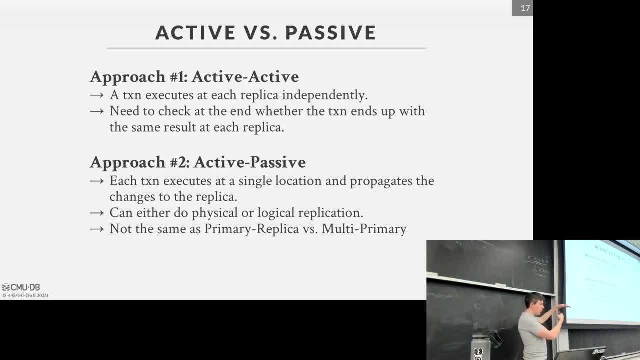 I gotta run the query, generate the write-ahead log messages. after I run the query, then send the updates that then get propagated, whereas the other two can potentially happen at the exact same time If, like, they don't end up with the same result. 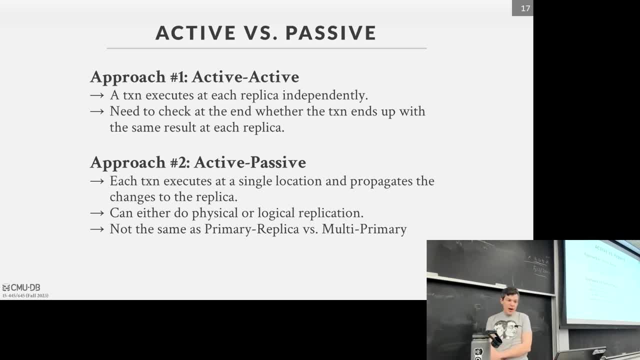 Or like that one. The question is: if you do active-active and they don't end up with the exact same result, what do you do? You have to abort the transaction. That's why most people don't do it. 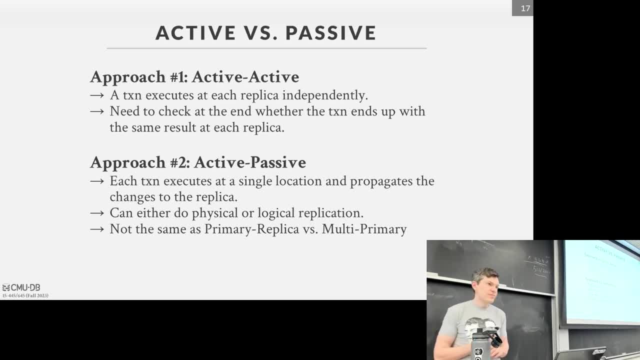 Yeah, Yes. So with active-passive, wouldn't we need to spend a lot more traffic over and above it? The question is, with active-active, wouldn't you like Active-Active? wouldn't you need to send a lot more data? 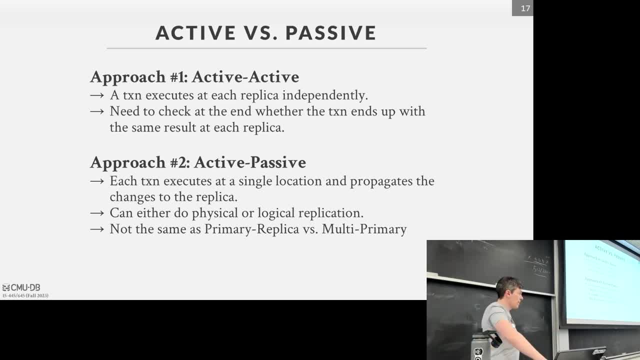 over the network. Why? Because for each query you'll have to send a message. Instead, with Active-Active, you're going to send the whole log over at the same time. So the statement is: and the answer is, of course. 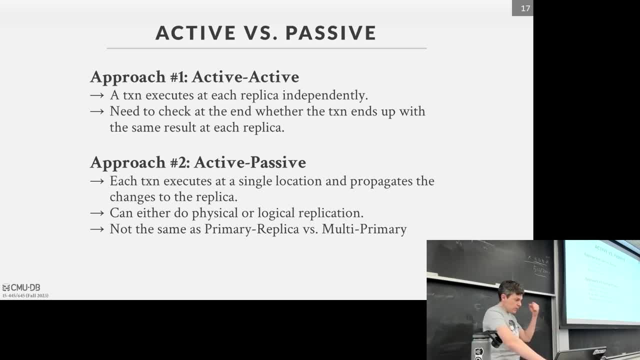 in data. it depends The statement is. with Active-Active, you would have to send the query. With Active-Passive, you'd have to send a write-ahead log. And couldn't the write-ahead log, the records, be larger than the query? 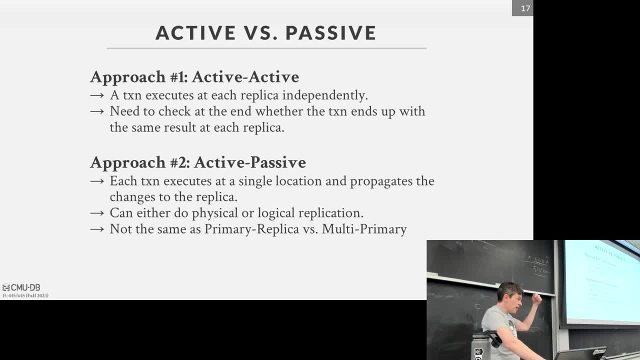 Well, it depends. I have a single update query that updates a billion tuples and I could just send that single string and that's enough to update a billion things. So I don't want to go too much into this, but to handle. 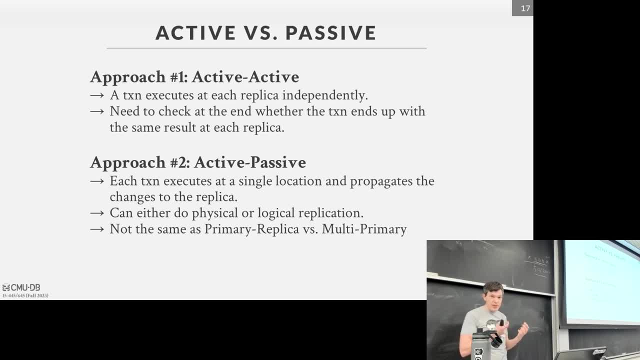 all of these problems. if you can run your transactions as stored procedures- which we haven't really talked about, but think of like an RPC- I literally have a function that I can put inside my database system that has if-then-else statements- things you can't easily do in SQL for loops. 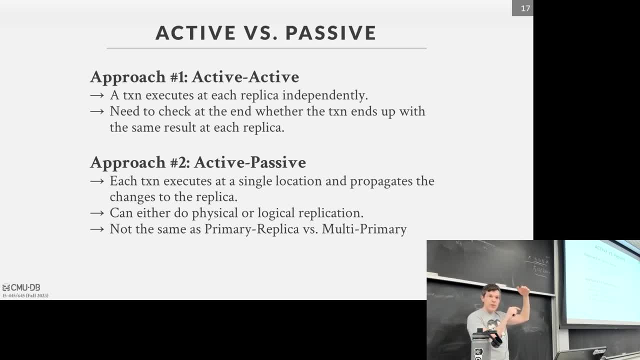 and all that. It's a procedural code that then makes invocations of SQL queries. Now the application, once it runs a transaction, doesn't say OK, begin a transaction, update this query, get a response, update next query, and so forth. 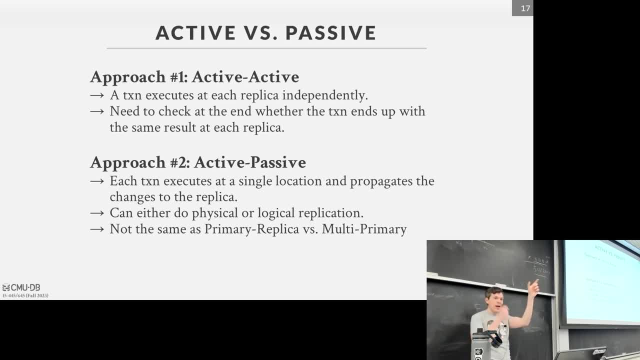 You literally say: execute this function with this input parameters and then that runs on the database server. This is very common in enterprise systems and older systems, And so if you can run everything as stored procedures now the database system actually can look inside the code. 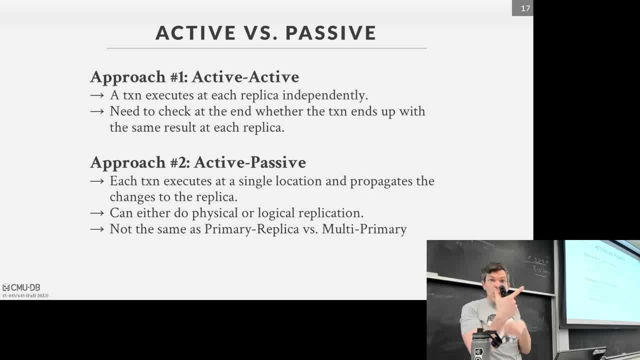 and figure out what's going on and flag anything. Oh, there's a timestamp call, There's a random function and so forth, And then you can play a bunch of games of making sure that when you send that function request to the different servers. 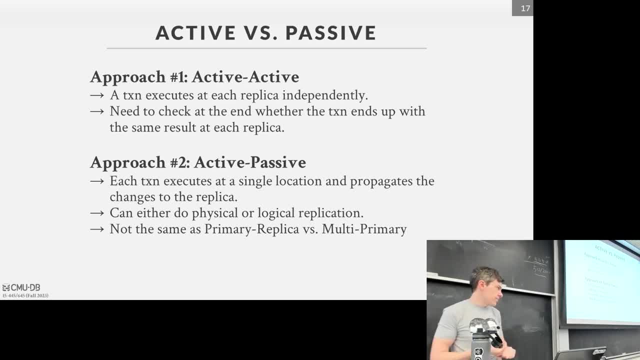 that do active-active replication, it's guaranteed to execute in the exact same order. Actually, the way you handle random and timestamp is you basically piggyback on. the request has to go to one server. that server then signs like: hey, have you ever called timestamp? 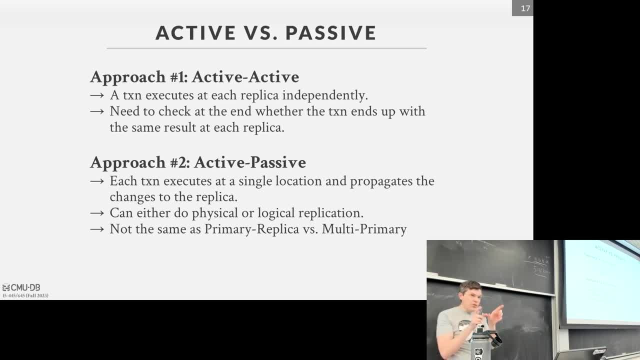 Here's the timestamp. Have you ever called random? Here's the starting seed, And then that way you send that information, along with the, the request, to any other server, So when they execute it, they'll get things running in the exact same order. 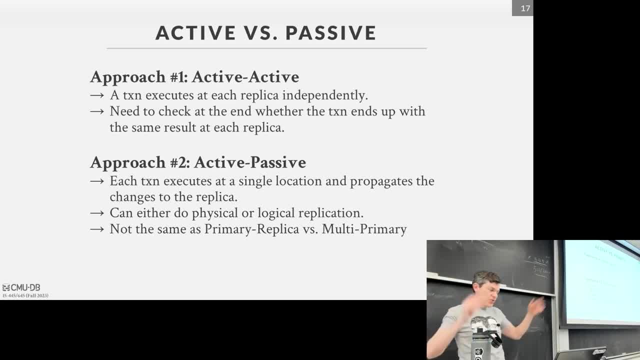 That assumes, though, you're running transaction requests in the exact same order, which you can do with serializability, And that's why we care about that. Again, most systems will be active-passive, But there's active-active, if you can do it. 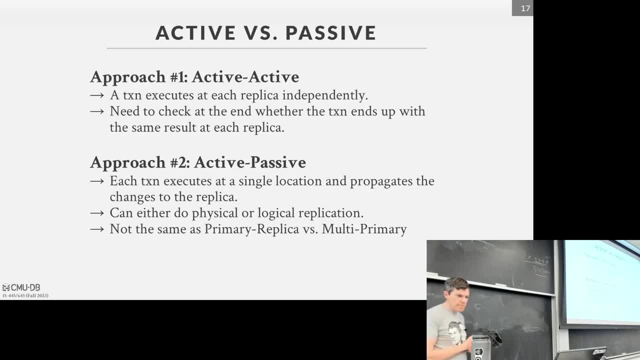 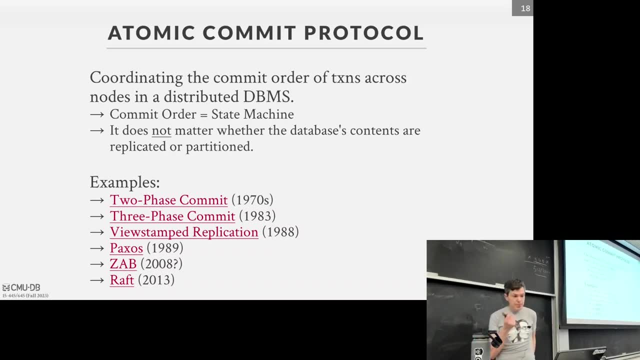 Not all systems can, Provides a lot of benefits, All right. So now we've got to talk about how we actually want to get everyone to agree that we want to commit transactions. And, out of curiosity, who here has taken a distributed systems course either? CMU? 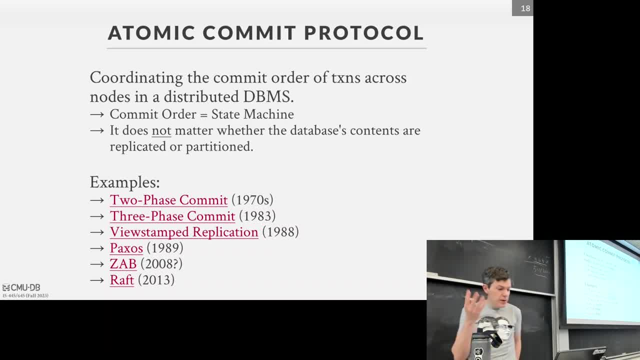 or somewhere else. All right, So more than half OK. So some of this will be somewhat redundant, But again I want to focus on the things we care about in the context of databases, And so in the distributed systems literature they'll call this state machine replication or log. 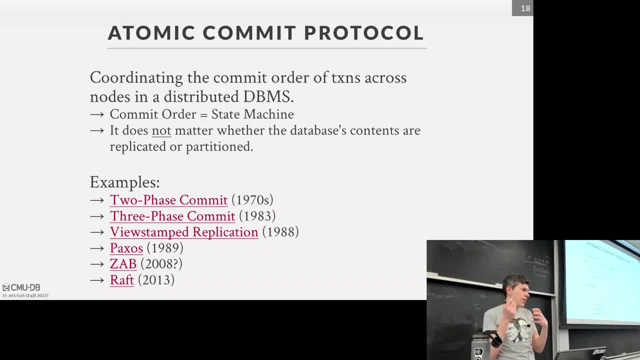 replication And the way to think about it in the context of databases. the thing we're trying to get everyone to coordinate on is the order in which transactions are committed, And that's essentially our state machine: This transaction committed, followed by this transaction and this transaction. 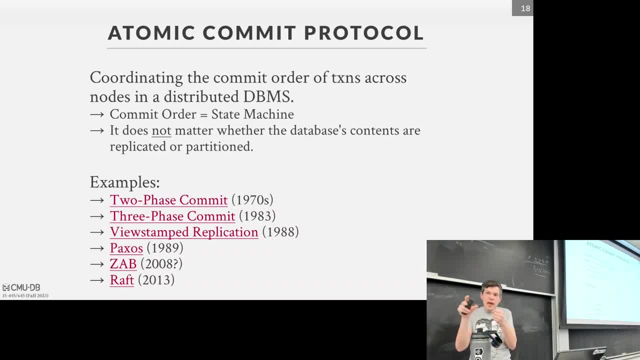 And it's not so much like here's the changes that they made. We know what the changes are because that's part of our log, But the higher level thing that we're trying to order is the commit order, Because if you say here's the commit order of my transactions, 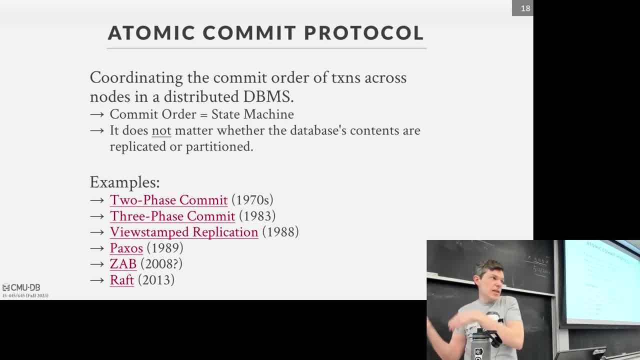 along with that is the metadata that says: here's the changes, Here's the changes that they made. So if you get the commit order right and you piggyback the changes that the transactions made, then you can propagate that to all the nodes. 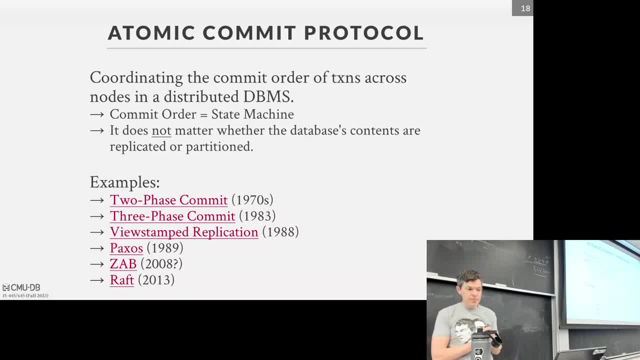 And then everyone will be synchronized in order. So the thing we'll talk about now is: this: doesn't matter whether the database system is going to be partitioned or replicated. We still want to do this to get everyone to agree that this is the order that transactions. 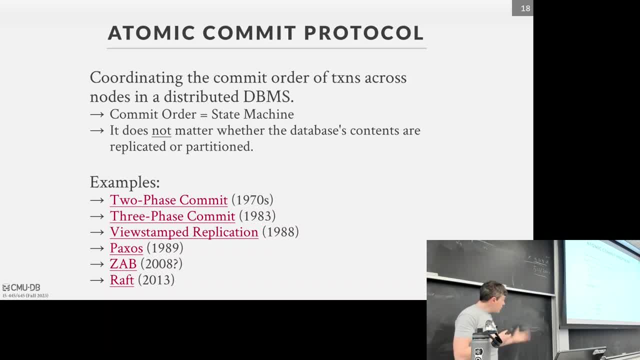 are going to commit. So there's a bunch of different pro- actually I take that back. There's not a lot of protocols that do this because it's really hard. These are the main ones that show up in databases. Two-phase commit is the original one. 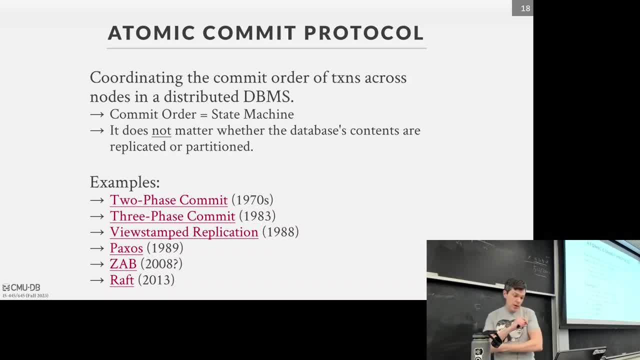 And this was originally thought to be invented by Jim Gray at IBM. He won the Tony Wooden Davis in the 90s, But there's a famous transaction book where he actually transits to this other dude in Italy who implemented two-phase commit for one of the early databases. 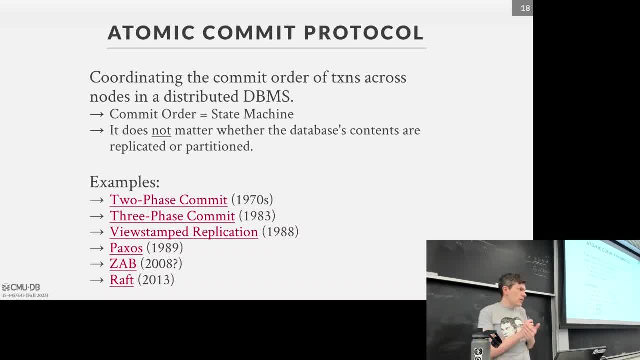 that they built for the Italian social security system in the early 1970s. But even then the idea of two-phase commit comes from the real world. It comes from contract law between legal arrangements between humans. So the idea of two-phase commit is sort of 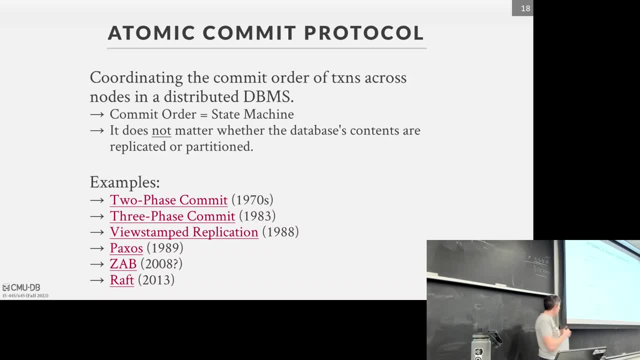 it's implemented in database systems or it's implemented in distributed systems, but the idea predates computing. Then there's three-phase commit, and that's from Stonebreaker. Nobody actually does this. We can ignore it. View stamp replication is considered to be the first consensus protocol that. 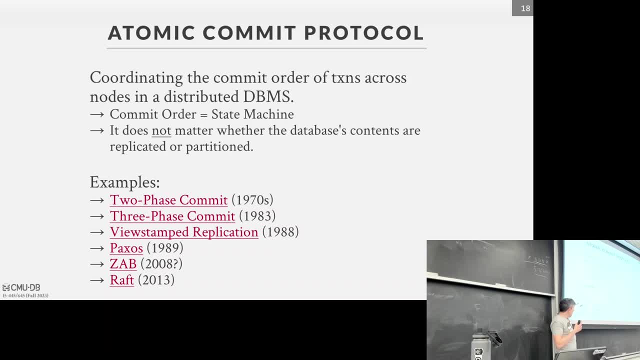 is shown to be correct. It can handle a lot of things. It can handle liveness issues, And that was invented by Barbara Liskoff, who won the Tony Award a few years ago at MIT in 1988.. Paxos is probably the one everyone's also heard about. 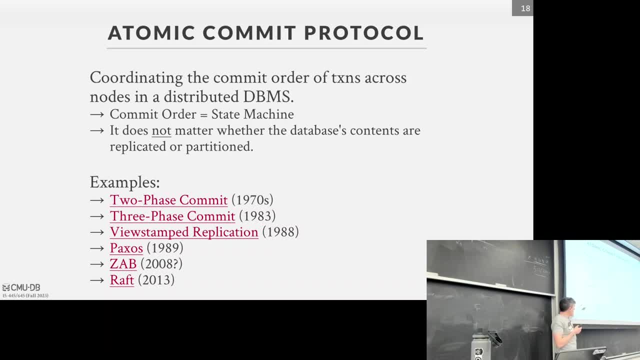 This was invented a year later, But the paper itself didn't come out till the 90s. I'll explain why. in a second ZAB is from the Apache Zookeeper people, the Zookeeper Atomic Broadcast Protocol. That's roughly 2008.. 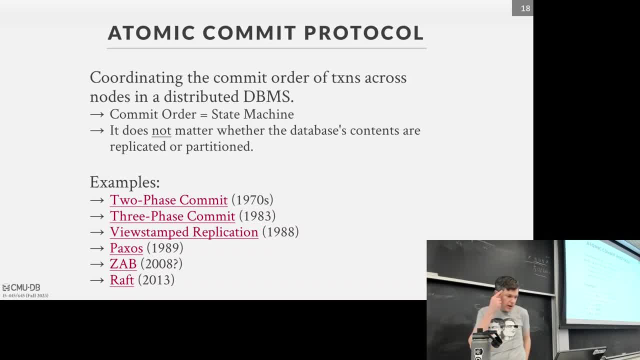 And then RAFT is another popular one that was invented at Stanford in 2013.. And this is the one that- OK, You know it's sort of in vogue now. If you're building a distributed database system, oftentimes you would use RAFT. 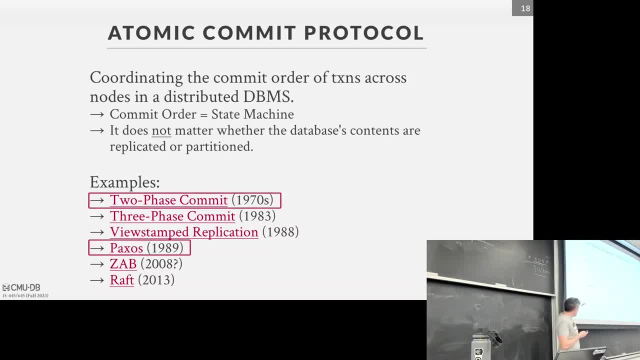 But for this talk or for this lecture, we're only going to focus on two-phase commit and Paxos. RAFT is considered to be a more readable, understandable version of Paxos And the key difference is that there's fewer node types. 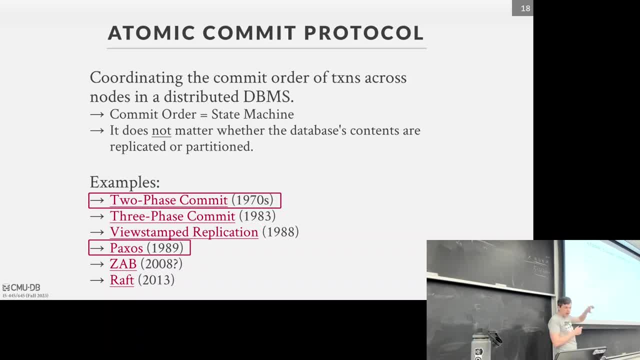 or participant types in the network And then when you do a leader election, only the nodes that have the most updated logs they're allowed to go for election. where Paxos anybody can Right View stamp replication or VSR again. 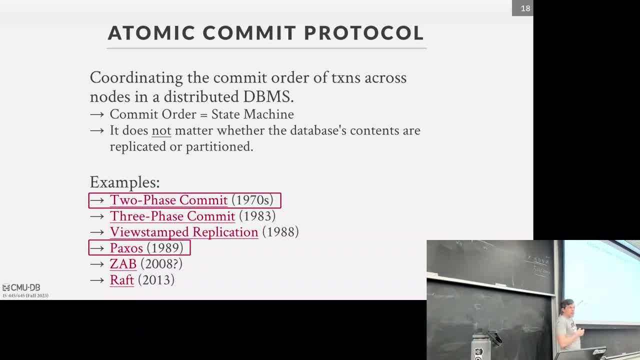 this is becoming popular now because there's a distributed database out of South Africa called Tiger Beetle. that's written in ZIG, which is like ROS but more rare, And then you also use VSR for that. OK, So here's two-phase commit. 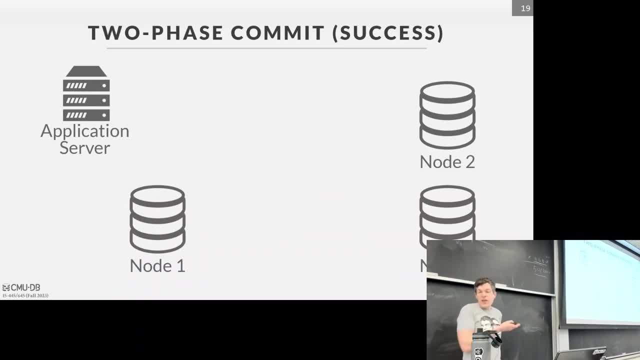 Basic idea is that there's an application server. Again, we ignore whether this is actually going through middleware or whatever. It doesn't matter. OK, They made a bunch of updates to the database. We don't care whether it's partitioned or replicated. 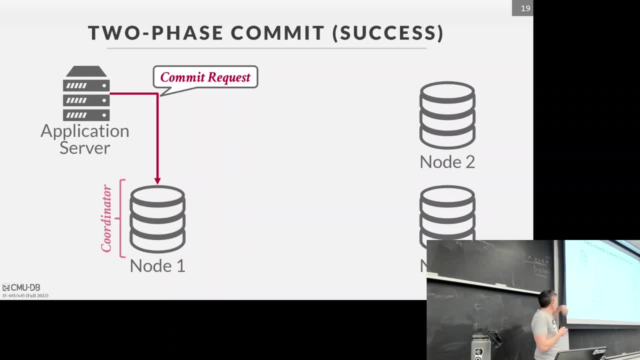 It doesn't matter. They want to say, OK, I want to commit my transaction, And so the commit request is going to be going to some node. We said it was the primary, but in the two-phase commit parlance it would be called the coordinator. 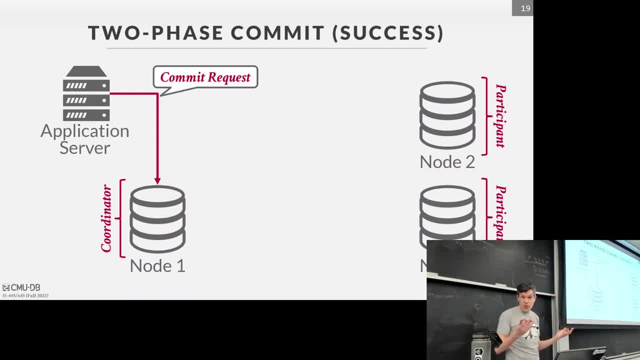 And then the other nodes that were involved in the transaction. they'll just be called participants. So two-phase commit, it is what it sounds like. right, It's two phases, So in the first phase it's called prepare phase. You send a message. 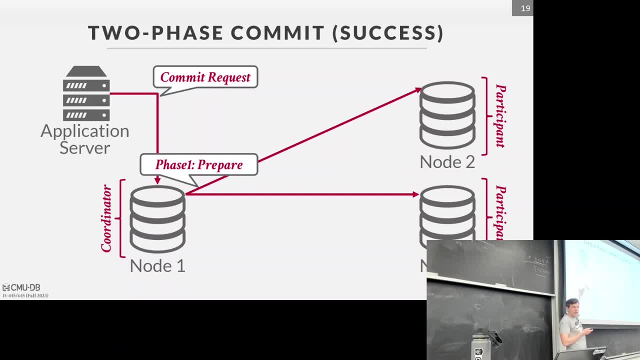 The coordinator sends a message to all the nodes. The participants will say: hey, there's this transaction, It's got this ID, whatever, whatever metadata or identification you want to use, Go ahead and prepare to commit And they come back and they vote and say yes. 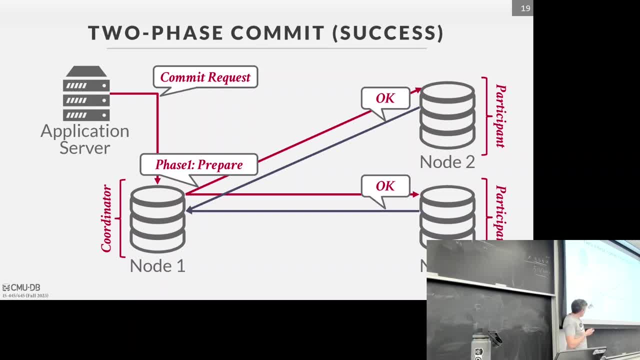 OK, yes, we want to commit this. And then, once you get all the OKs from all the participants, then you go through the second phase and say: OK, guys, go ahead and commit. You send that message to them. They come back with OK. 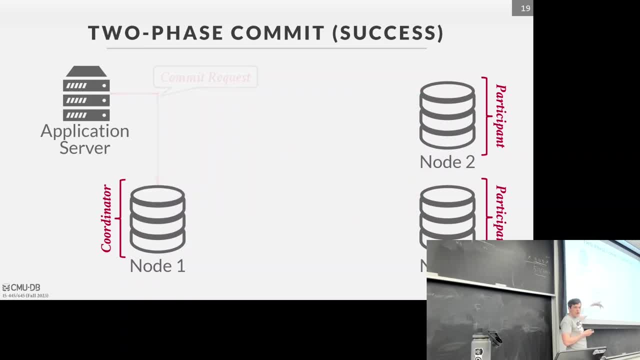 And once you get all of them from the participants, then you're allowed to go and tell the application that this transaction has been committed. Now, what I'm not showing here is that on every node we're actually recording in our write-ahead log. 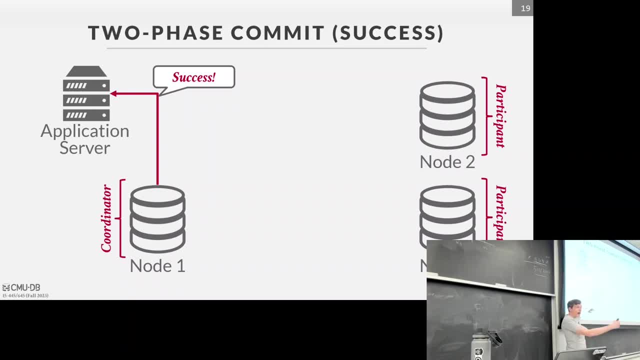 here's all the messages that we got and here's our response to them, And we flush that to disk So that way, if there's a crash and we come back, the node can look on the log and say: well, I was involved in this transaction. 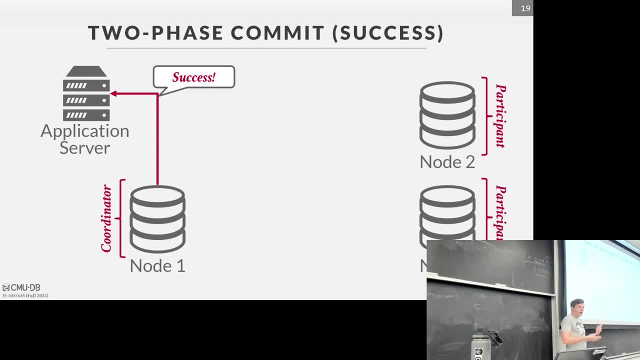 So it at least knows about it and it knows that it voted a certain way. So again, if there's node failure, we can come back and reason about what was the state of the system while we were committing transactions at the time of the failure. 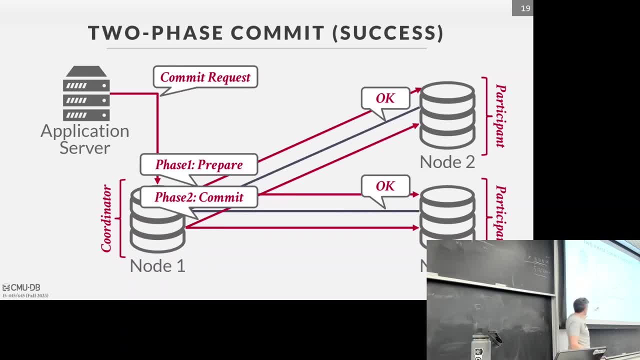 So another key thing about a two-phase commit is that we have to wait for all the OKs to come back from all the participants before we enter the next phase or before we tell the outside world our transaction is committed. That's going to be different than Paxos. 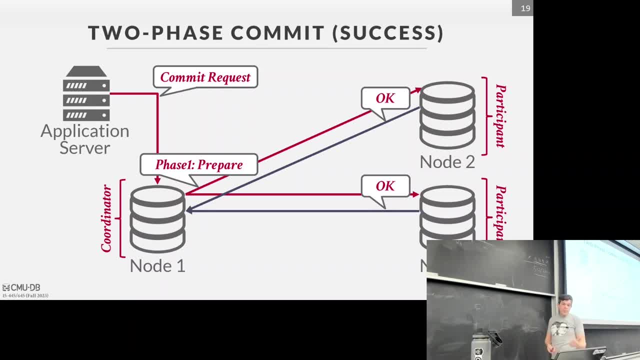 Paxos has to wait for a majority. Raft as well- And I'll talk about this in a second But basically two-phase commit- is a generative case of Paxos, But it has this liveness issue where any one node can take the whole thing down because you're waiting for it. 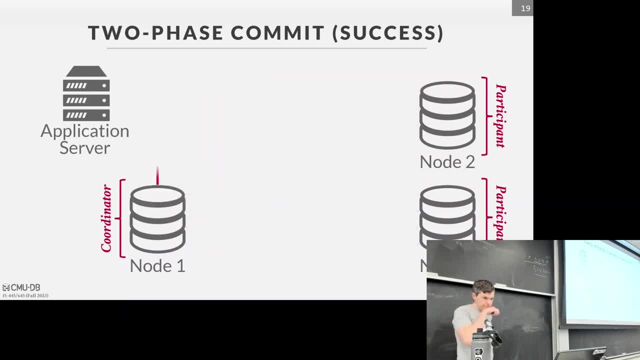 until you time out, So this is a success. For abort, say, the application server says a commit request, We send the prepare message out to everyone. One of them, for whatever reason, we don't care, we don't know why- comes back and says abort. 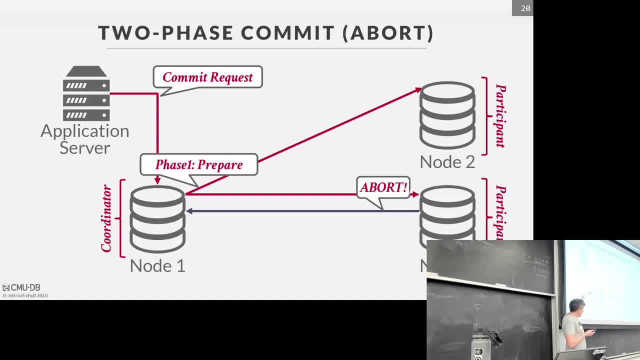 And if one participant in the network says we want to abort this transaction, then immediately we can tell the outside world that our transaction has aborted And then we enter the abort phase and we send all the abort messages to everyone, Even though one node might have said, oh yeah. 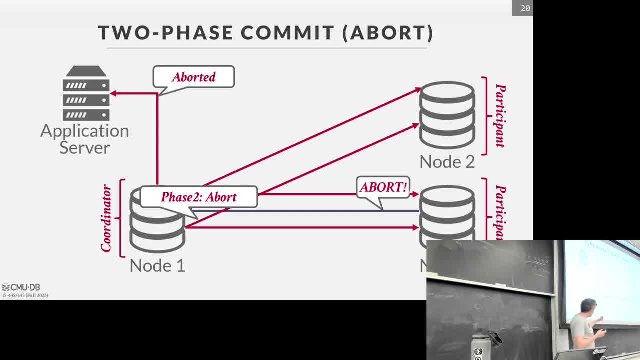 I really want to commit this transaction. I love it or whatever. If we get one abort, we have to kill the whole thing. If the coordinator tells us we have to fail, we have to fail, Right, And then they send back their acknowledgement. 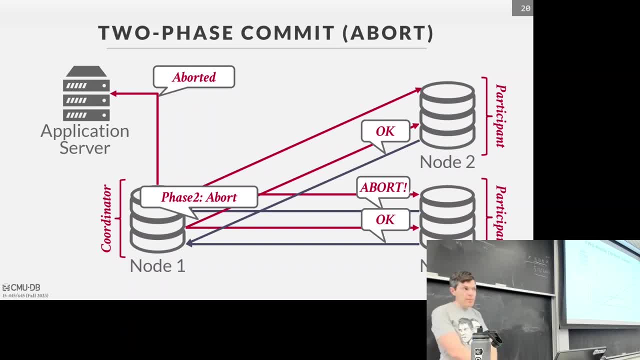 and we log all of this. OK, Pretty simple, right? Yes, So is this for active-active only? So the question is: is this for active-active? Why would it be only for active-active? Because we're OK, so we're. 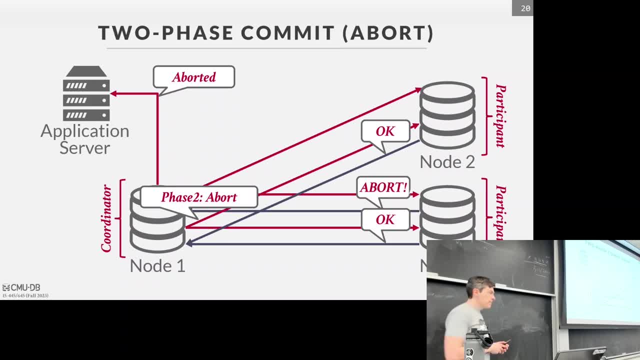 checking the other nodes. if it's OK, Does that imply the other nodes are running the query? The statement is: because we're checking the other nodes when it's OK to commit, does that assume they're running the other query? It doesn't matter. 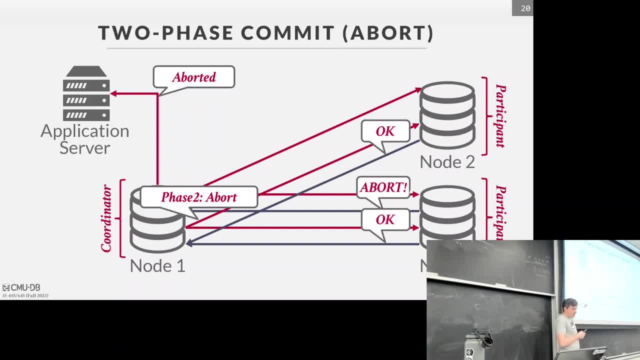 You have to have someone be the coordinator. Someone has to say, OK guys, we're committing, It doesn't matter how node and 2 got propagated with the updates- Active-passive, active-active, it doesn't matter. OK? so I guess, in what case does it send abort then? 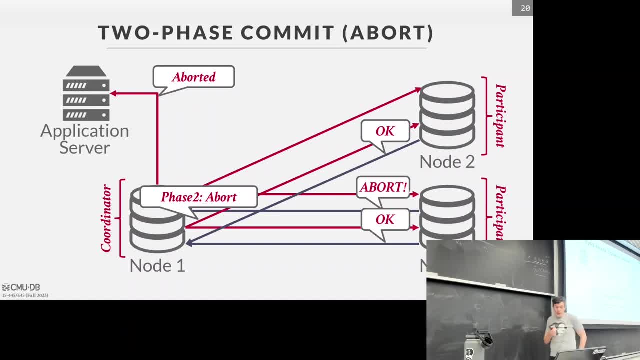 if they're only propagating updates. So the question is: in what case does it send abort? So there could be another coordinator committing another transaction and node 3 is involved in it And for whatever reason, it can commit that guy's transaction. 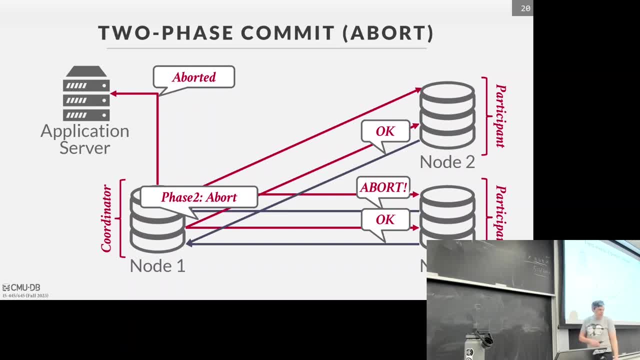 OK, It's a transaction, but not this one. Yes, Are the participants limited to replicas? Question: your statement is: participants are not limited to replicas, correct? yes, So it could be multi-home, the multi-primary. It's just again when a transaction commits. 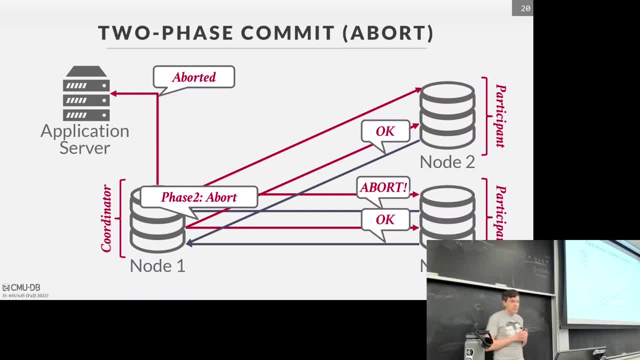 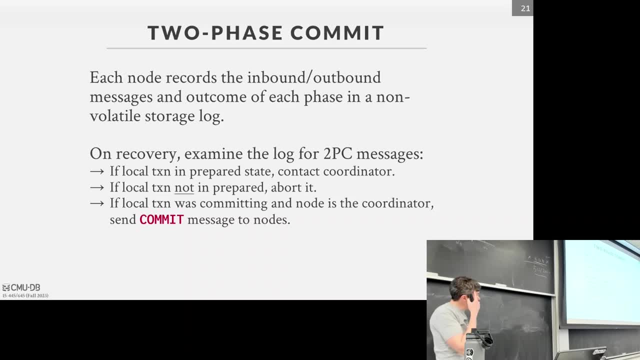 someone has to be in charge, OK. So, as I said, OK, All the inbound and outbound messages we have to store on disk and we have to flush them, like the redhead log, And then when we crash, we come back. 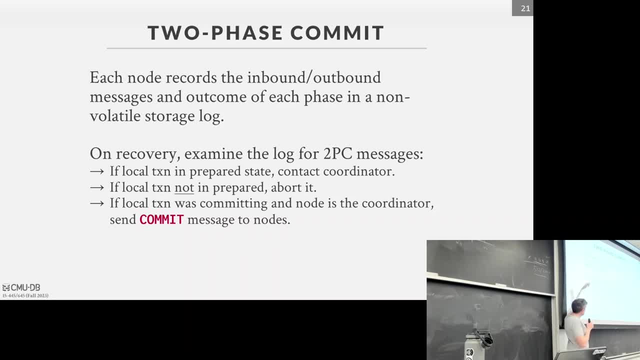 If we see that, if we could look at our log and we see that we were in this prepared state, meaning like we got a request to prepare the transaction and we said, yeah, let's go ahead and prepare it, but then we didn't see whether the vote was successful or not. 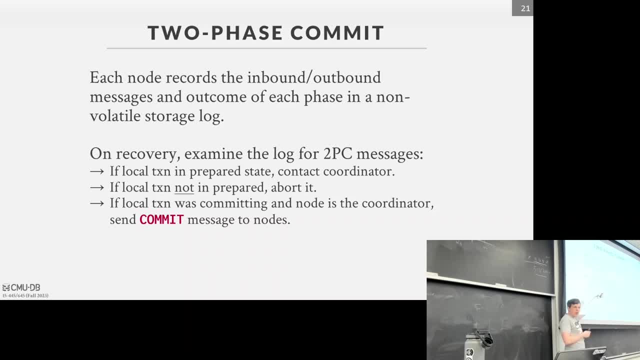 then when the node comes back, it contacts the coordinator to get the updates for the log. I forgot what it missed. If the transaction was not in the prepared state, then we assume that it was aborted, Because if I was involved in the transaction on our two-phase- 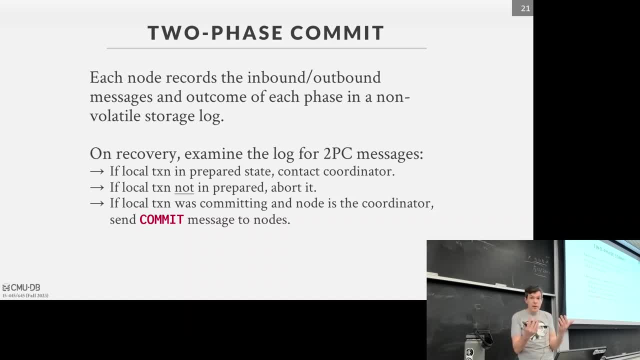 commit and then I crashed. clearly it couldn't have committed, So I'm going to correctly assume that it was aborted. If the transaction was committing and the node that fails is the coordinator, then when I come back up I just send out again, hey guys. 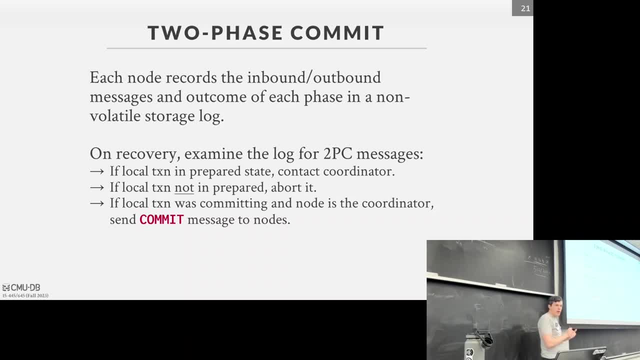 you may have missed this, But I'm pretty sure you were supposed to get this. This transaction was committed. Of course, now again the other nodes have to wait for that coordinator to come back up and come back online, Or at some point there'll be a timeout. 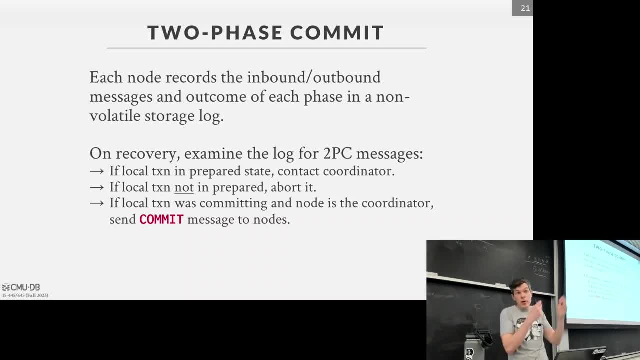 And they say, oh well, that coordinator's dead, He's never coming back, This transaction's aborted. But again, one node going down can take down the whole thing. So, all right, what happens if the coordinator, if it, crashes? I've already said this. 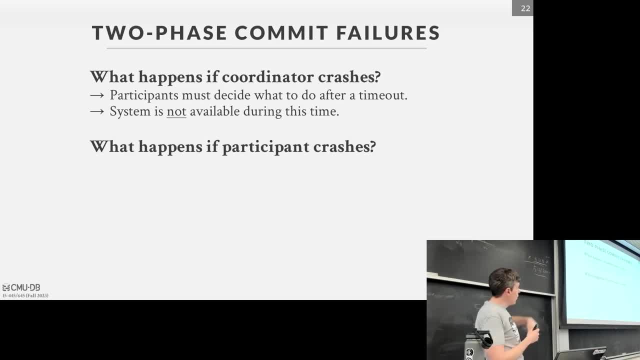 they have to decide what to do after a timeout. And again, the system is not available during this time, And available means I can't take any new queries. I could take read queries, if I'm OK for things being a little loosey goosey, if you. 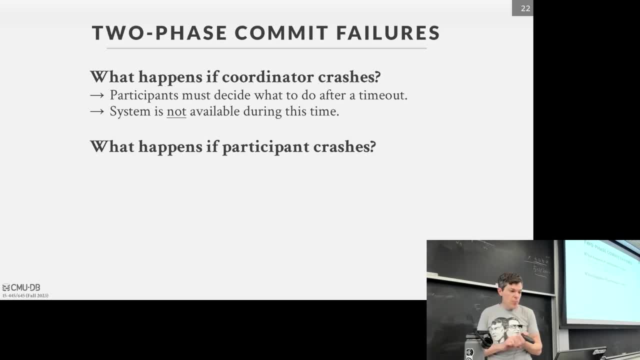 don't want that strong consistency guarantee, But I can't take any writes because I can't propagate those writes until I find out what the transaction before me actually did. And then, if a participant crashes, the coordinators are going to assume that it just. 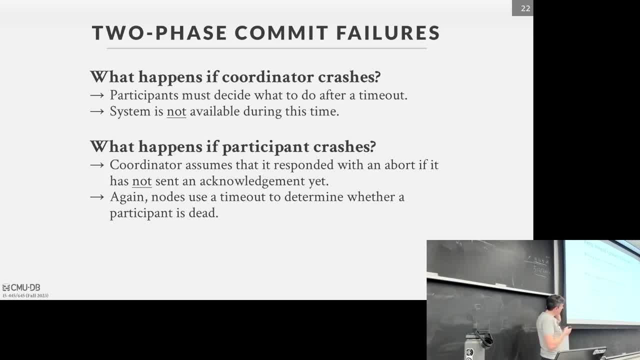 hasn't responded and it's going to be abort, And then we just timeout and say, OK, this guy is dead, And then we just abort the transaction. So there are two optimizations we can do in two-phase commit. The first is called early prepared voting. 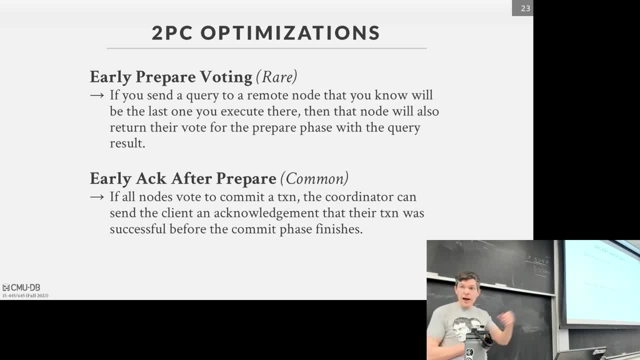 which is actually very rare, And you can only do this with the active-active approach I talked about before and with stored procedures. Yeah, I think that's true. You could do it with the JDBC, but the wire protocol of database systems doesn't support this technique. 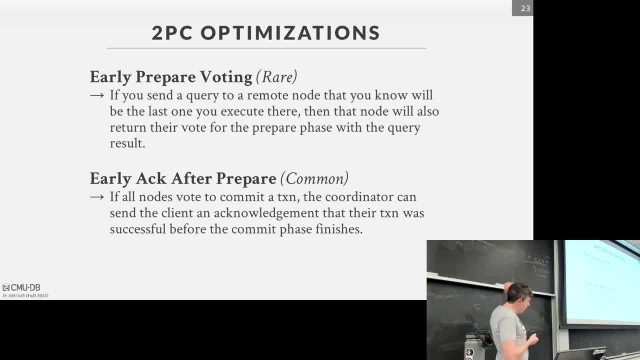 But you can do this, Some systems can do this if you do stored procedures, And then the one that's more common is early acknowledgment after prepare. So early prepared voting is if I'm sending a query request to another node, and I know this is the last time. 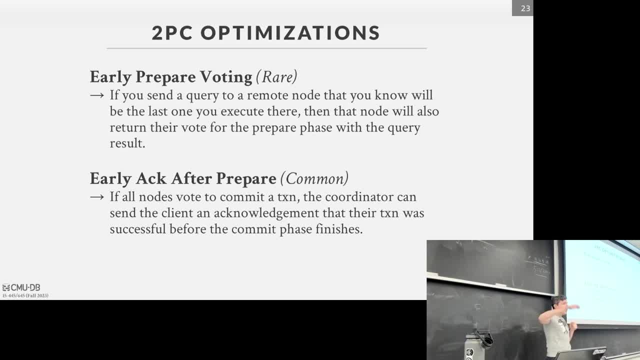 the last query I'm ever going to execute on that node for this transaction. then I piggyback on my message and say, hey, execute this query. And oh, by the way, I'm going to come in here, I'm going to commit pretty soon. 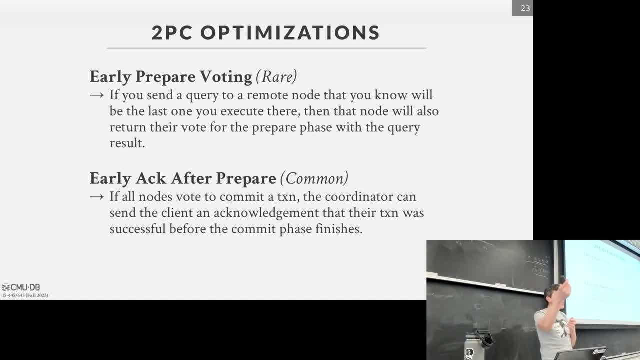 I'm never going to come back and ask you to run another query, So go tell me what your vote's going to be for two-phase commit, So you get the query response back and actually the vote on the prepare phase all in one round trip. 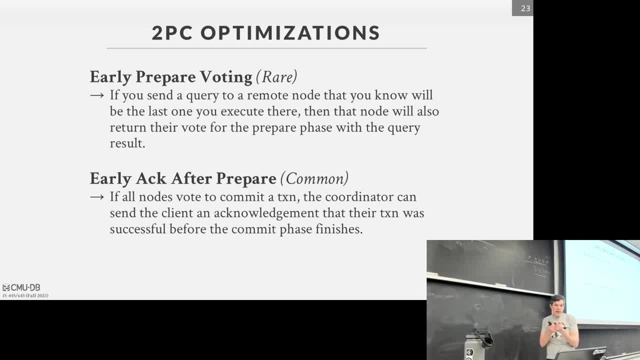 Early acknowledgment after a prepare is basically: if I get the acknowledgment on the coordinator from all of the participants that this transaction is going to commit, then I don't wait until I get the acknowledgments from the commit phase. I immediately send back. I send back the commit message to the application. 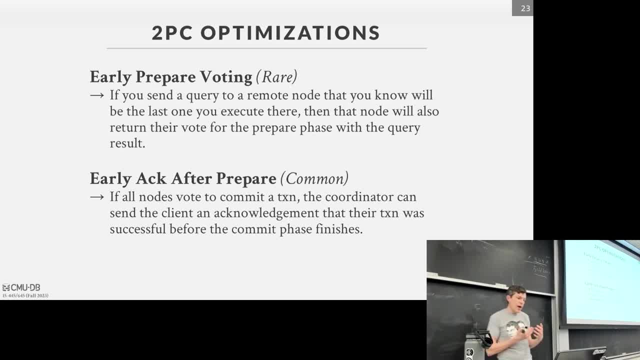 the acknowledgment back to the application, Because at that point I assume that if there's a crash and I come back, then the coordinator or the nodes will look in the log and say: OK, we all agreed to commit this transaction, So let's go ahead and actually apply the change. 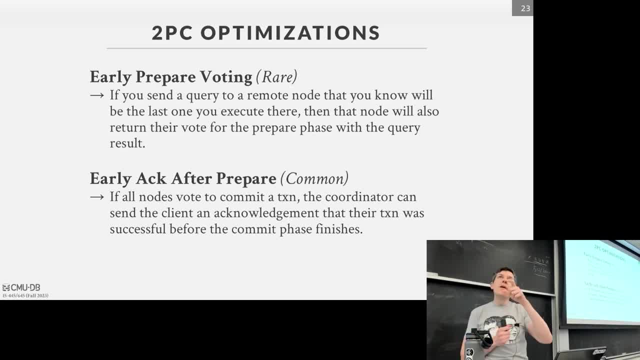 So there's a small window where, like sorry, there is not a window where you could crash and lose data, but it will make recovery a little bit longer. So it looks like this, right, So I get my commit request. I do my prepare phase. 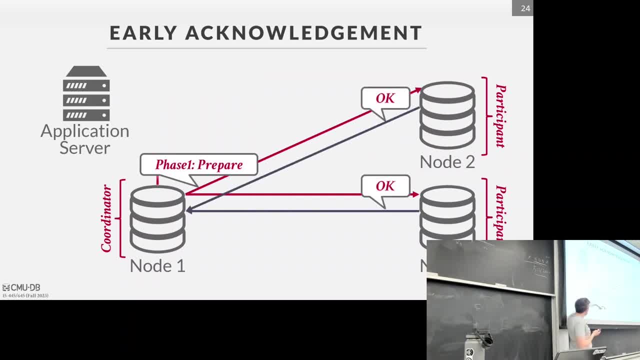 They all come back and say: OK, go ahead and commit, And then immediately, once I get back all the OKs I can send back to the success And then I still then have to do the commit phase and get that round trip. 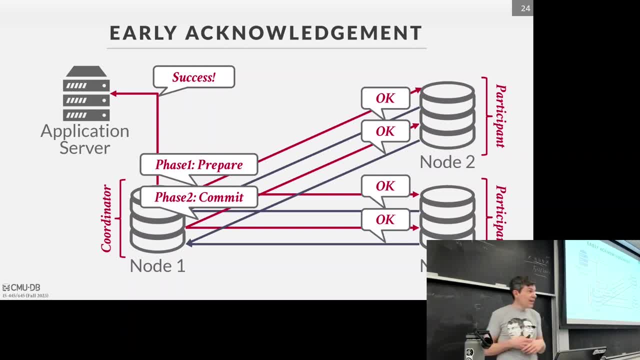 Again, all of this is written to the log, which not everyone always does or not everyone always flushes it, But most systems doing two-phase commit are going to do this simple optimization Because the window, the failure window, is pretty small. 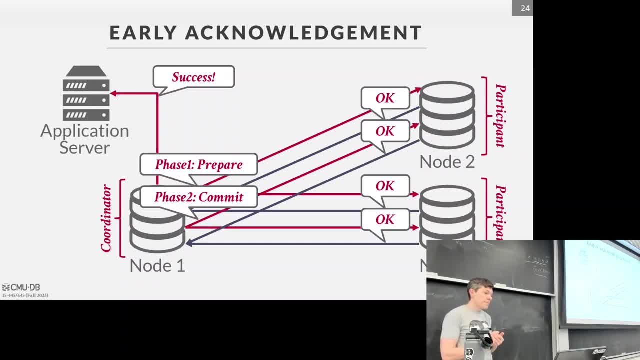 Yes, Is it still important to do two-phase if we're doing asynchronous? This question is: do we still need to do two-phase commit if we're doing asynchronous commits? You should, because you want everyone to say: OK, we all agree that this is the update that happened. 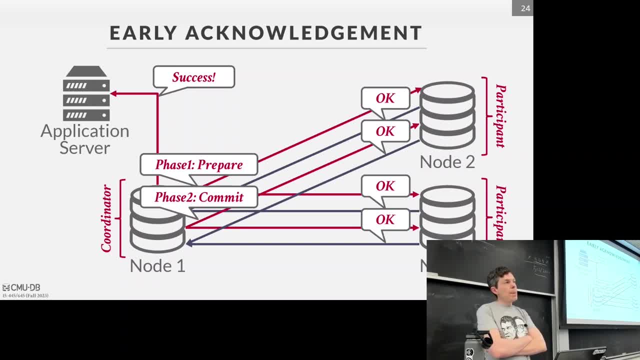 You don't have to, though It makes you'd have to do more work on recovery, But you could potentially not use two-phase commit. I think that's true. yes, Yeah, I think a lot of the NoSQL systems. 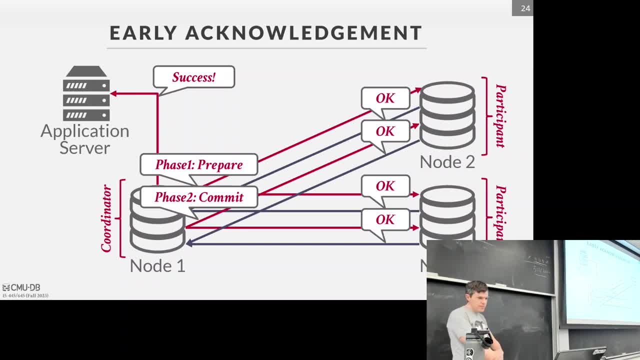 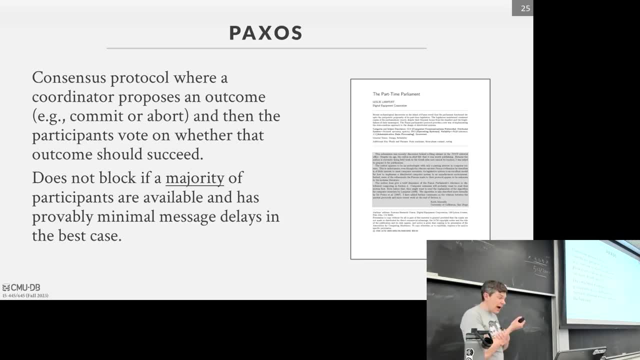 when they did that propagation they weren't using two-phase commit. So Paxos is, as I said is, considered a superset to two-phase commit And this was the- I think this was the first correct protocol that was pursued. I mean provedly resilient in the face. 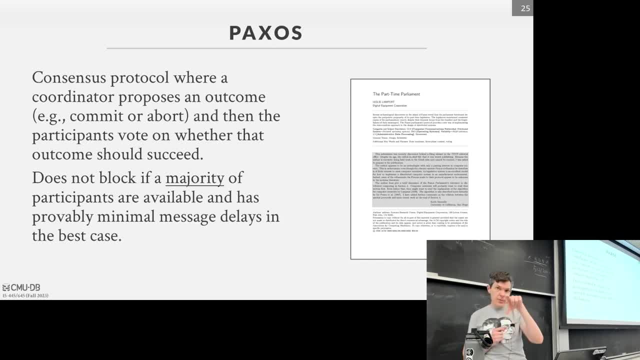 of asynchronous networks, But again, it wasn't the first one that actually could do this. Vue stamp replication came before it, And so the idea is basically that we're going to send out the votes like before, but instead of having all the participants. 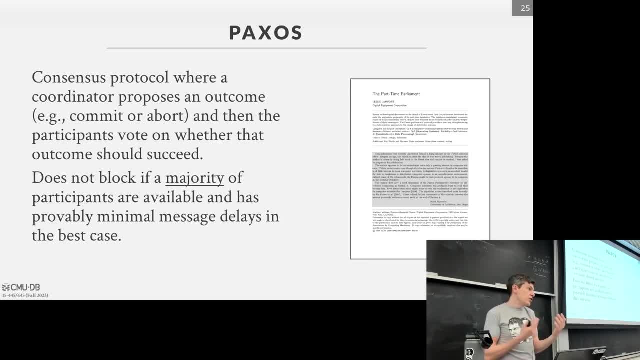 come back and acknowledge that current action prep commit. you just need a majority. And then for the ones that are in the minority right, I say OK, they basically are treated as as failures or fail failing, and they have to basically crash, pseudo crash, and then replay the log to get them back up. this 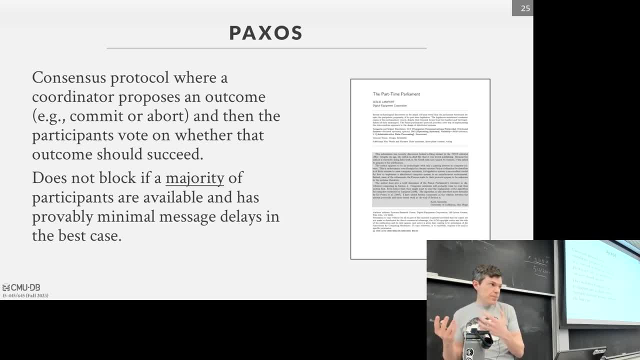 day up to up to the correct state- and this is going back to my same before this- why we don't care about Byzantine fault tolerance in in the real world. well, this world, because it's not like someone's gonna vote no, because they want to right when everyone else is going to commit. there's something you. 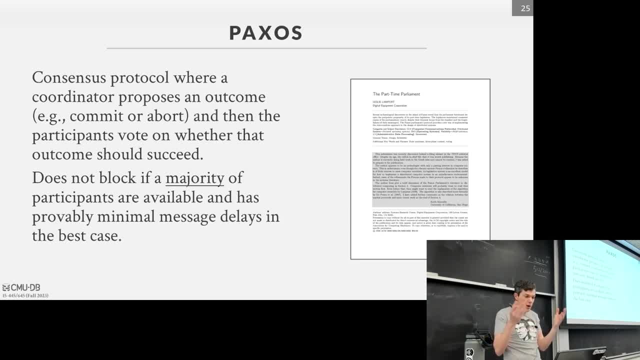 know really wrong with it or the network, and but when it comes back it can get back up, up to up to date, right, assuming that, you know, and there's no massive hardware failures. so the the original Paxos paper, I think. is there a date on this? yeah, 1998. um, the Lamport actually wrote the paper in 89, but he 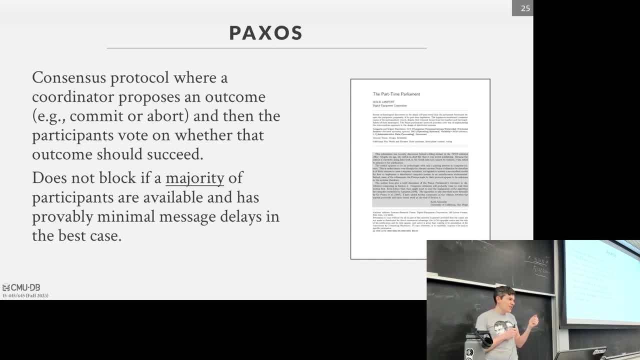 actually, who here has ever read the Paxos paper one, two. it's a wild read, right, yeah, yeah. so it's crazy, I it's. basically he's trying to be very illustrative and and and not poetic, but he was trying to. instead of saying: here's the protocol, like it does this, this and this and this he describes it. 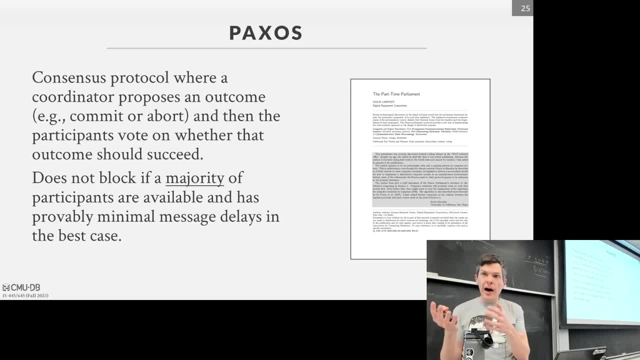 as if he's like archaeologists finding this ancient Greek tribe on the island of Paxos and how they would do voting by put throwing tablets in a hole and then coming back later and to read them right like it's. it's just, I mean, it's amusing. 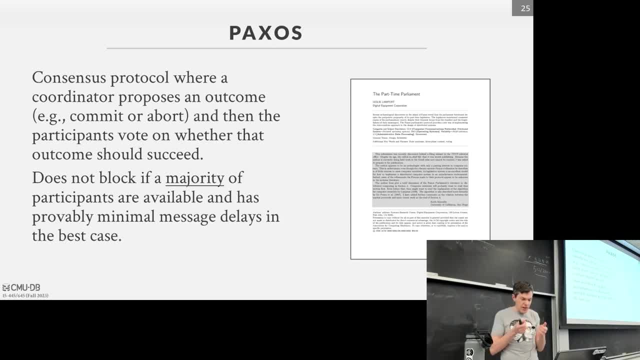 but, like, if you really try to read and understand what the hell is actually trying to do, you can't. and so the story goes is that if you go to- actually if you go to- Leslie Lamport's website and you go look at his bibliography, which is: 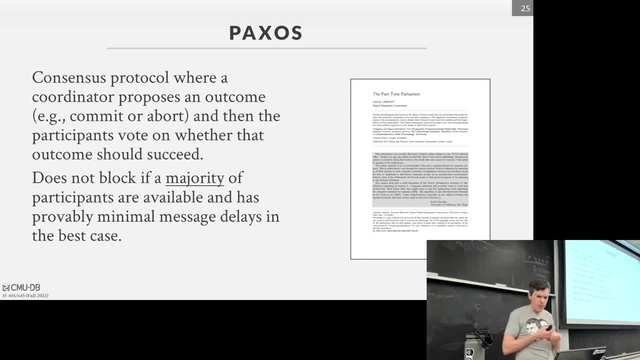 kind of cool he lists like for every single paper, at least for the major ones. he lists like what he was doing in his daily life when he wrote the paper, like what he was eating, who he's dating and so forth. right, and so he talks about in. 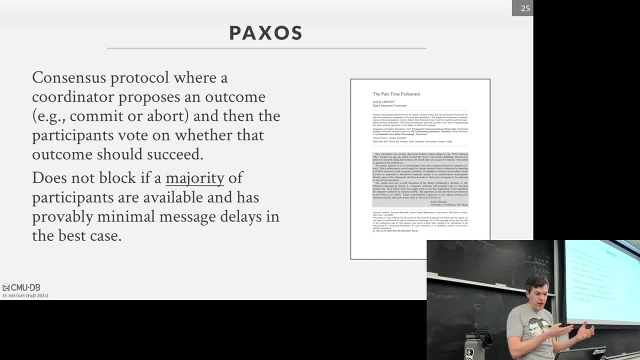 the Paxos paper when he submitted, with this Greek archaeology story inside of it. it got rejected and he says like, oh, the reviewers were stupid because, like, they couldn't appreciate my genius, or whatever. and so when I was in grad school, I took a distributed systems course and I presented the Paxos paper and I 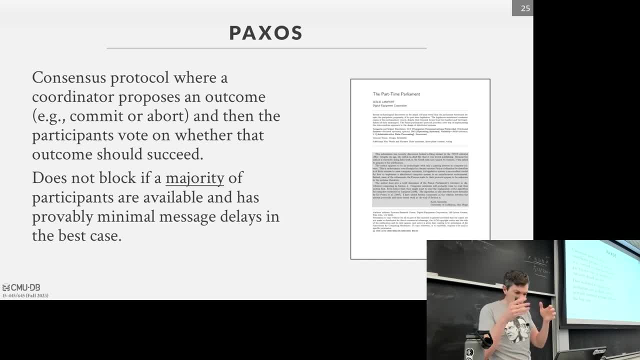 started going on about like, oh yeah, this paper is brilliant, and like the reviewers were super, you know they were stupid for rejecting his. you know he was a genius. turns out, though, the professor teaching- and this was back at Brown is- was Maurice Hurley. he used to be here at CMU and he he's like, yeah, actually was one of the. 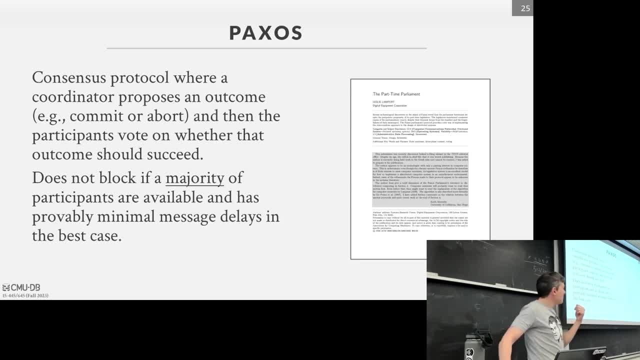 reviewers on this paper and the story goes, is that they were okay with what he says. they were okay with all the Greek stuff. these wanted him to have an add, an appendix with like I you know, with an algorithm and like a proof to showing that what the thing actually was. and 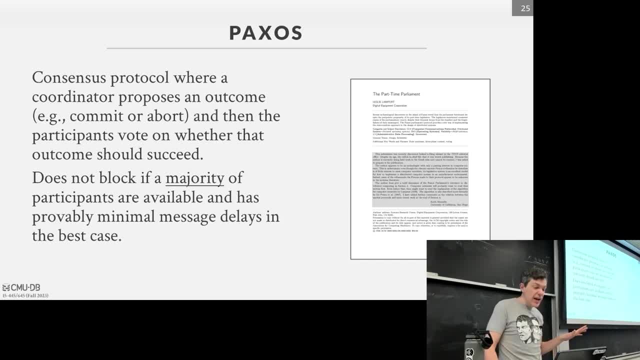 Leslie Lamport was apparently super stubborn, didn't want to change anything in the paper because he thought was perfect as is, so got rejected. they put it in his filing cabinet or put it in a shelf and didn't do anything with it for like ten years. and then over the 90s, people started publishing papers that. 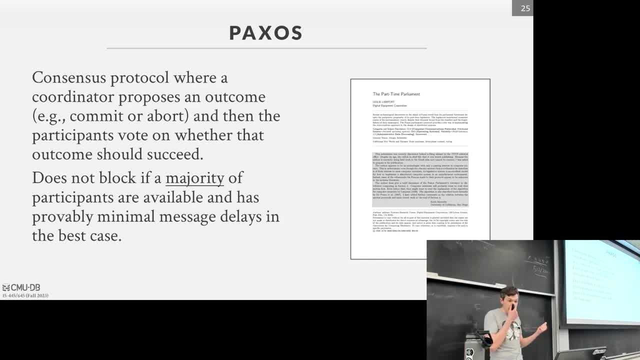 sort of like dancing around the problem that he already saw back in 89 he actually was not aware of used in replication, which is came out in 88. but then once, once you saw enough papers trying to kind of barking up the same tree as Paxos, then he put the original Paxos paper out along with another paper. 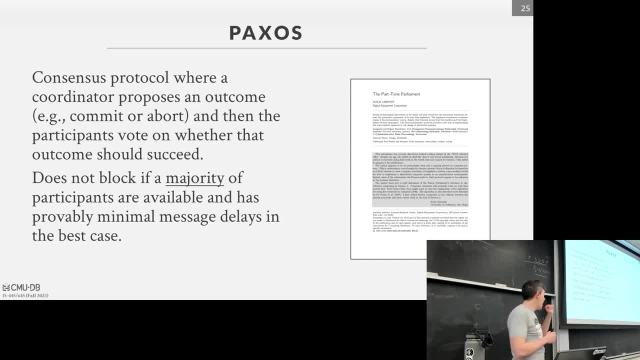 called Paxos made simple, which is not simple, but actually the one paper. if you want to read a Paxos paper, the the Google one, Paxos made live, that's the one that, like for me, clicked. oh okay, now I don't understand what they're doing. 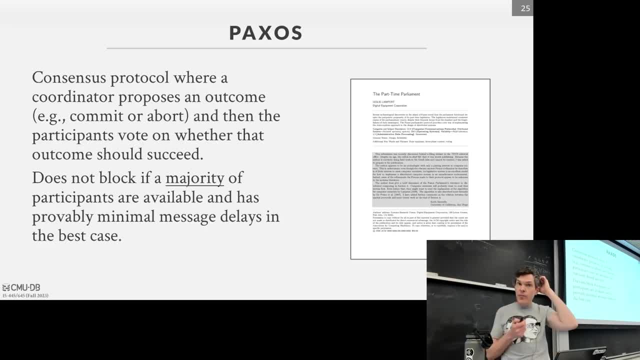 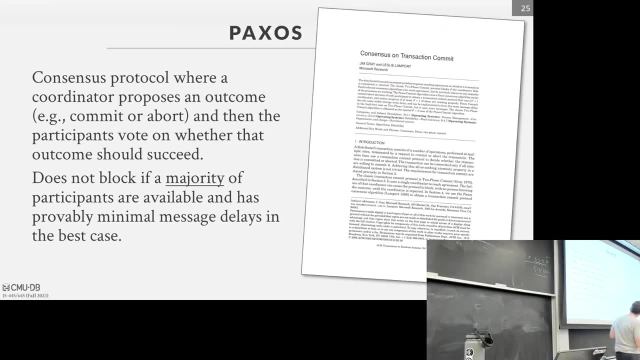 But then once you know that it's actually just a degenerative case of two-phase commit- at least for me coming from the database world- then it makes sense. So there's this paper here- This is 2006- from Jim Gray and Leslie Lamport. 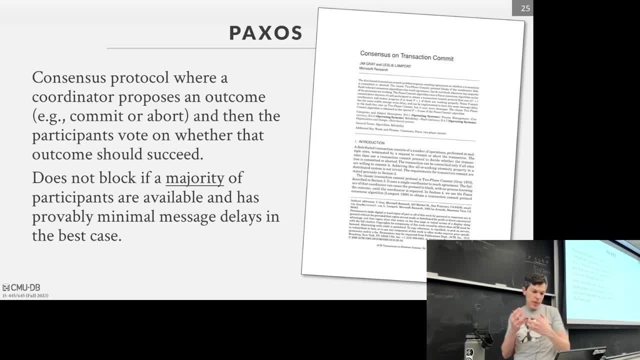 This is right before Jim Gray got lost at sea, where they basically show, they prove, that two-phase commit is a subset of Paxos. So again, and RAF is going to be basically the same idea here, It's just going to have fewer node types. 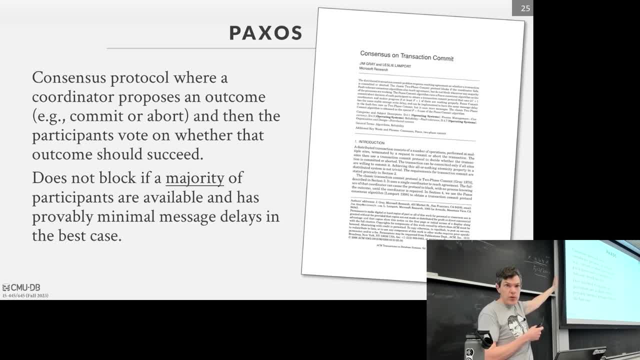 And actually I'm not even going to show this. There's another node type in Paxos called learners. We can ignore that. I don't think anybody does that. The nodes have multiple roles, so it doesn't matter. But again in Paxos, when they do a leader election. 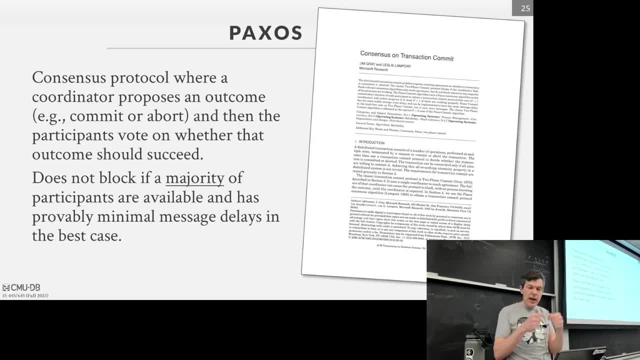 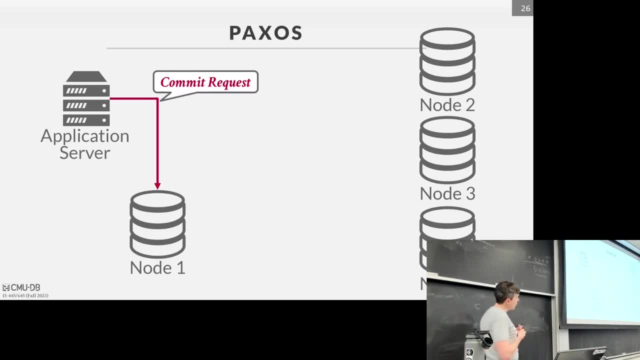 any node can be a leader, But in RAF they choose the ones that have the most updated logs. That's sort of the major distinction. So going back to our example here, now we have three nodes. Our transaction goes ahead and commit. 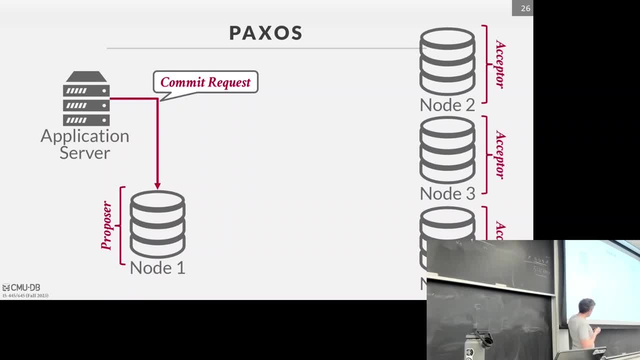 The Paxos. instead of calling them coordinators and participants, they're going to call them proposer And acceptors. again, those are learners. We can ignore that. We send out the propose that we want to commit this transaction. Say this one. node three here goes down for whatever reason. 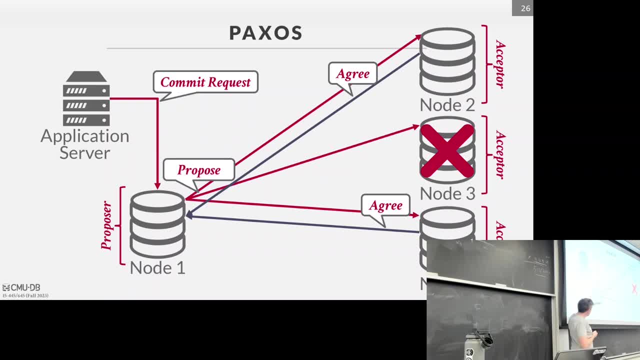 It doesn't matter. And then we get back the agreements from the other two nodes And since we got two out of three of the nodes agreed that we can commit this transaction, this transaction is allowed. Well, we do the commit phase And then the transaction is allowed to commit. 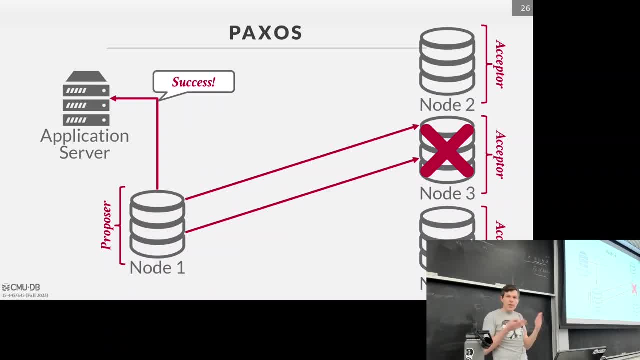 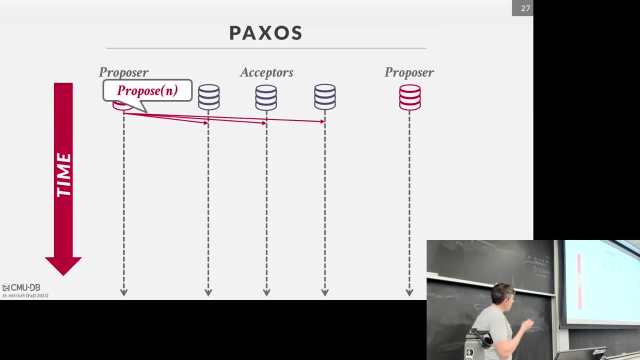 And eventually, when node three comes back up, it can learn about the the changes that it missed. So another way to look at it is often this sort of timeline graph here, Where you have a proposer that says: I want to commit the transaction, you have a timestamp n. 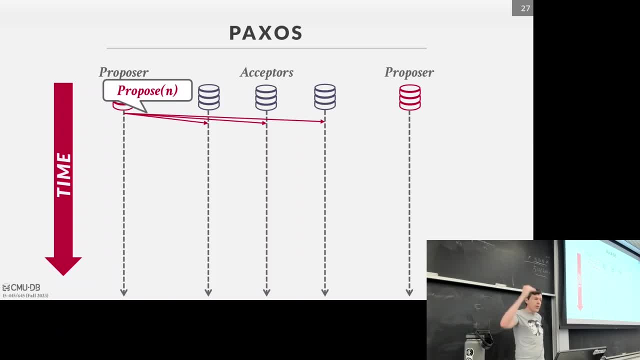 Again. think of the log as just an ordered list. So here's the transaction that I want to commit. So the first guy says I want to commit transaction n. So all the acceptors get that They agree to do it. But during this time another proposer comes along and says: 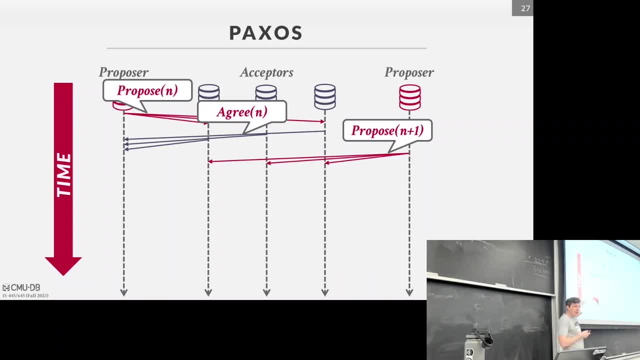 I want to. I propose commit transaction n plus one And then, as soon as the acceptors see a new timestamp value that's greater than anyone's seen in the past, anything that comes after that is automatically rejected. So the log is always sort of moving forward. 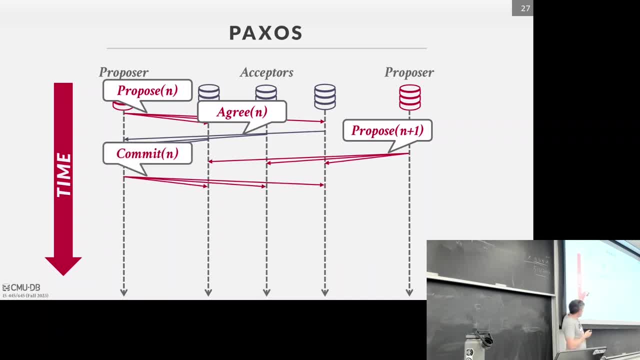 You never move backwards. So now, when this other guy says: I want to go ahead and commit- assuming we're not doing the early acknowledgement optimization- go ahead and commit because these acceptors already saw n, They reject it and say: I can't take n because I've seen n plus one. 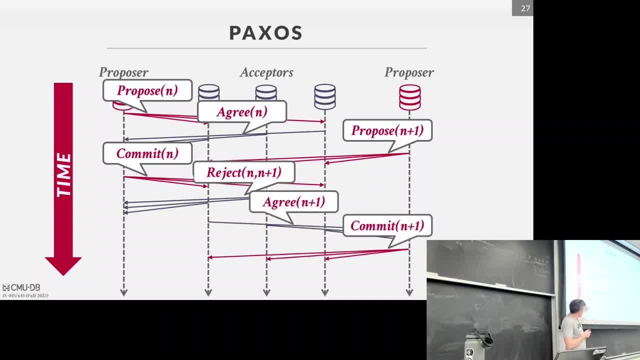 So now they can go ahead and agree to commit n plus one commit that And then this other guy here he can resubmit his request to commit that transaction. So in this world we have multiple proposers proposing to commit transactions. 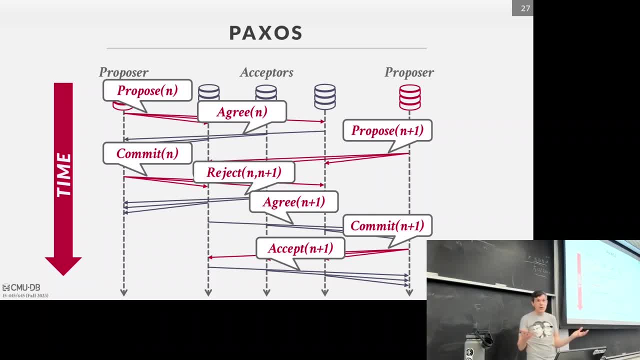 And obviously that's going to be problematic because you're going to have this contention of everyone trying to clobber each other. Yes, In this example, would 2PC actually say it? Because I It looks like, like you said, the difference is in majority. basically, right. 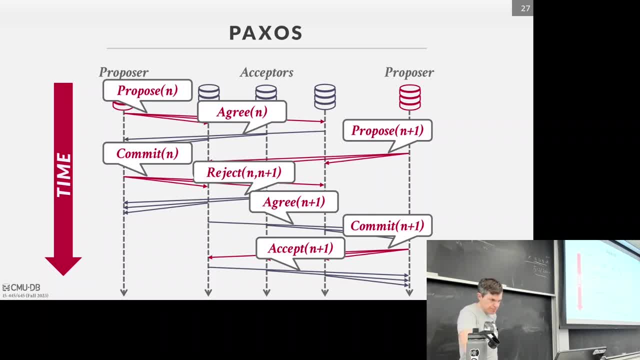 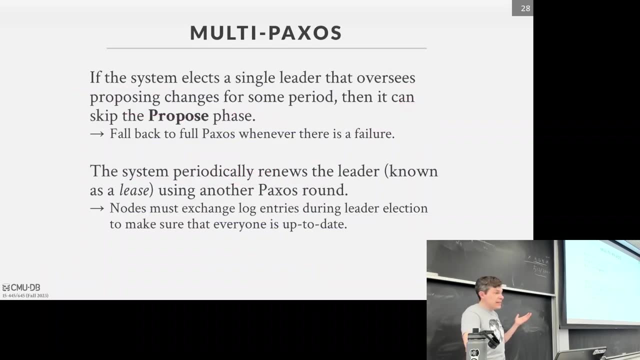 But it looks like here they're all responding at the same time. So the statement is: would 2PC have the same problem if you have multiple coordinators? Yes, So again, the way we're going to handle this is through leases. 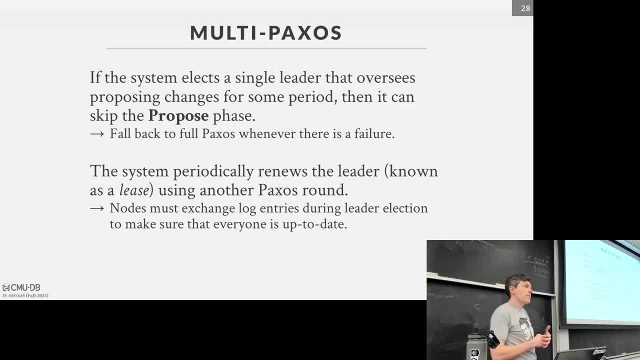 to limit the number of or limit which node can propose commit transactions, Basically, how to anoint Which one's going to be the primary, which one's going to be the coordinator or the proposer for a distributed database system. So this came from a Google paper called Multipaxos. 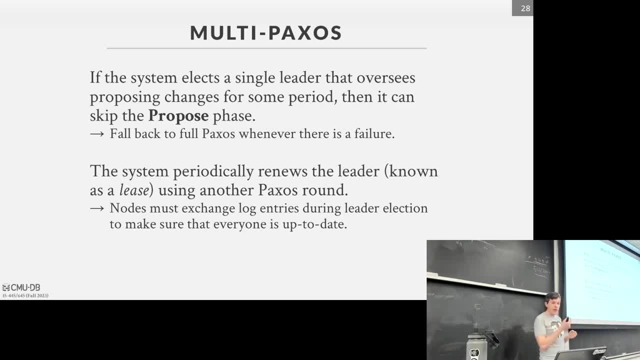 The idea here is that you run leader election every so often to say: okay, this node here is anointed, as the proposer, And then in some cases now you can skip the propose phase, because now the coordinator or the proposer can say: 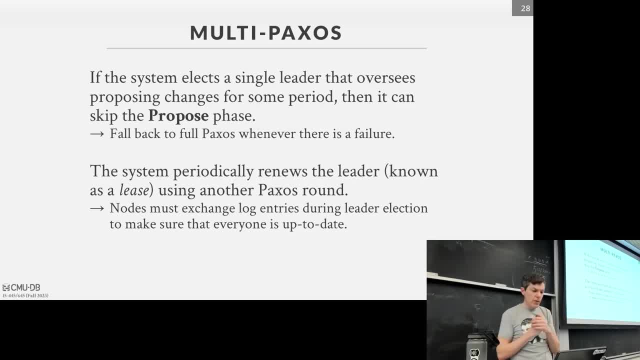 here's the transaction I want to go ahead and commit. Everyone agree that we're all going to commit this right. And then if at any time there's a failure, either, like the node you know, the leader goes down or some node goes down. 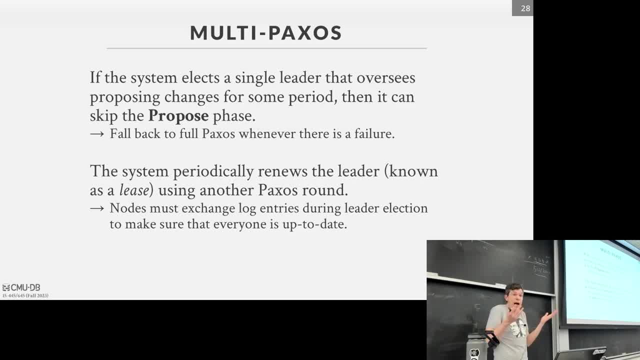 then you just run the leader election all over again, Which is then just running Paxos, right? Because, again, think of the state machine- is here's the order in which transactions commit And, as part of that state machine, here's the 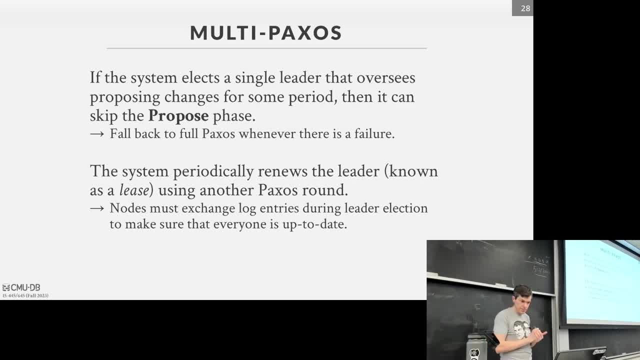 which node is the proposer or the coordinator, right? So you would send heartbeats out between the different nodes to figure out who's actually alive and responding to requests. And if you don't get a heartbeat with a certain amount of time, then you say: 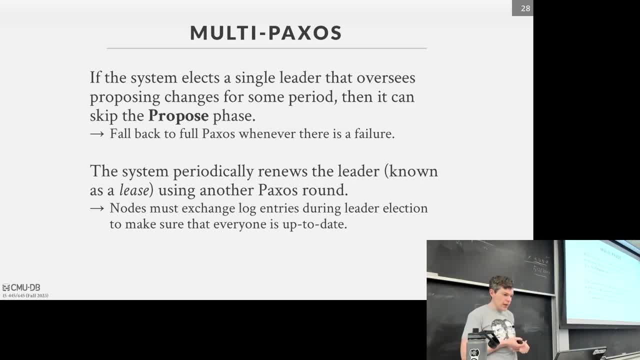 okay, this node is down and rerun leader election, right, And then you set the least time out to be like: okay, every 10 minutes or so, then I automatically run leader election all over again, And it may be the case I'd reelect the same leader, which is ideal. 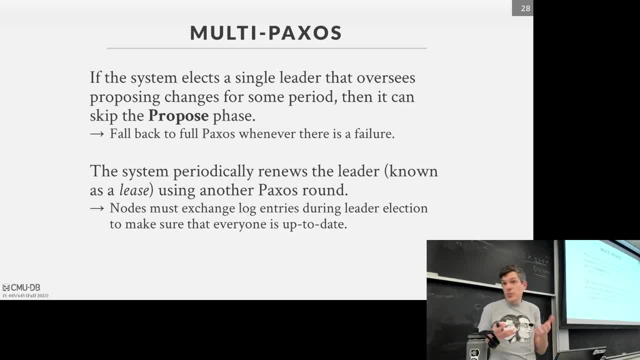 but at least you're running that election over and over again And different systems are going to run that leader election at different time intervals. Spanner runs it every 10 seconds, YugoByte is every like 30 seconds And I think Cockroach. 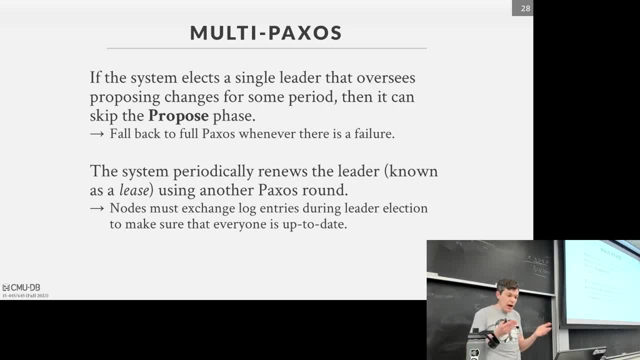 in the source code. it's like every five minutes And again it depends on how reactive you want to be to the, you know, to failures. YugoByte is two seconds. YugoByte is less than Spanner. It's two seconds. 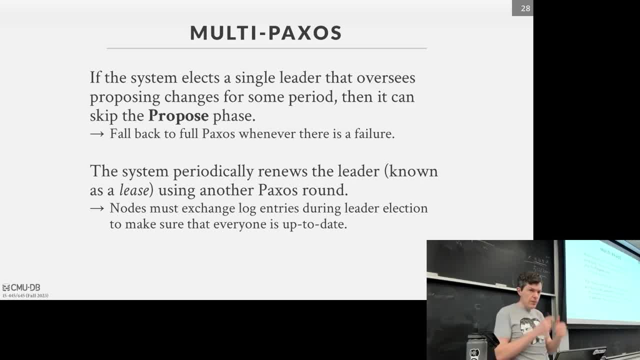 All right. But again, generally this technique is falls under the umbrella called multipaxels. So most people say they're running paxels. They're most often running multipaxels, All right. Again, I've already covered this already. 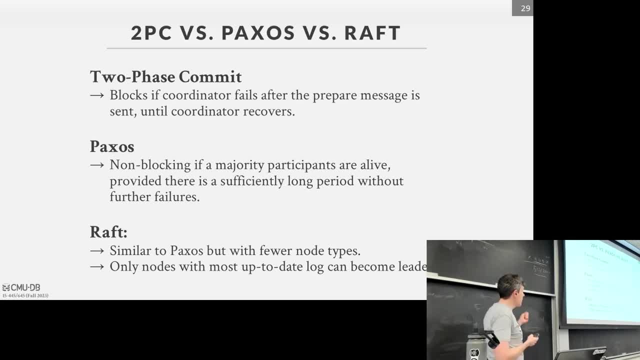 But the main idea is the main difference between two-phase commit, paxos and raft. Is there a two-phase commit that if the coordinator fails or any node fails, we have to block until the coordinator comes back In paxos, as long as the majority of our participants are alive? 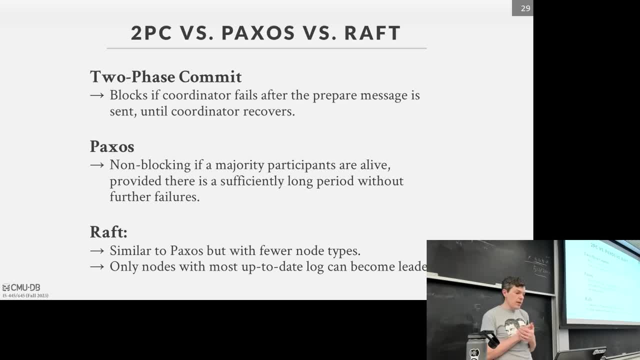 and we've waited long enough to make sure that there's no further failures. then we can go ahead and commit And raft, as I said, is basically the same thing: Fewer node roles, And when you do a leader election you choose the ones that have the most updated logs. 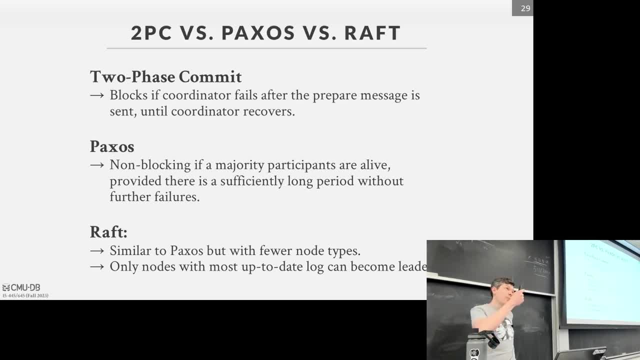 Yes, What were the node types for paxos? Paxos has proposers, acceptors, and then there's learners, which are just sort of downstream from the acceptors to say, hey, here's the changes, here's what we just committed. 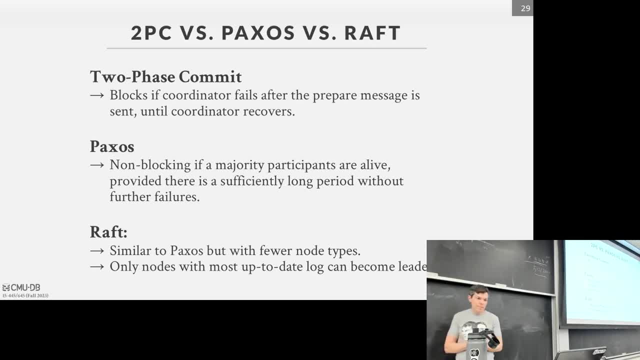 We can ignore that. Okay, So most of the modern distributed data systems are going to be running paxos or raft. Raft is probably way more common than paxos just because, when it came out in 2013,, a bunch of people took the protocol. 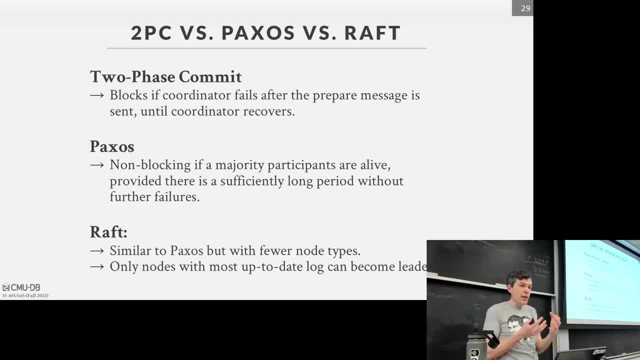 and they re-implemented it in different languages. So for a long time there wasn't a lib paxos you could download and just like. oh, let me put this in my distributed database. But in raft there was a bunch of correct implementations in Rust. 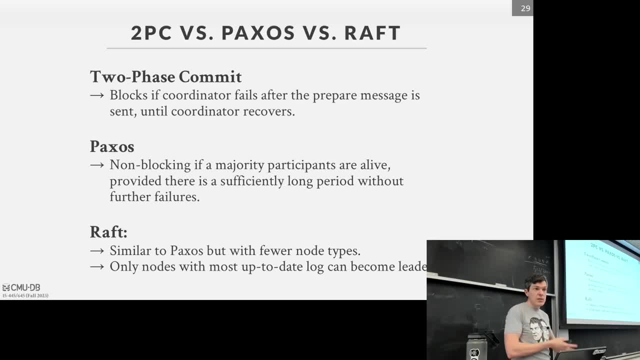 or Rust wasn't around, but in Go and Python and C++ there were a bunch of libraries that you could just plop in and get raft consensus out of that. So I think that helped evangelize it a bit more. Yes, What's the difference between multi-paxos and raft? 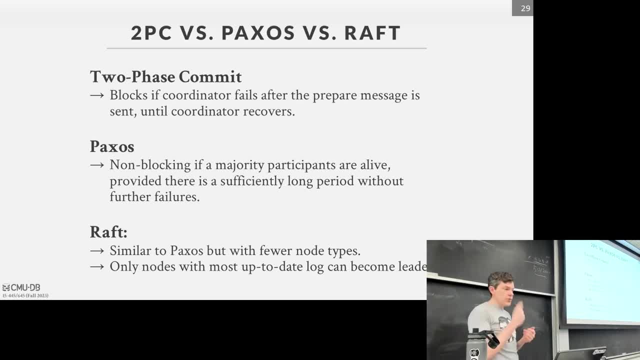 The question is: what's the difference between multi-paxos and raft? Same thing. How is it You run leader election? Okay, but what's the difference? like Multi-paxos is like 2004,, 2005-ish. 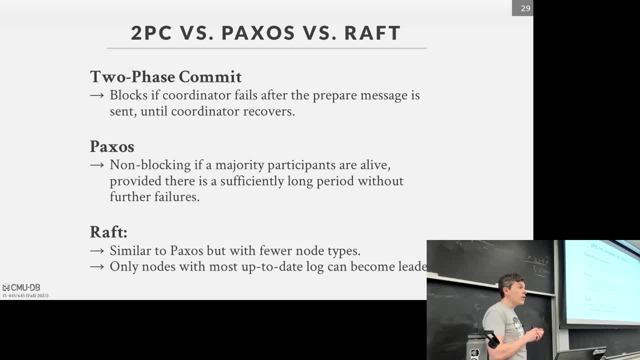 Then what's the difference between them? I mean, the question is, what did raft invent? Yeah, what's the difference? Oh, so again they don't have. raft is meant to be a more understandable version of paxos, right. 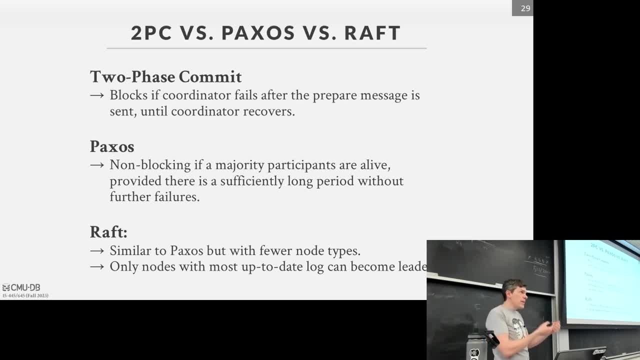 At a high level. they're the same right, But in terms of implementation you don't have to have a these learners, either participants or you know, or proposers, so there's only two node types. When you do a leader election, then you have 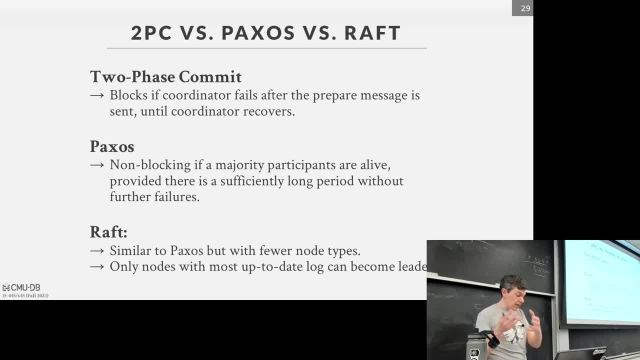 you choose the one that has the most up-to-date log versus paxos. anybody can be the leader And I think paxos had- or sorry- in raft. there's explicit like timeouts for heartbeats and things like that. 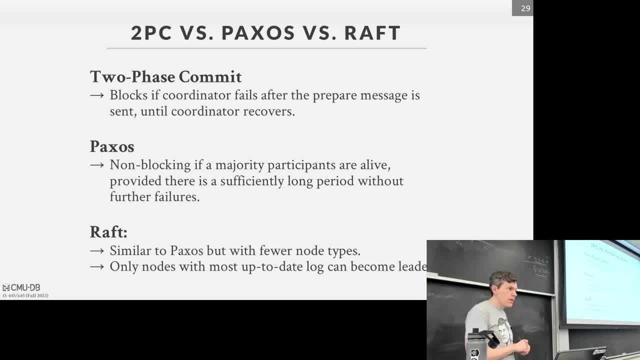 where in paxos people add them, but I don't think the original protocol talks about those things. Yes, So I'm a little confused on multi-paxos versus paxos. Is the main difference? like what's the difference? 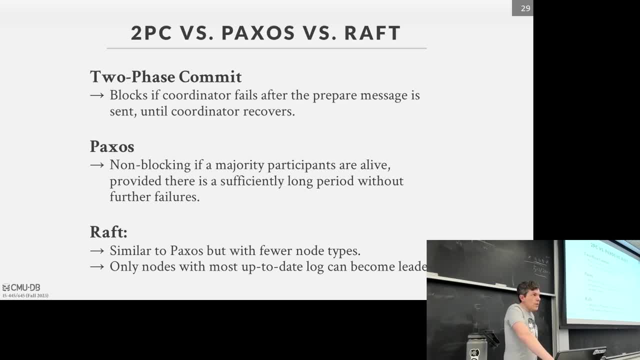 That multi-paxos will periodically shuffle where the leader is. The main difference in multi-paxos, yes, but in paxos anybody can be. anybody can be a proposer, anybody can be a leader to propose changes, to update. 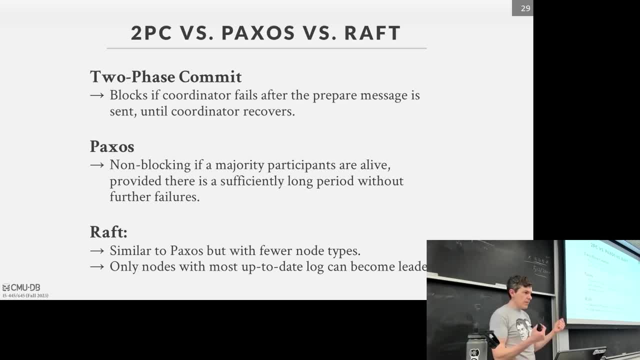 Oh, I see, Yeah, Okay, so multi-paxos. so it elects one and then all the changes get sent there to be coordinated. Yes, Because otherwise anybody proposing, and you're just like you know, you just clobber each other and so you have to do. 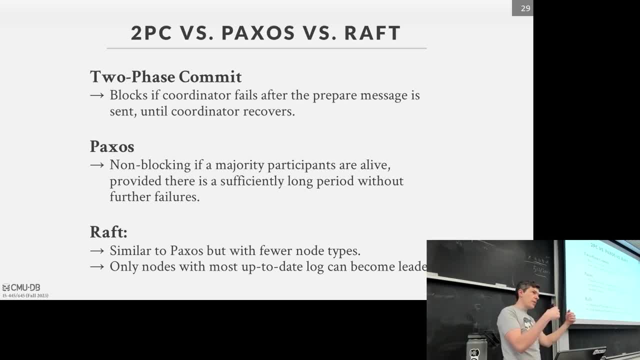 like back off, just like okay. why multi-paxos? you know you have to like my transaction. I got overwritten, I couldn't commit it, so maybe wait a certain amount of time and submit another one. 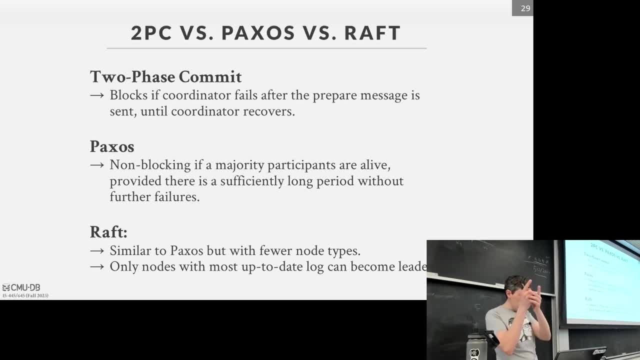 So, instead of like that back and forth to say, okay, you're the leader, everything goes to you and you don't worry about conflicting proposals coming in, Okay, Yes, So the difference is just that one proposer is the leader. 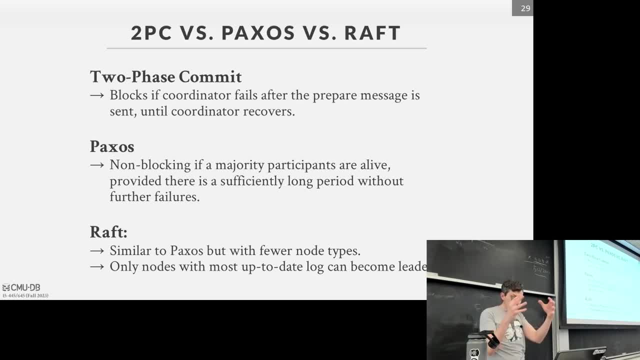 And you technically have one proposer within some boundary, in multi-paxos, yes, And whether that boundary is like a rack of machines or like a data center, it depends on the implementation. All right, Let's finish up. 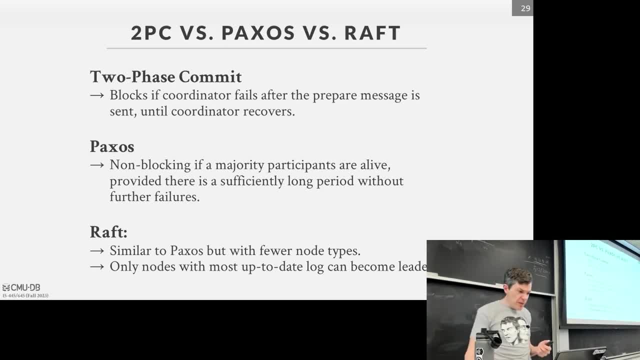 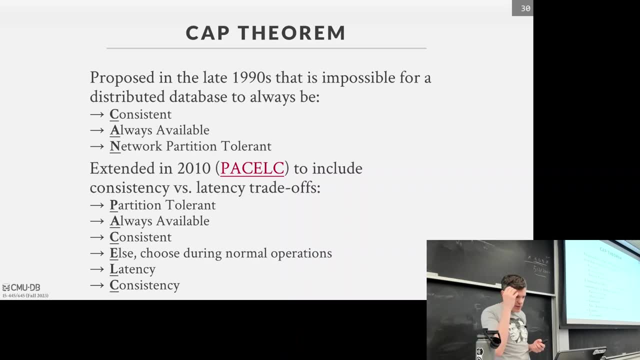 So CAP theorem. So this was the hot thing in distributed systems, the buzzword everyone used in the 2000s to describe their distributed database systems, And it was a way to characterize what the system could handle in the face of failures, right? 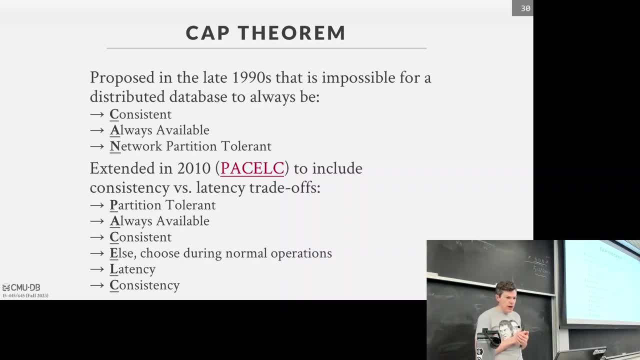 So the CAP theorem, the C, is the cap theorem. It's the same thing, It's consistent. It's basically strong and consistent. The A is always available, So if there's a failure or there's a network partition, you can still run any possible. 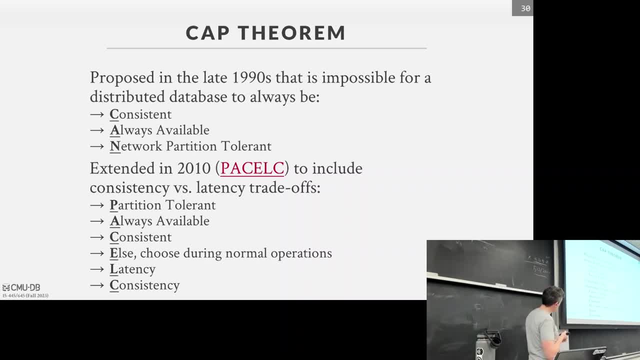 query And that's sort of tied to the network partition tolerance. What happens when there's a network partition? Can you handle updates in that environment? So it was proven to be correct the way to describe systems. The idea is like you can pick two out of three, right? 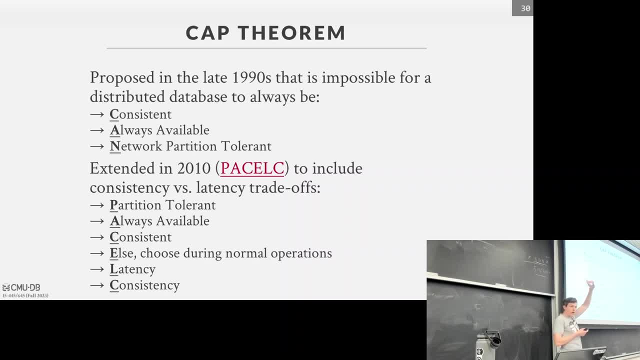 The way to think of like a boyfriend or girlfriend, like, are they good-looking, crazy or smart? Pick two out of three right. Same thing for your distributed database. And so this is proven to be correct. But a very important aspect of this is that the CAP theorem describes what happens if 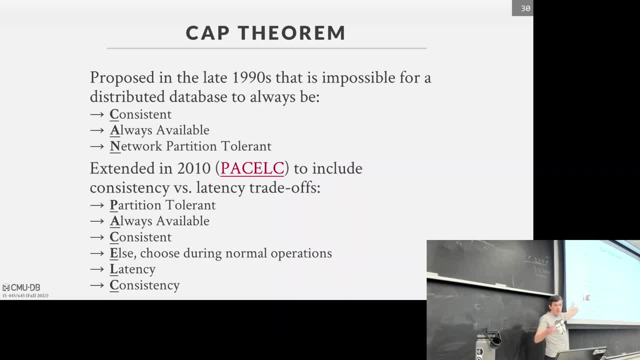 there's a failure, But most of the times there isn't a failure, right. So what happens when you're running no operations? So it got extended by Dana Boddy, who did a lot of the early column store stuff at MIT and is now a professor at Maryland. 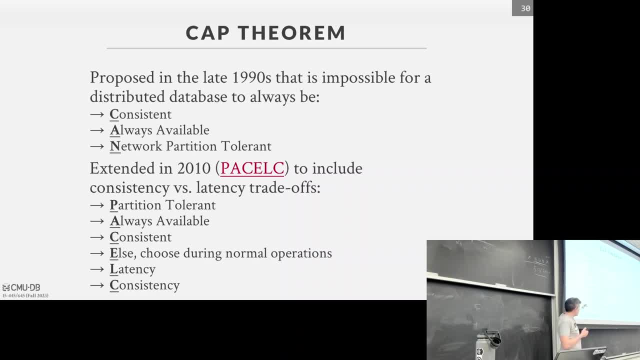 The first part is the CAP theorem: partition tolerant, always available, consistent. But then during normal operations you have this trade-off between your latency tolerance and your consistency tolerance, And we'll see what that looks like in a second right. So let's go through some examples. 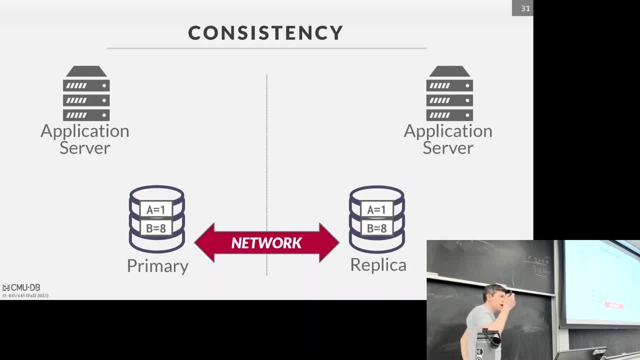 Oops, sorry. So with consistency. the idea is that if I do a commit or a change to a copy of an object in my database and there's replicas, when do I tell the outside world that my change has been propagated, And can anybody see an intermediate? 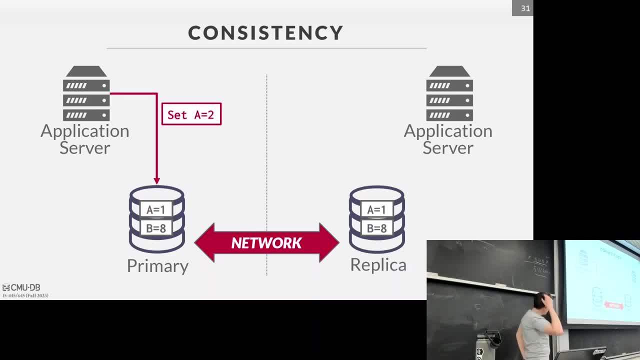 Right, So we talked about this before. between ventricle consistency and trunk consistency: same idea. So if I do an update to A here, this is the primary, this is the replica. I make the change to the primary. I then propagate the update to the replica or, if it's active-active. 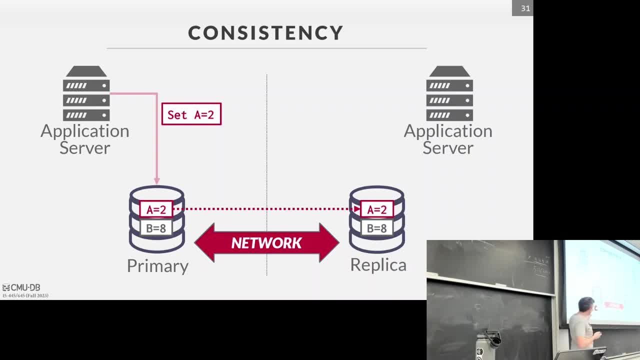 they both run at the same time, it doesn't matter. And then, once I get the acknowledgment from the replica that the change is durable and safe, then I can tell the outside world my transaction is committed. So now, if any other application comes along and does a read on A, they're guaranteed to. 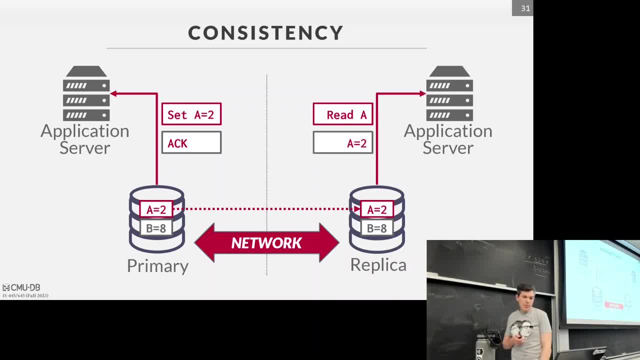 see the update from the committed transaction right. So for single objects, all right, this is doable. You know, really, it starts to matter when you have multiple objects, right? If I update A and B at the same time, can I guarantee that I'll see a consistent view? 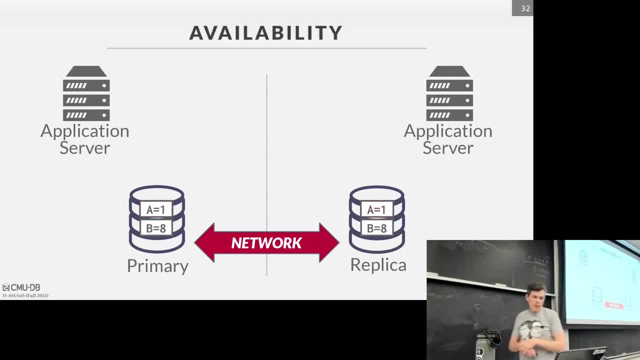 of the database. Availability determines what happens if there's a failure to the overall system. So say this node goes down here for whatever reason. So my application server here They can read the copy on the primary. that's just fine. but what happens if this application? 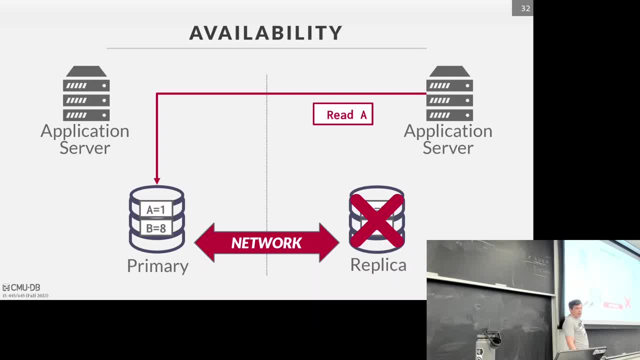 server over there. Well, assuming they can connect to this other replica, then they can still access this content and read the database over there. assuming the network hasn't been severed And no matter how many nodes go down, Partition tolerance says if the network gets severed and now these two nodes can't talk, 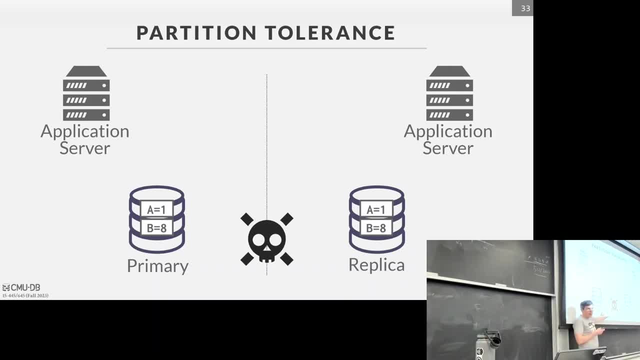 to each other. So what's going to happen here? under Paxos, This guy was the primary right and he's holding the lease on that. and now there's a. it never gets severed, so the replica can't talk to this guy, so he says: oh well, this. 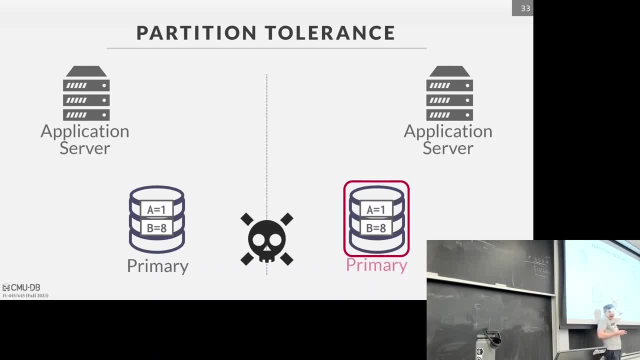 guy's down, so let me run leader election. oh, look at that, I'm now the leader, right, So it becomes the primary. but what's the problem here? So now the first: both applications send updates to A. Both of them think they're the primary and they said, okay, yeah, great, we'll go ahead. 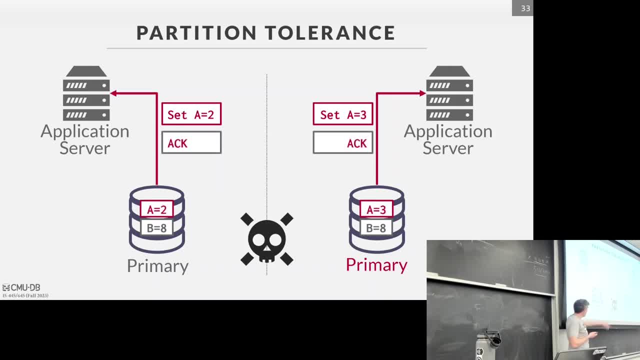 and commit your changes. that's fine, all right, And they get. you get back acknowledgment that those changes got persisted. but then now the network comes back up and now there's a problem where they both think they're the primary and they both think they have the latest version of the object. but who's correct? 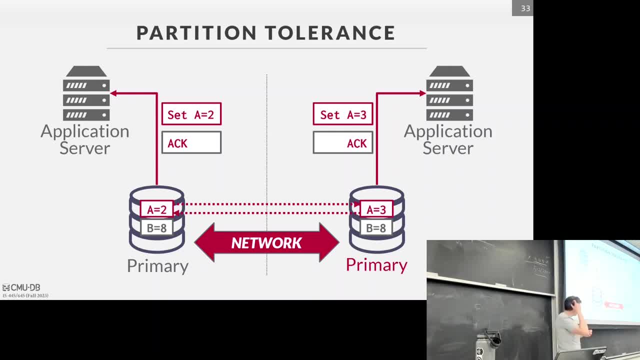 So this is called split brain, right And in most systems, right, Right In most systems. when you have this problem like this goes back to the case. safety thing is: once I don't have enough copies of the of my data, I'm gonna stop the system. 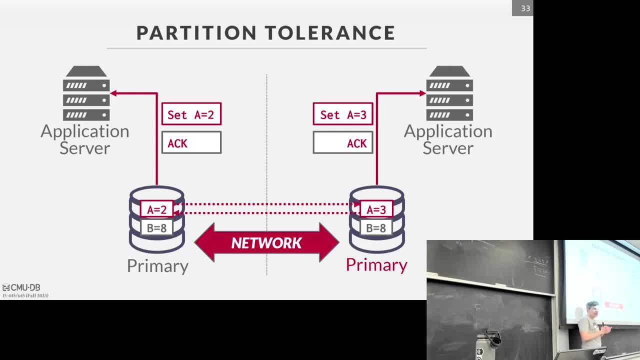 A small number of NoSQL systems back in the day used what are called vector clocks, invented by Leslie Lamport, was basically. it's almost like multiversioning: you're keeping track of the different versions of the object over time. so now, when the network gets connected, 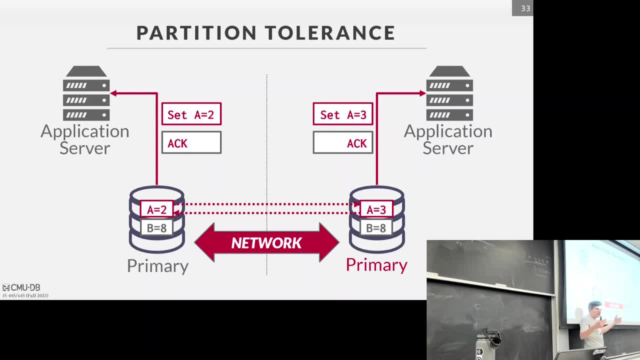 up again. you say, okay, well, you have these changes and I have these changes and I have these changes over this time and you merge the two vector clocks together, but then now you still have a bunch of like different copies of different versions in your database. 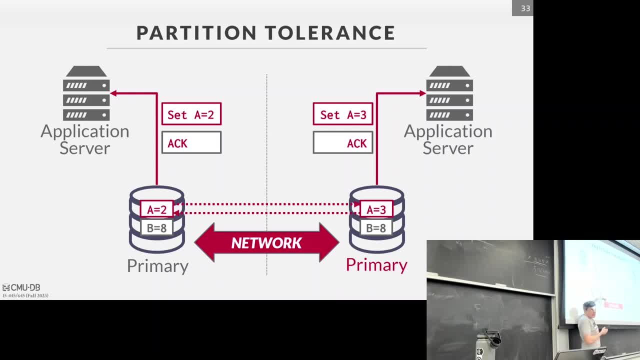 for these objects. so now in your application code you have to write stuff to go reason about what is actually the correct version. So like you as the application programmer, have to write a bunch of up here that, like it's, people always get wrong. it's super hard, right. 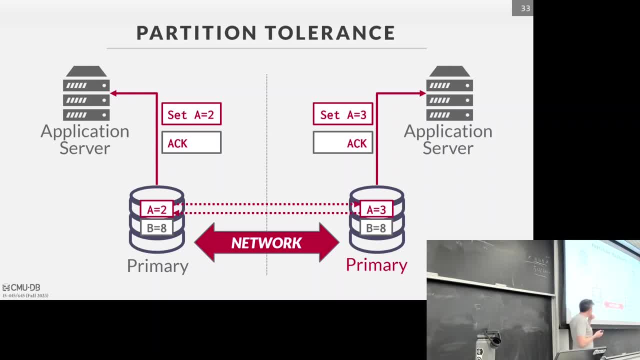 So in the NoSQL world they would. in some cases they would actually still allow this to happen. But then when the network gets you know connected back up again, they'll just pick what everyone has, the latest timestamp, and say that's the latest version. 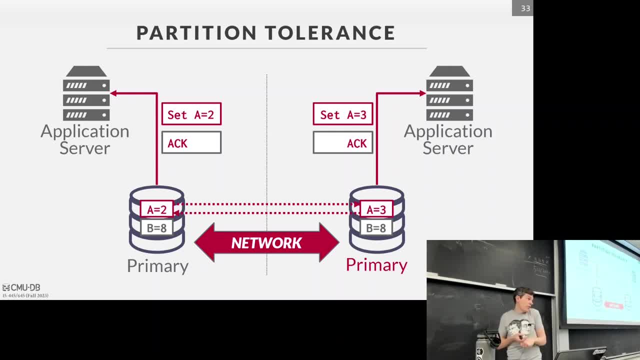 And whether or not that's right or wrong depends on whether the application cares or not, or someone will notice Yes, So why would that be wrong? My bank account has $100.. This guy pulls out $100. This guy pulls out $100.. 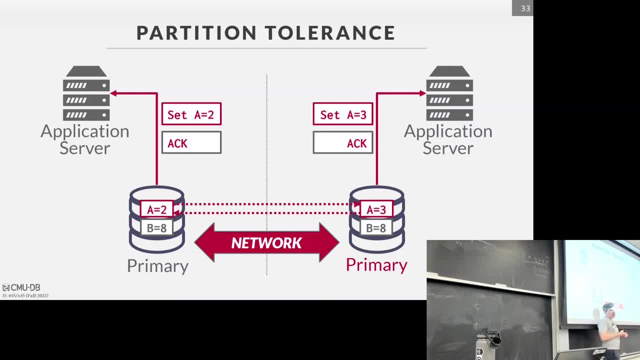 I now come back and now I have negative $100.. That's definitely wrong. What did you do? What did you do? But I've already given out. give out $100 twice. all right, You're happy, Bank's not happy, all right. 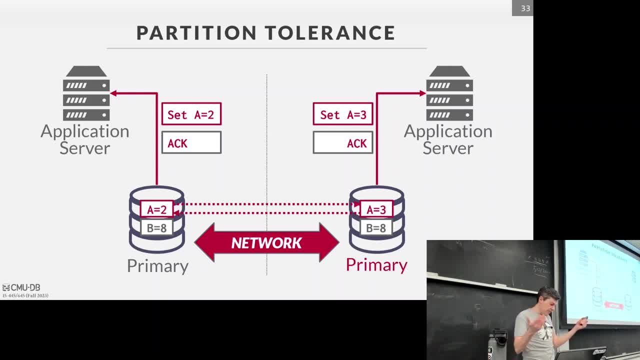 Or think about it: it's the, it's the, the, the, the, the the tuition payment. they take it out twice. You definitely would care, all right, All right. so, and again in the CAP theorem, you kind of see you're going to see you're. 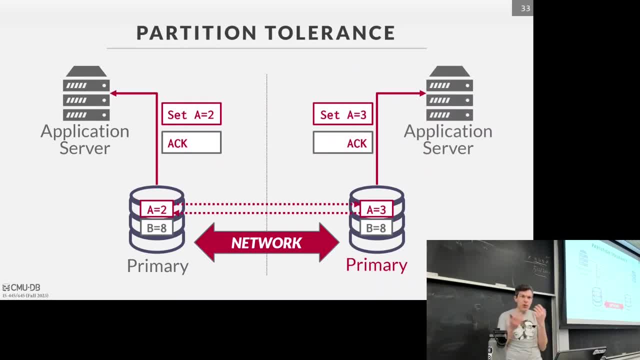 going back here quickly, You can kind of see why, like you can't get all three of those properties right, I can't do, I can't guarantee consistency if I'm going to start doing things like allowing both sides to get updated, because that's not a consistent view of the database, right. 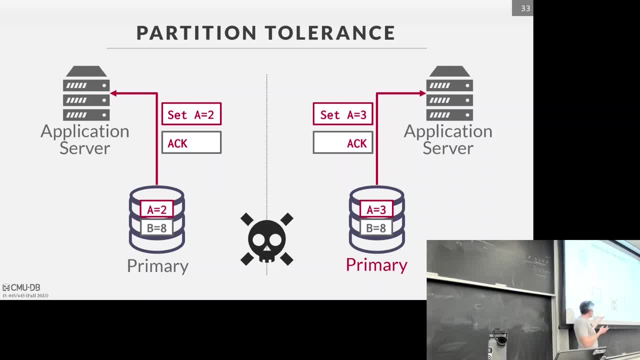 And so what typically will happen is like say: you know, say you have an odd number of of of of replicas. I have three, So in this case here, maybe two's over here and one's over here. 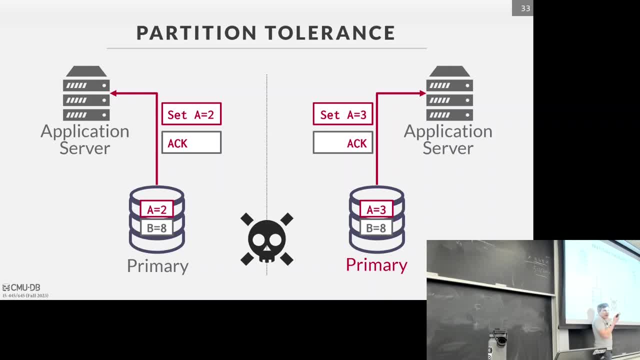 It knew that there was three before, but it says now I don't, I can't do it, I can't get a majority out of, you know, two out of three. So this guy then just says, okay, I'm not available. 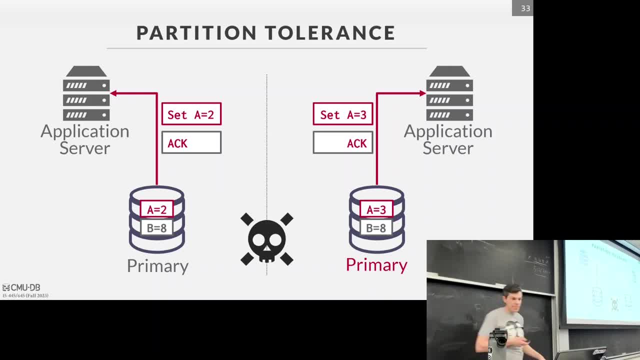 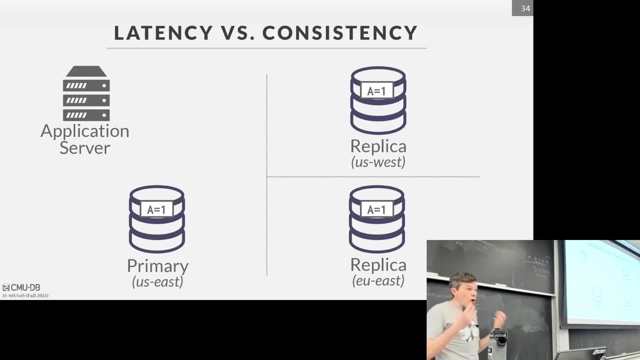 And then this guy, would you know, could run the election just fine. All right, so okay, this is all what happens when there's a failure. But again, under normal operations, even if we have these different properties under the CAP theorem, there's this trade-off between how long we want to wait for changes to get. 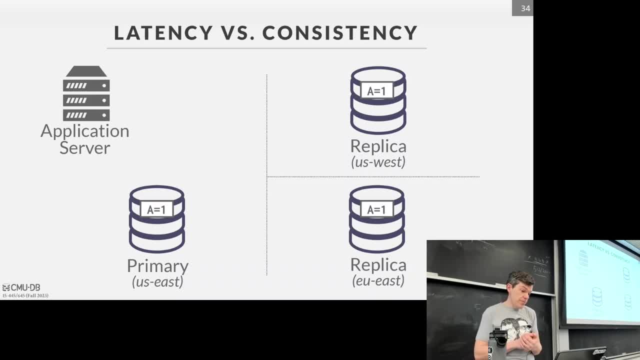 propagated and acknowledged from our replicas Versus guaranteeing that everything's going to be consistent. And so again, so say, my application wants to do an update on A, it's going to set it to two, But then it's going to propagate those changes to the replicas. 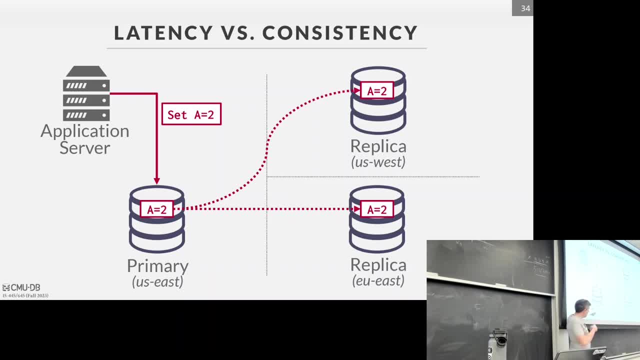 And say: these replicas are in different data centers, like you know. one's going across the country, one's going over the ocean to Europe, And now the question is, how long do we want to wait for the acknowledgements from those other replicas before we tell the application server we, we got those changes? 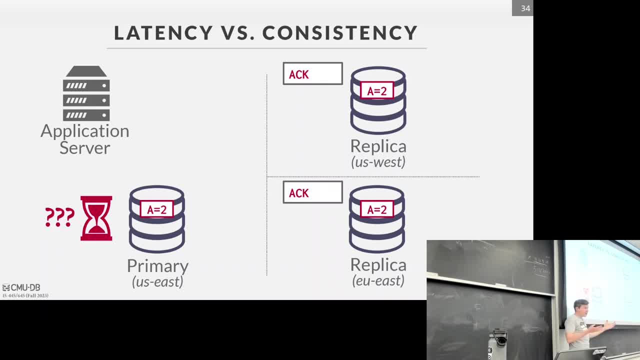 Okay, And again this goes back to that strong consistency versus eventual consistency, and I was saying that somewhere in the middle. So maybe the just waiting for the, the update from, or the, the, the acknowledgement from US West, maybe that's good enough. 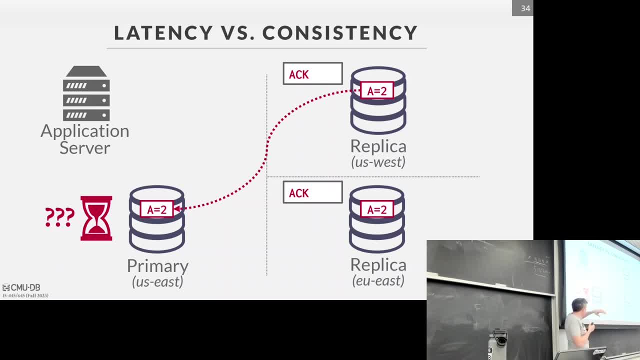 Because now, if I crash and come back, I can, I can, you know, I can make sure that the you know at least pull the change from one of the locations. But depending on like how, how much I really care about my data, which is actually not- 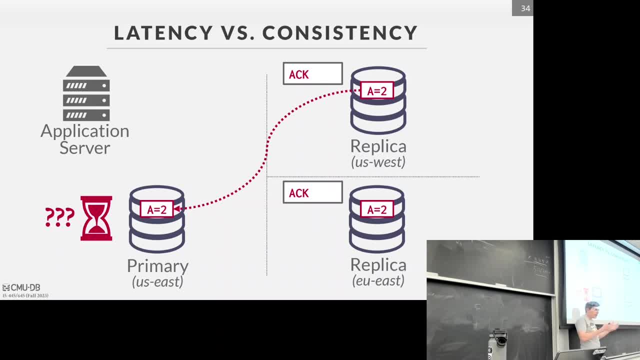 something the data system can, can, can reason about. Okay, Because it depends on the application, It depends on the organization, It depends on whether you're a bank and and like it's financial things, or it's like you know some, some Mastodon website or who cares if you lose some stuff, right? 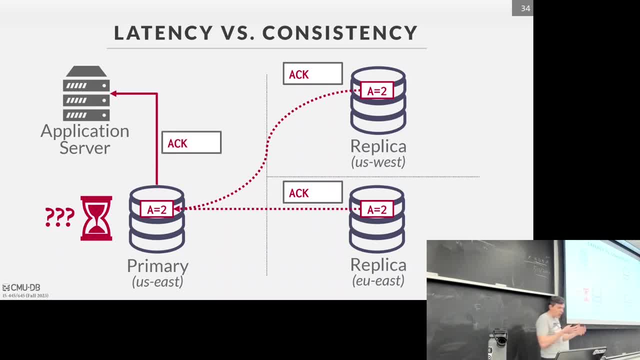 So there's no hard and fast rule to say: okay, this is the right way to do this, no matter what. It really depends for a human to decide what the what the tolerance actually is. But you can clearly see how there's this trade-off between: I can make sure everything's strong. 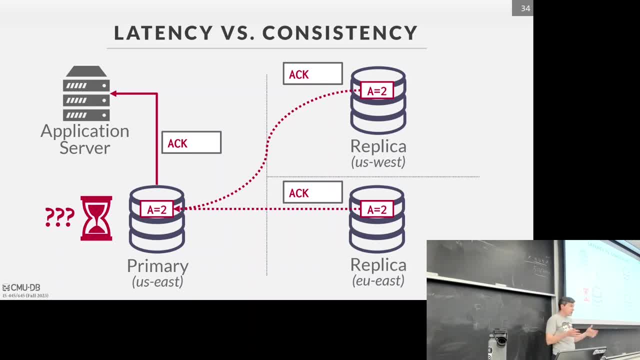 and consistent. but I'm going to wait for that Because there's there's there's the speed of light issues of sending and propagating messages that I can't, You know. there's no magic wand to make that go away. 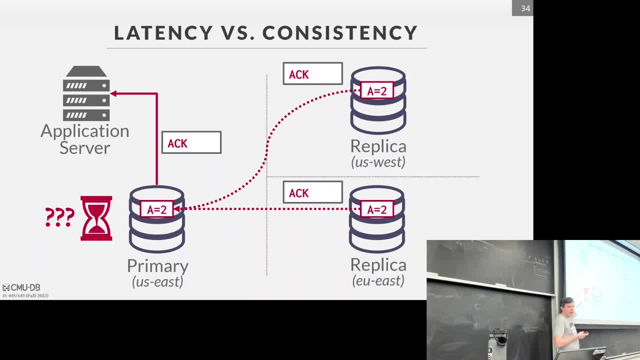 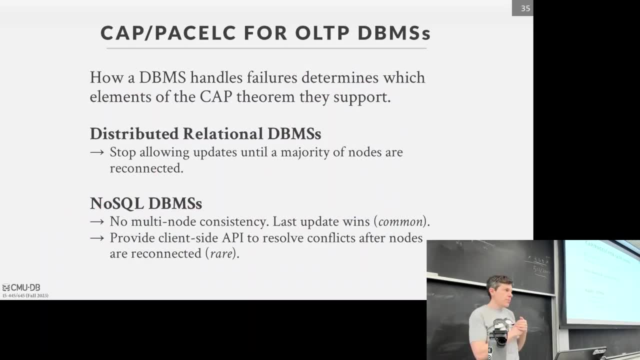 And then if, but, if, but, if I don't wait, then I could have inconsistent data right. So, as I said, most distributed relational database systems, both the traditional ones like the ones from the 1980s, like DB2, and Oracle, RAC and others, they're, they will. they will lean heavily towards strong consistency and overabundance, Over-availability and partition tolerance. meaning if a bunch of nodes go down, they're just going to stop the world until those nodes come back up, because they don't want to have inconsistent data. They don't want to cause you to to to, to have integrity issues, Whereas the NoSQL guys in the original a lot of the original versions they they would not support multi-node consistency because they were trying to support high availability. 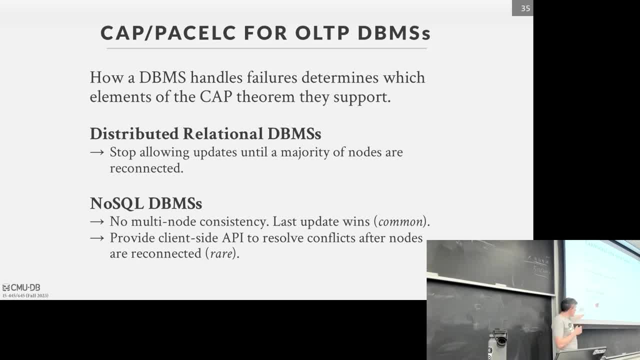 right and be able to scale out, And they would do something really simple like last update, wins, And this last one here. these, these are the vector clocks and, as I said, this is pretty rare. Very few systems do this. 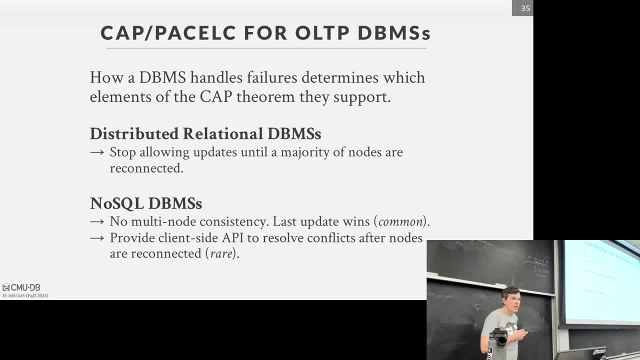 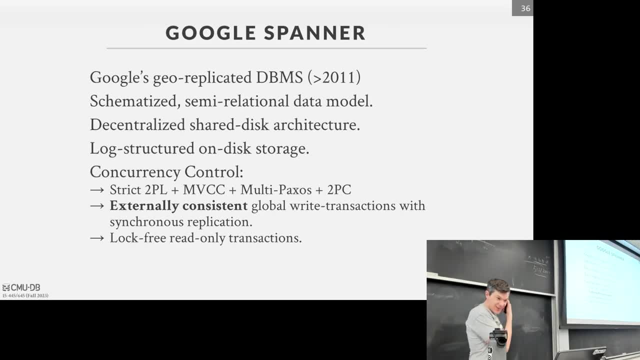 Okay, All right, in the last five minutes let's go through what a very complicated database system that Google split, you know, spent years and years working on, called Spanner. So the background is: Google was one of the biggest proponents of NoSQL systems in the 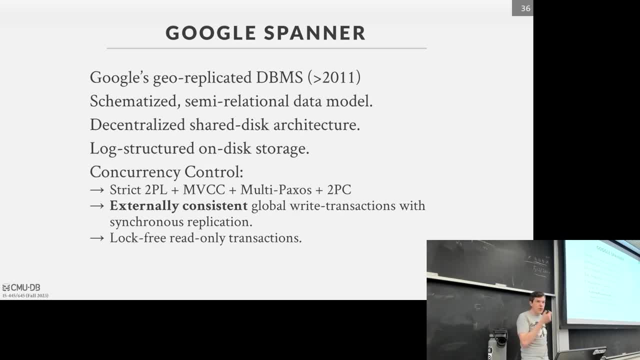 day right, They wrote this paper called called Big Table in 2004,, where they said: transactions: we don't need them, NoSQL: we don't need that. They didn't explicitly call NoSQL, but a bunch of people read those papers and said, oh yeah. 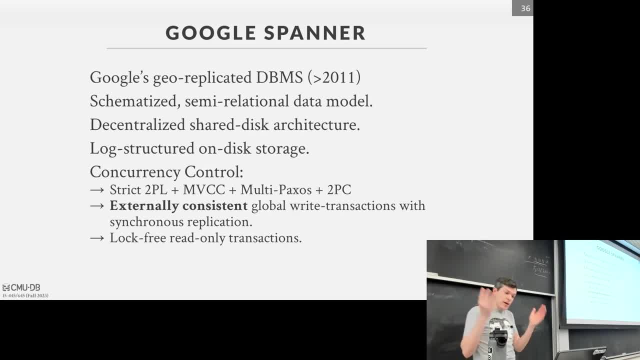 let's build the same things Google's building, because Google's making a lot of money. we want to make a lot of money And it's clearly because of their database. So a lot of people re, re, re-implemented what Google talked about in their papers. 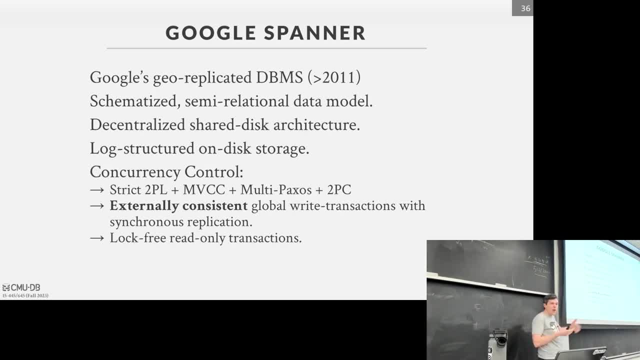 But then so so Big Table came out in 2004,. it didn't have transactions. I think a lot of their stuff had vector clocks where you had to reason about inconsistent data in the application code, But why everyone else in Silicon Valley was re-implementing Google's papers. 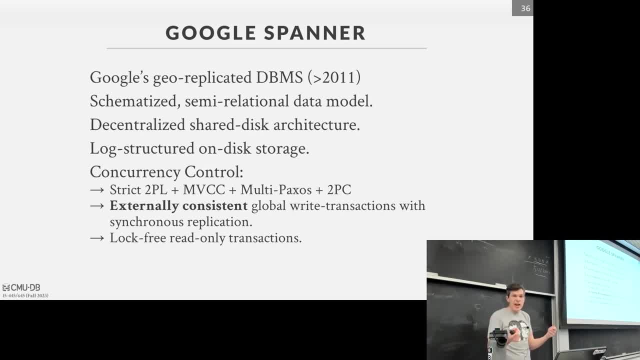 Well, I don't know, I don't know, I don't know why they were re-implementing Google's papers. Google was realizing, hey, wait, SQL transactions are actually a good idea. And they then, over a five year period, when NoSQL was a hot thing, they were building. 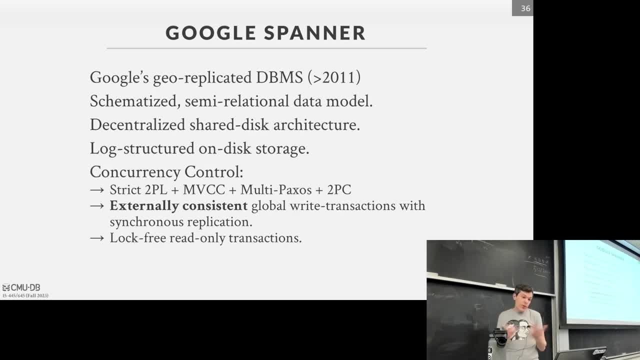 this thing called Spanner. right, And what is? what is Spanner? It's a. at least the original version was not relational database system, It was. it didn't support SQL. They eventually added that. But it's gonna be a, a decentralized shared disk architecture using log structure. on. 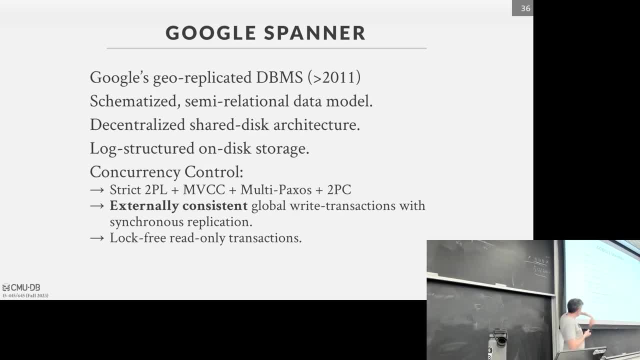 disk storage. And for the concurrency tool, it's gonna hit all our favorite buzzwords. we talked about this this semester: 2PL, multi-version concurrency control, multi-PAXOS and two-phase commit. Now, hopefully at this point in the semester- 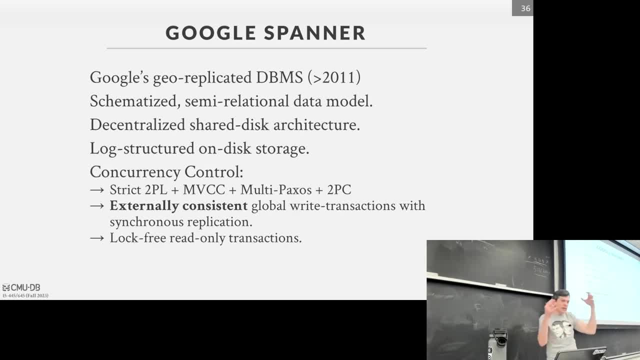 all these words just start clicking and you see: oh yeah, I know what those things are and you see now, when you see them in the context of someone describing a database system, you now can get a big picture of what they're actually doing. 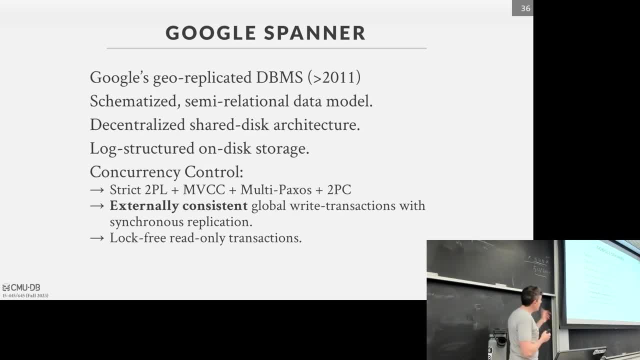 whether it actually makes sense. Now, the one thing Google does- that is very rare, that most people don't do- is that they're going to support what is called external consistency, or strict or strong serializability, Which I think we might have talked about. 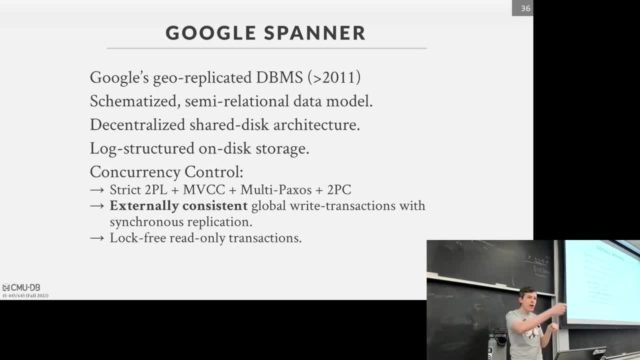 And the basic idea here is that the commit order of transactions is going to be equivalent to the arrival order of transactions, which is not something we talked about when we talked about serializability. on a single node, We said: oh yeah, this transaction. 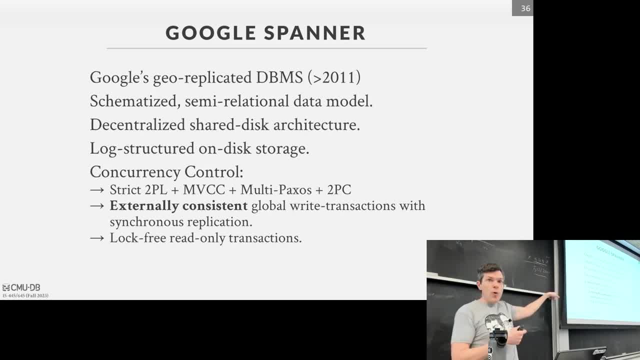 could arrive after this one but could still commit for the other one. In their world they need to guarantee that transactions arrive or get committed in the same order that they arrive. They claim in the papers: because of something about ads, They built Spanner. 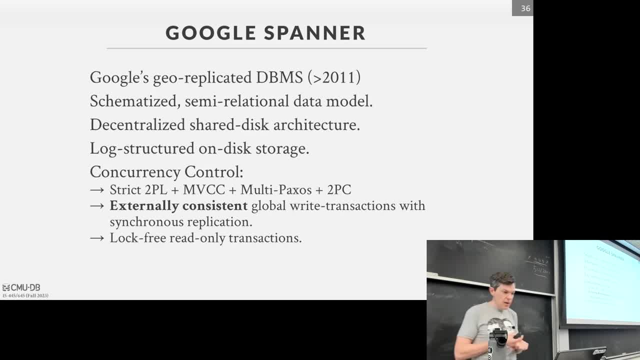 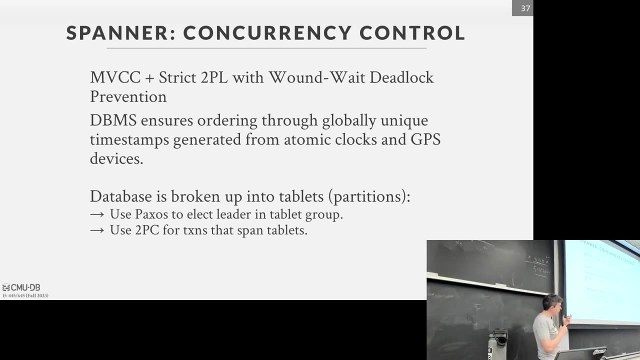 Spanner for running their behemoth ad infrastructure. Very few people need this And very few systems actually support this. We can ignore lock-free transactions for now, So the way it's going to work is that they're going to guarantee the ordering of transactions. 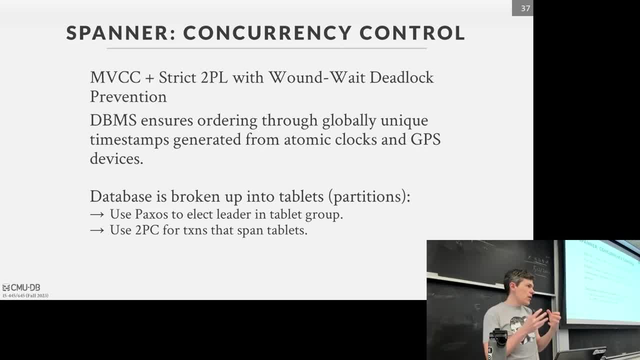 through globally unique timestamps that are going to be generated through a combination of atomic clocks and GPS receivers in every data center. So they're going to have some satellite dish on top of every data center. They're going to have some satellite dish on top of every data center. They're going to have some satellite dish on top of every single data center to pull down the timestamps coming out of the GPS satellites. Now it's not going to guarantee that timestamps are going to. It's not going to guarantee that it knows the exact ordering. 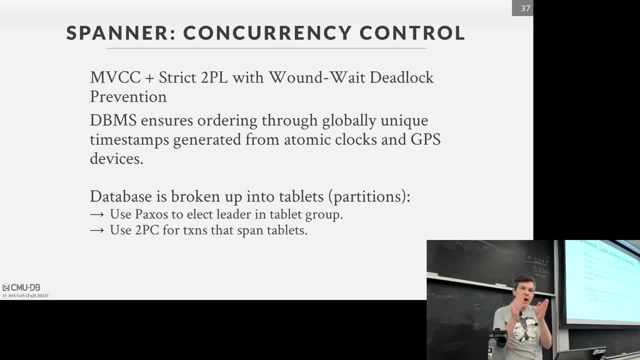 at any given time for any transaction, but it's going to allow us to bound how long we have to wait before we expect a transaction to show up with a lower timestamp than our transaction when we have to commit. And that's the novel aspect about this. 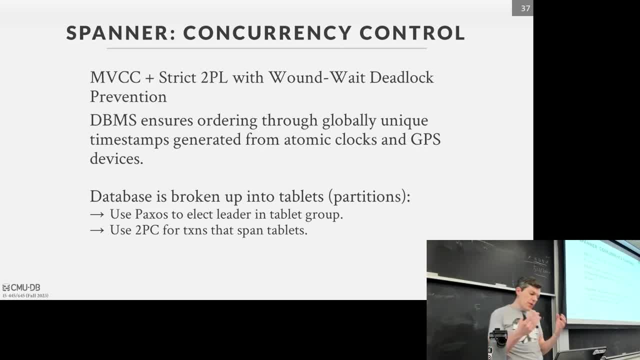 because otherwise, you know, if you want to do this global ordering across different data centers across the wide area network, you're going to have to wait. but because the clocks could be skewed slightly off from one data center to another, you might have to wait a little bit longer. 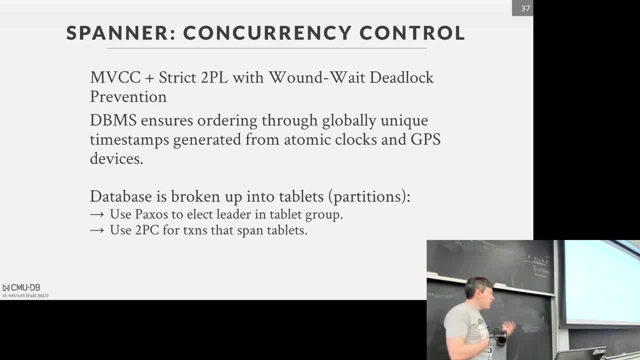 than you would otherwise if you had this. And as far as I know, I don't know of any other people, I don't know of any other company that publicly talks about having this kind of infrastructure. The high-frequency trading guys might, but they don't write papers. 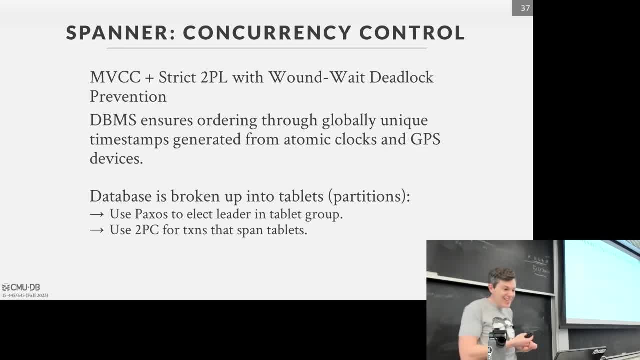 and they don't share what they're doing because they're too busy counting their money. But, fun fact, when I was in grad school, one of my early years, I was sponsored by The research funding was sponsored by this company out of Chicago. 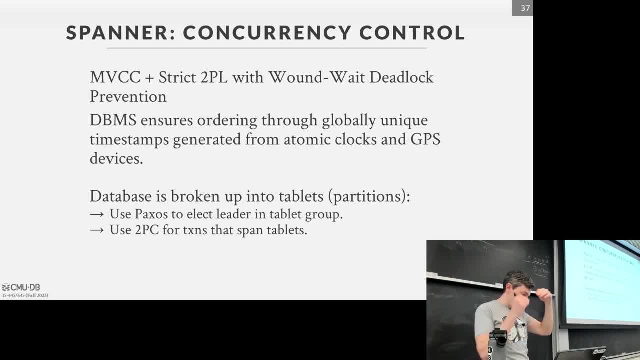 who their claim to fame was in the 90s. they figured out if you put the database server on the floor above the stock exchange, you make money faster. They obviously did a lot more stuff since then, but the things that they were telling me. 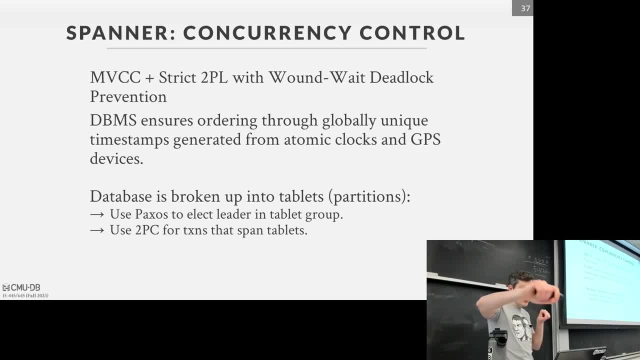 they would do was insane. We're talking about digging trenches to run their own fiber optic cables, because it'll get them like five milliseconds less, because, again, in their world that matters a lot. So all right, All right, so the way. 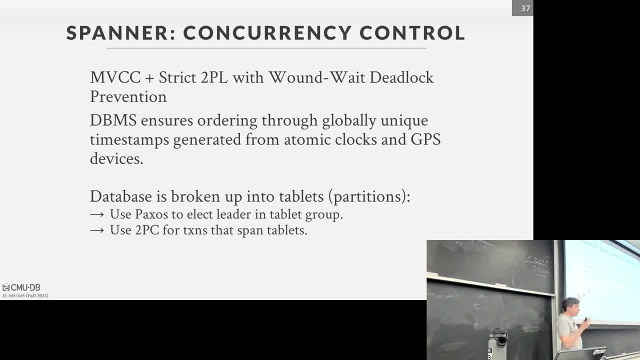 Spanner's going to do it. it's going to break the database up into what they call tablets. These are just partitions And they're going to use Paxos to do leader election in a tablet group. But then, if I have to update data, 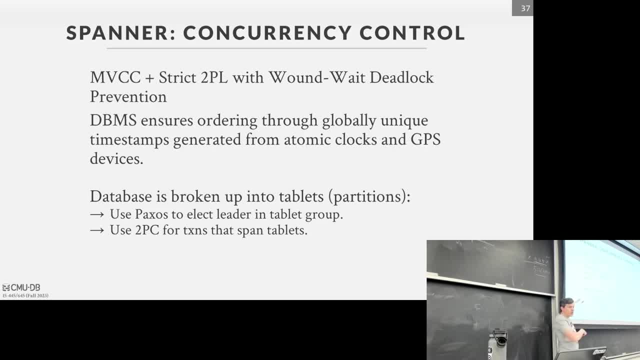 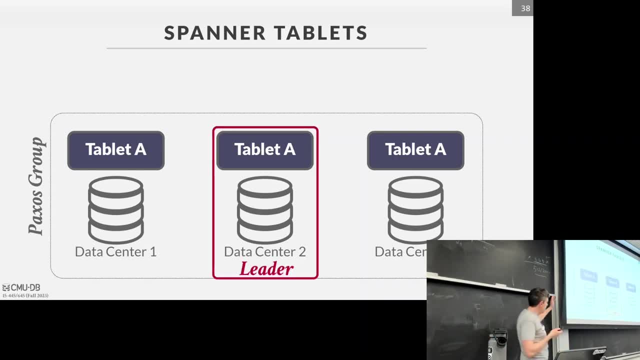 across multiple tablets, then I'll just use regular two-phase commit for this. So visually it looks like this: You elect a leader within my data center. All right, so there's the tablet. All right, so there's the tablet. 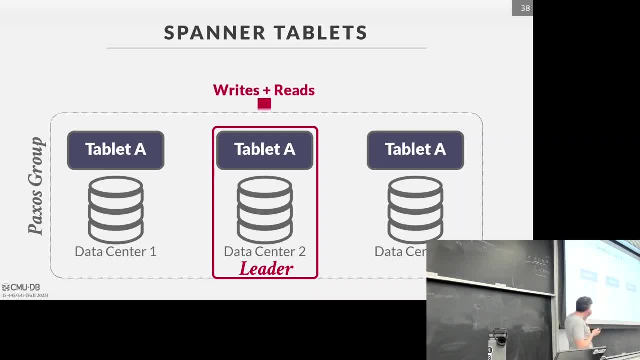 And it's replicated across different data centers. There's some data center that's a leader. All reads and writes have to go to this guy And then use Paxos to propagate them to everyone else And then any snapshot reads which again. 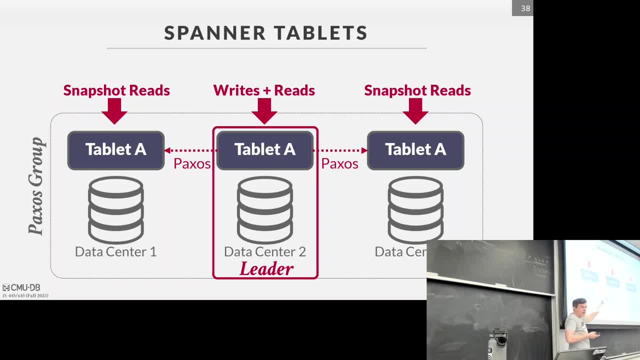 think of like a consistent snapshot on time. I can then run on the non-leader tablets to read any data that they have. But if I have a transaction that has to update another tablet group, whether or not it's in my same data center or not, 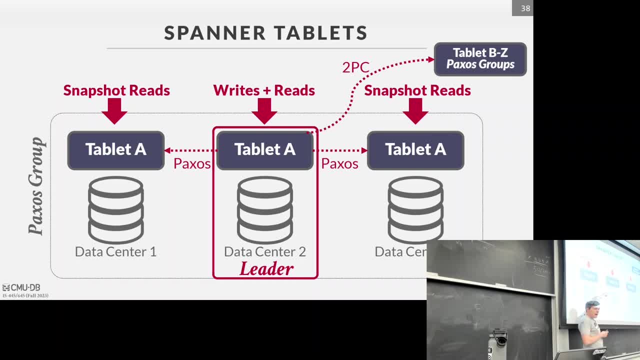 in their world. they're replicating across multiple data centers. I'm going to use two-phase commit to then replicate and do updates that get propagated to those other tablets, which then go to their leader, who then propagates those changes using Paxos. 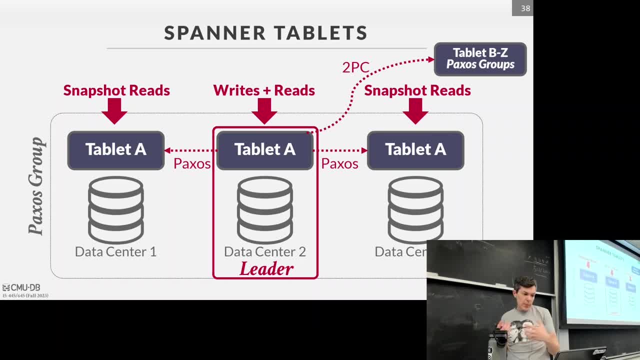 So this is a good example where the things aren't mutually exclusive. like Paxos and two-phase commit, You can use a combination of both of them. Most systems just do one or the other. All right, I'm going to skip this slide. 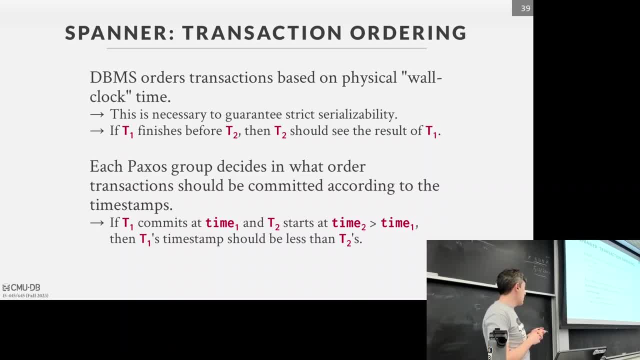 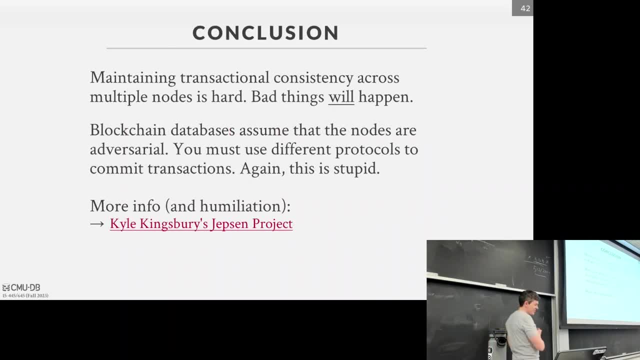 This basically says how they guarantee strict serializability and do time sampling. So all right. so there you go: Three minutes to cover Paxos or, sorry, to cover Spanner. If you guys want to learn more about it, we can again vote for it. 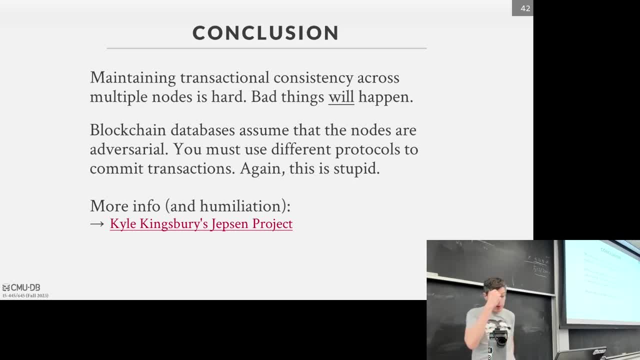 We can cover it on the speed run at the end of the semester next week, All right, so the main takeaway for this would be that maintaining consistent view of the database across multiple nodes is hard, And it's important that you get this right, because there will be failures. 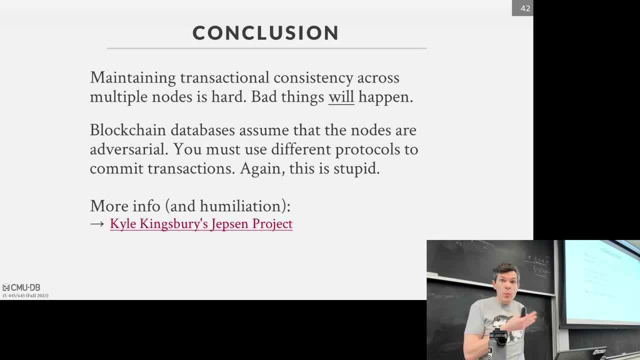 Not just the machine goes down, but weird things that are outside of your control: the purview of the data, some like GC pauses or network hiccups, that again. so you have to prepare for all these things And, as I said, 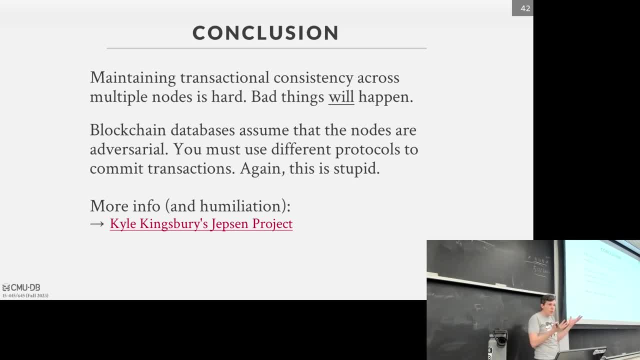 blockchains are a waste of time because most applications don't run. in this world. Bitcoin is the only really useful thing you can use a blockchain for. Most you know most people running transactions are going to trust people to you know are going to trust the machines. 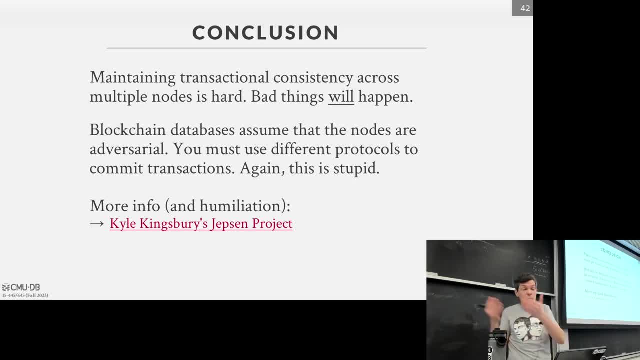 and are going to trust the authority. because this is sort of how the real world works: If you buy something, you give them your credit card number and you trust them to go charge your credit card number. All of those are going to be trusted transactions. 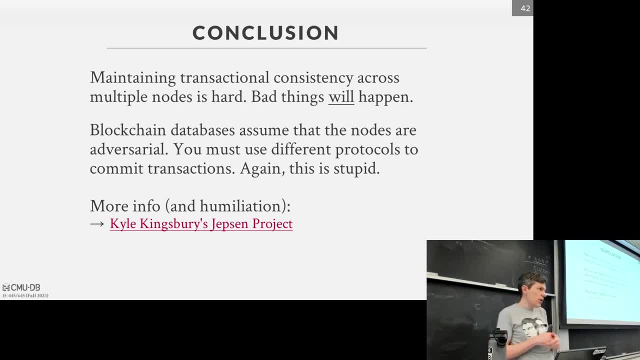 And so you don't need blockchains. So the overhead of gaining visit team fault tolerance is unnecessary. So if this stuff is super interesting to you, there's a great blog article or blog from this guy, Kyle Kingsbury. He has this thing. 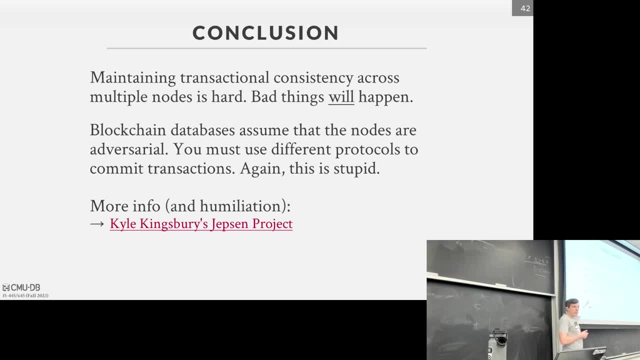 called the Jepson Project. Ten years ago at Stripe he basically wrote a torture chamber for distributed databases to prove that they don't make all the. they don't achieve all the guarantees that they're claiming. They don't, you know. 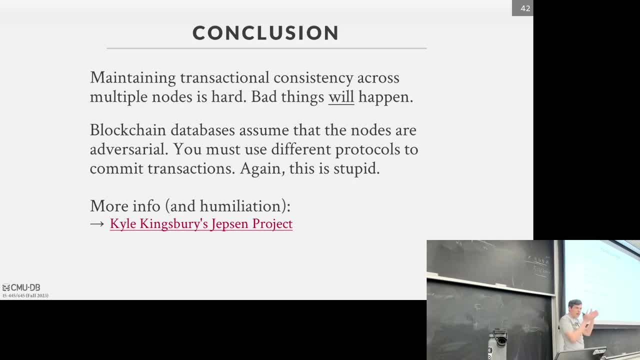 they're not strong in the ecosystem and they can't handle this kind of failure, Like think of the context of the cap, like are they truly partition tolerant, or so forth. And so his blog articles are fascinating. They're very, very detailed and they go into 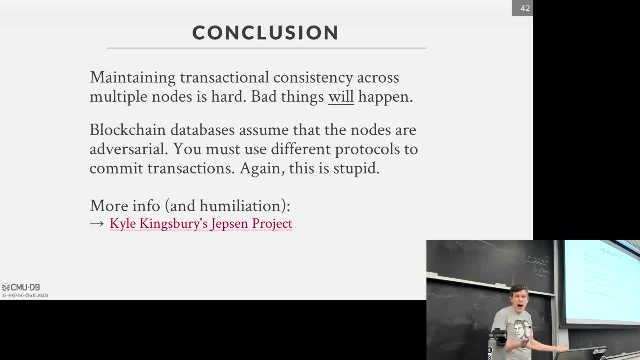 all the failures that occur. He was really just doing this as a hobby, but then now he spun it off as a consultancy company. So a bunch of the distributed database companies hire him to then run his torture chest, torture chamber on their databases. and then he writes: 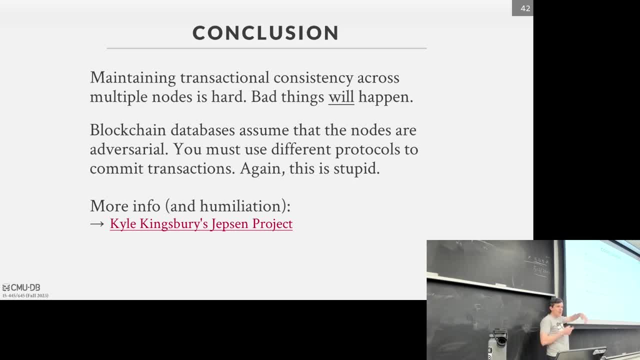 about all the failures. What's awesome is that he- a bunch of companies claim that he could do this feature or that feature. He comes in and destroys them and they have to change their marketing language to to reflect that like: oh yeah. 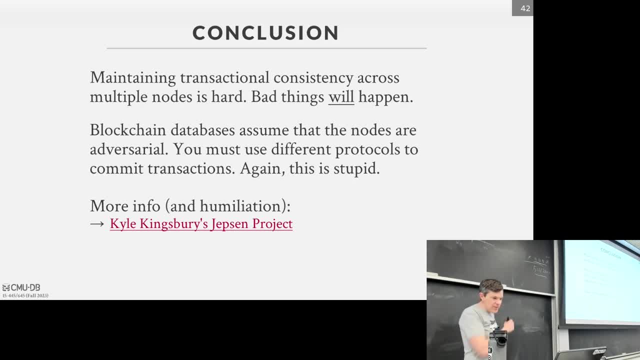 we're not actually this until they eventually actually fix it. So again, this stuff is. don't read his blog article, You'll see why. Okay Next week or sorry next Wednesday. OLAP systems- We won't worry about transactions. 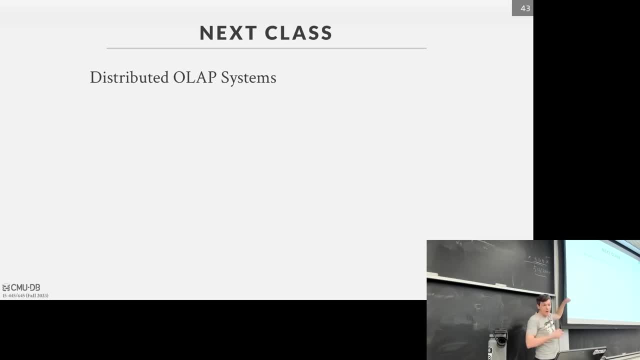 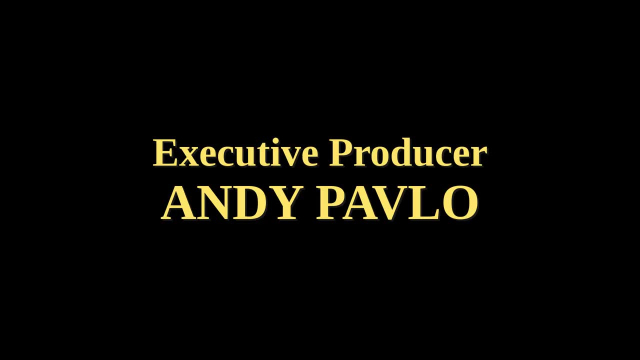 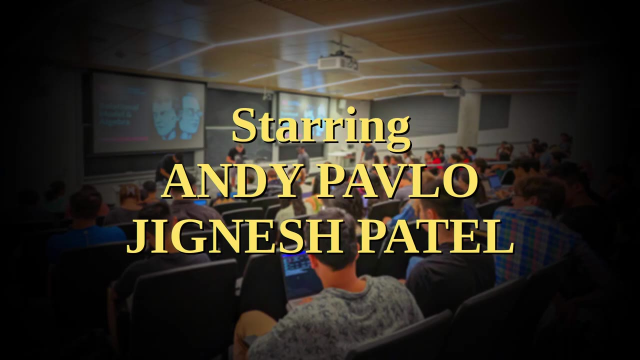 but the big problem we're going to face now is how do we do joins in a distributed environment? Okay, I wouldn't normally say, hit it if he's not here because he's sick. The shit is gangster, Gangster, That boy's a gangster. 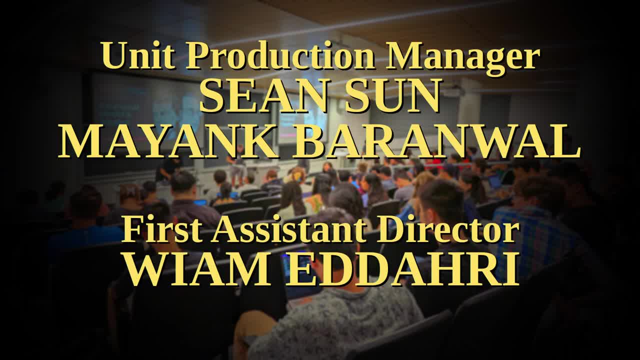 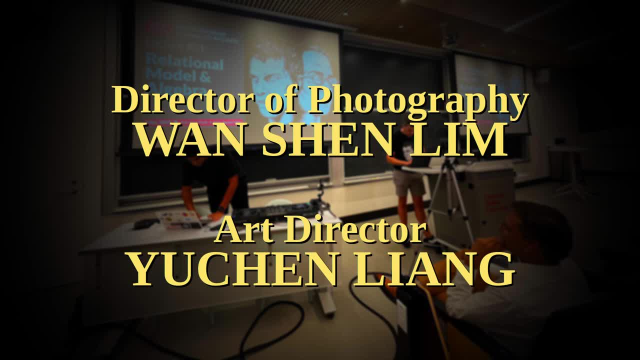 You ain't nothing but a gangster, Yo yo. Now listen, I'm the papi with the motherfucking hookup: 28 a gram, depending on if it's cookup. You ain't hit a mob yet, Still got you shook up. 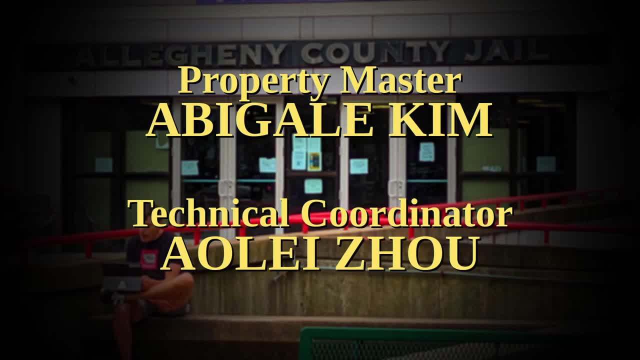 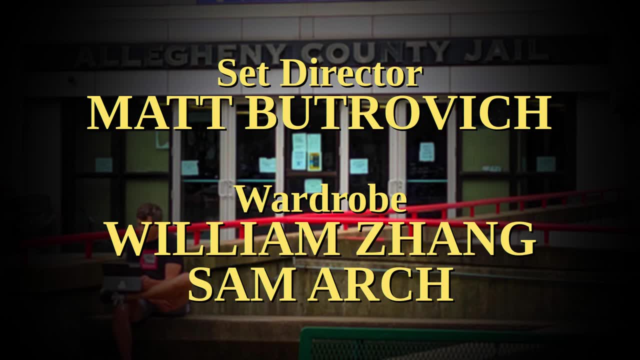 I smack you with the bottom of the clip until you look up. Show me where the safe's at before I blow your face back. I got a block on taps. The feds can't trace that. Style is like tamper proof. You can't lace that to Dominican. 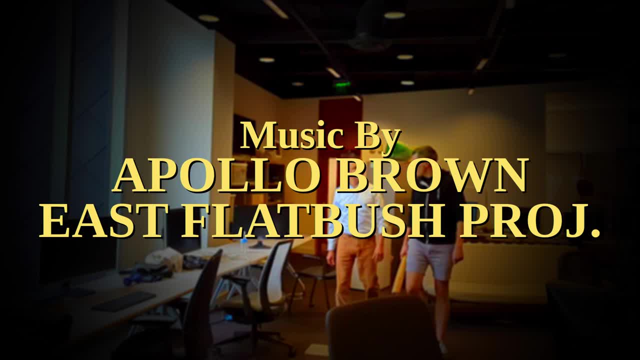 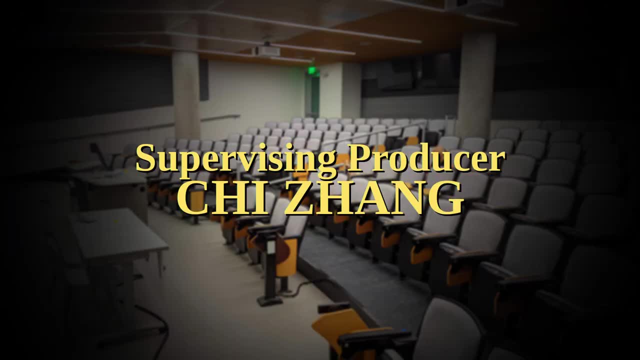 Or you could call me Dominican Black, skelly black, leather black, suede Timberlands, my all black dirty haters, Send you to the pearly gates. You get Kusama trying to skate And that's your first mistake. I ain't lying for that cake. 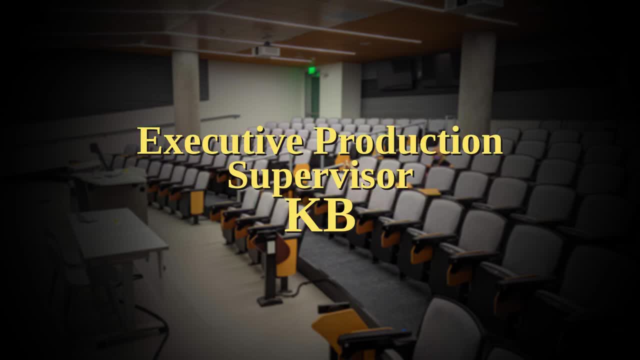 Your fam will see you wake. My grams is heavyweight And ran through every stake. When they ask me how I'm living, I tell them: I'm living great.